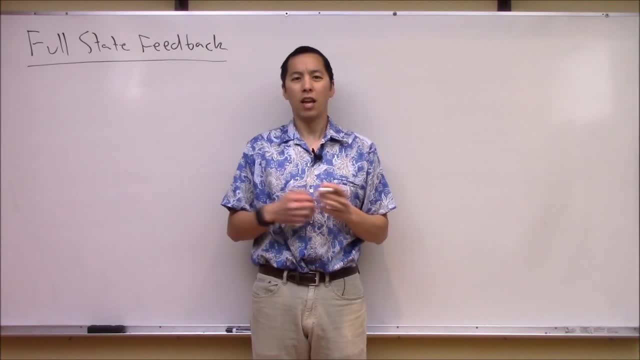 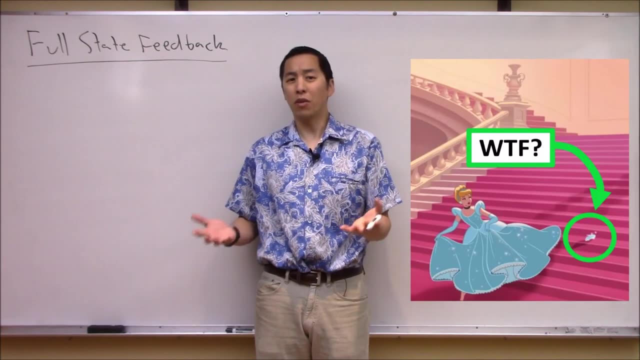 simple or powerful, not both at the same time. It almost seems like a paradox, Like: if Cinderella's slipper fits so perfectly, how did it fall off in the first place? Well, in this case, if this controller is so simple, how is it able to be so powerful? Well, that's exactly what I'd. 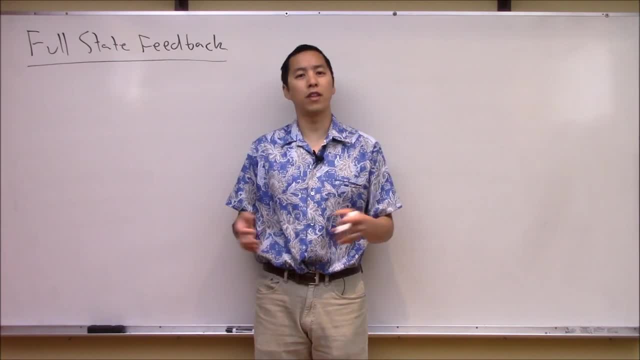 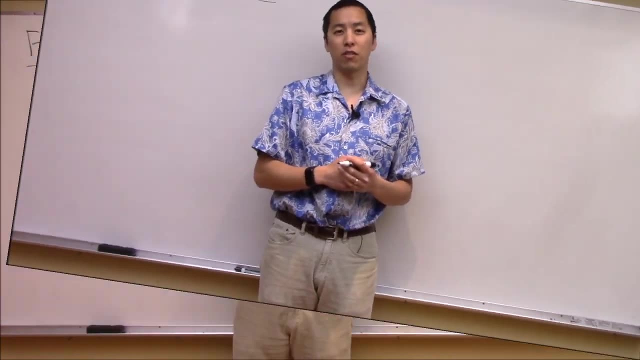 like to investigate today. So if all this sounds like more fun than a box full of GI Joes- and I guarantee you we'll actually play with a bunch of GI Joes before the video is over- then let's jump over to the whiteboard and get started. All right, so let's start with. 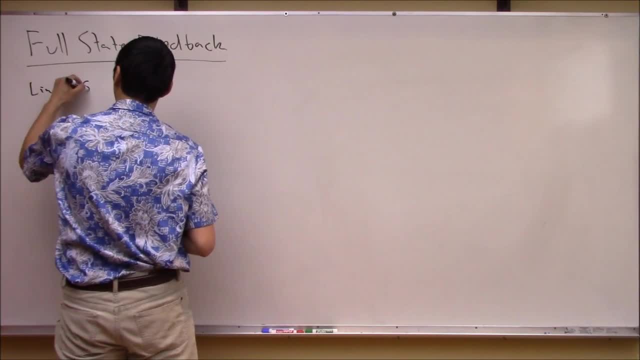 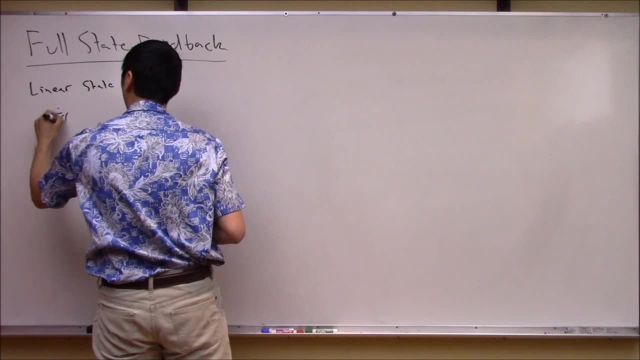 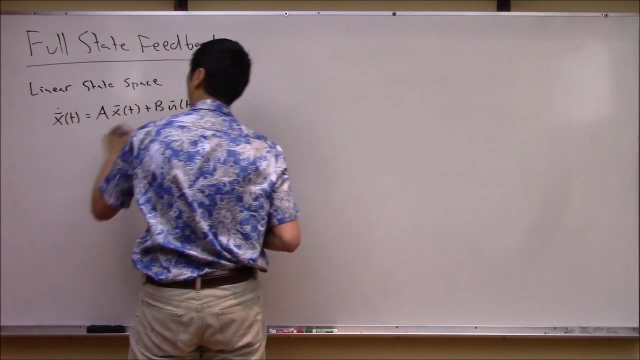 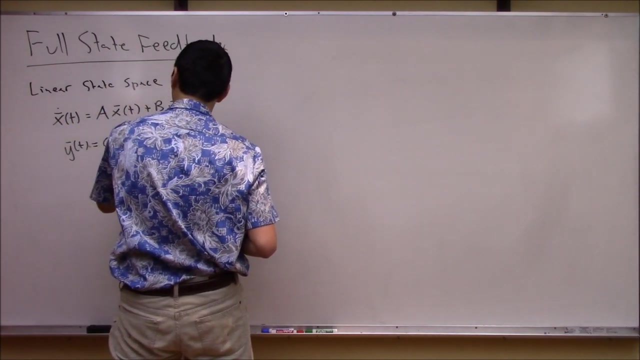 our good old friend, the linear state space representation of a system. Okay, so, if you remember, that's just saying that we've got our model of the system, as x dot is equal to ax plus bu and in this case, y is equal to cx plus du. Okay, all right, so graphically, 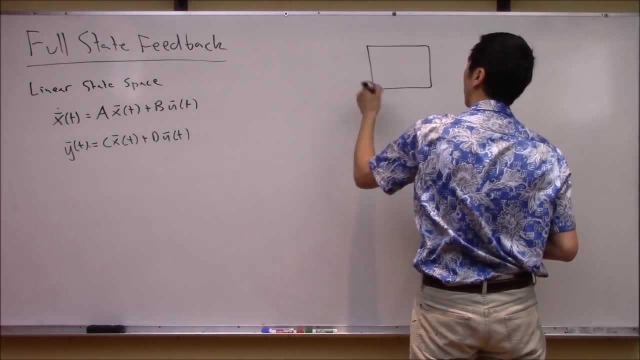 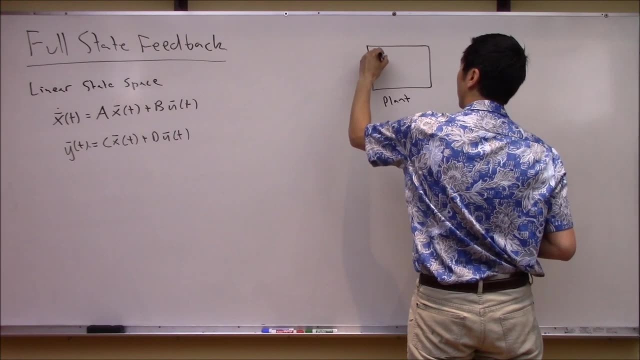 again, if we want to look at this as a block diagram, you've got your system here. So this is your plant, So it's got our state space representation here Of x dot is equal to ax plus bu. And now let's deal actually with this output here. So what I 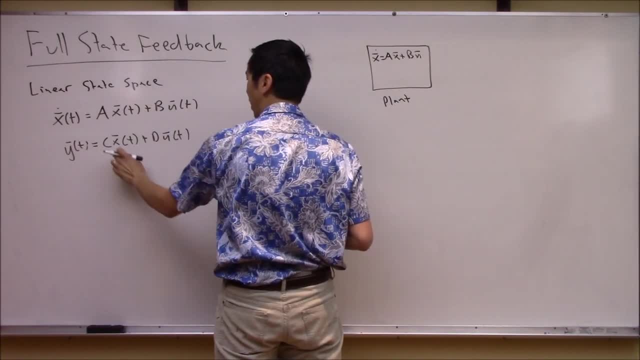 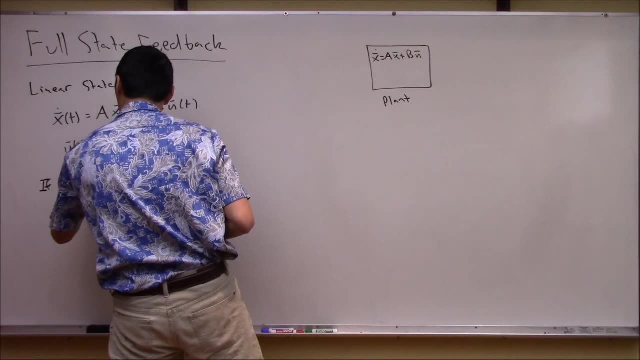 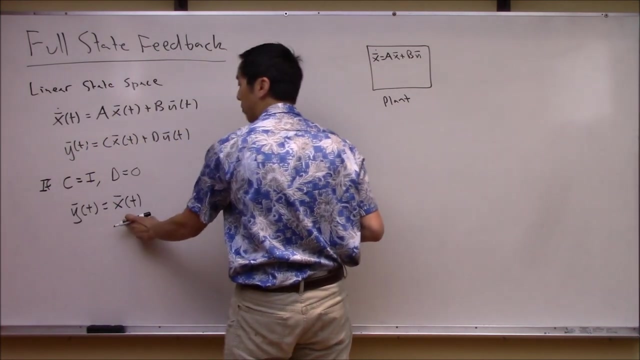 would like to consider now is what would happen if c was the identity matrix and d was zero. So if c was the identity matrix and d is a big fat zero matrix, what we're basically saying here is that the output of the system is the entire state of the system, right? So that's one of the 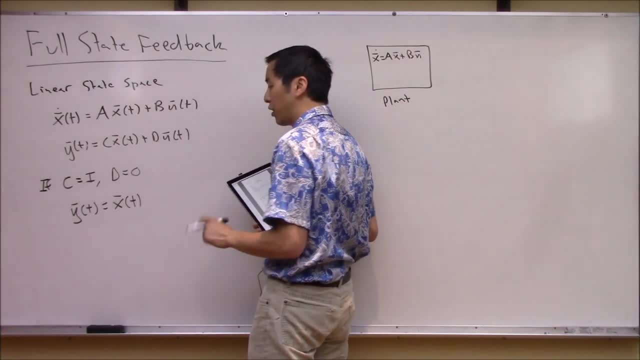 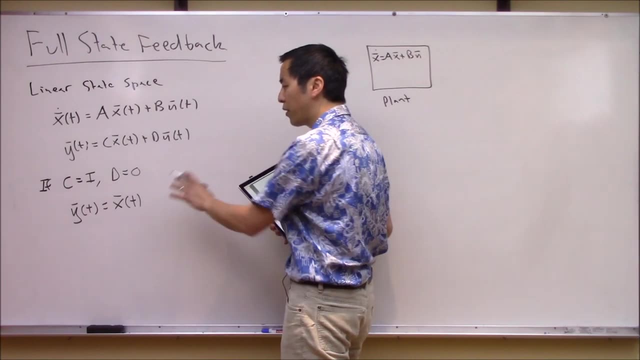 assumptions we're going to have to make for this full state feedback discussion here. We're going to see later on that that might come back to. I don't want to say to come back to bite us here, but it is a a bit of a restriction. But for now let's make this assumption. 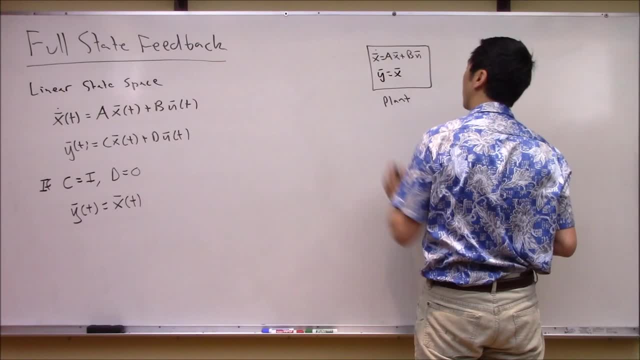 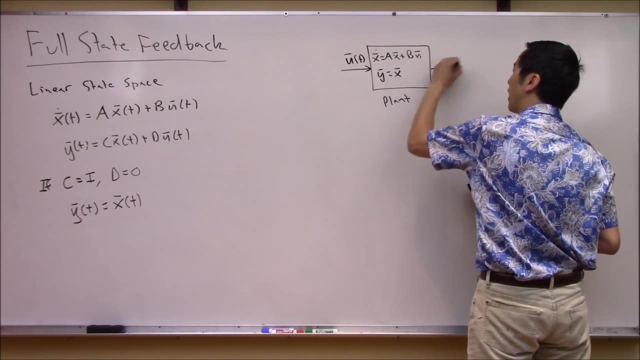 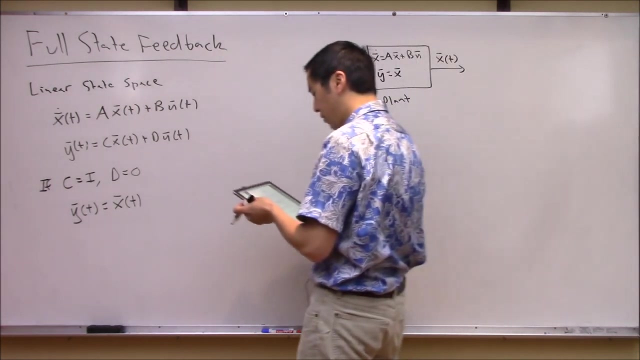 here. So in this case we have, y is equal to x, right, So coming into the system is obviously u, but coming out is the entire state vector. Okay, so if we have this system, the control law that we would like to consider is a very simple. 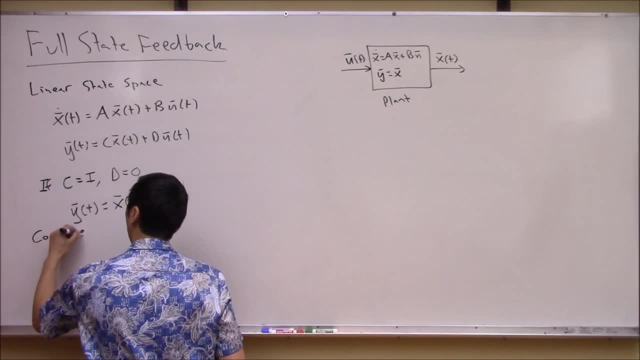 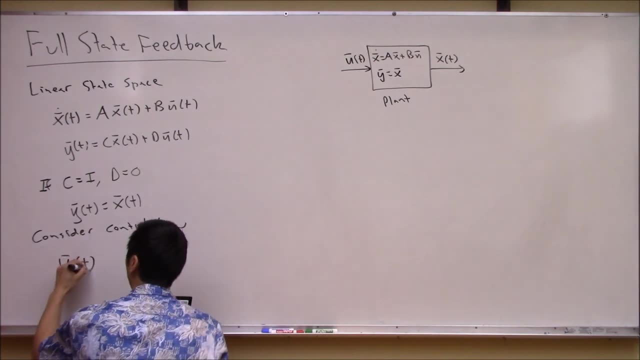 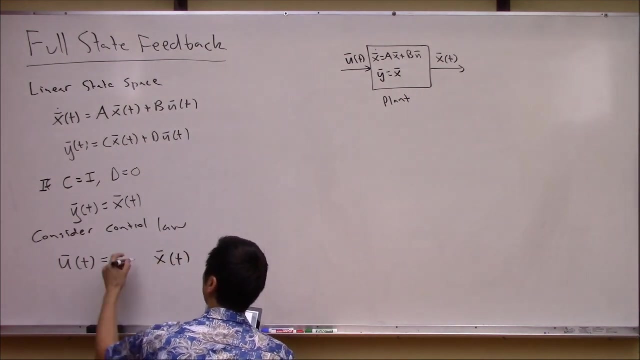 very simple method for full state feedback. So let's consider a control law that is very, very simple, And this is where the simplicity comes in. So we're going to say that the control law here is that the input to the system is just the state vector, but it is going to be scaled by. 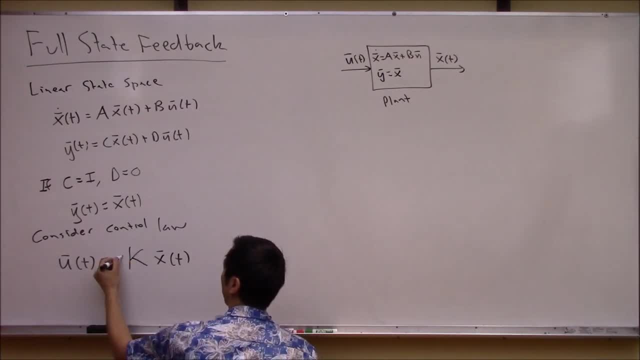 some matrix k And typically by convention, we're also going to put a minus sign in front of it. The minus sign. it could be consumed into the k sometimes, depending on who you're talking to, but most places we'll see this as a control law. u is equal to minus kx. okay, So let's box this up. 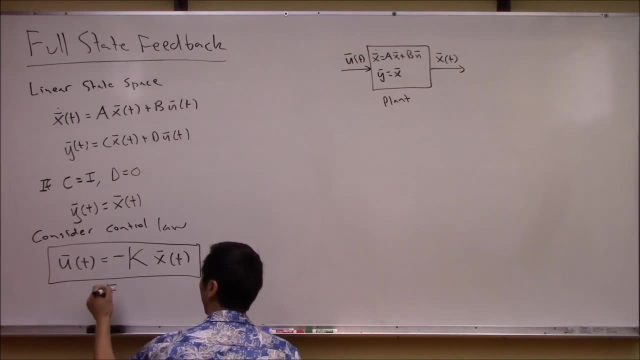 because this is actually the control law for full state feedback And I don't want to have to keep writing a full state feedback, so let's call this fsfb, okay. So full state feedback is basically saying the control, it's just the states scaled by a matrix here. So if I wanted to draw this up, 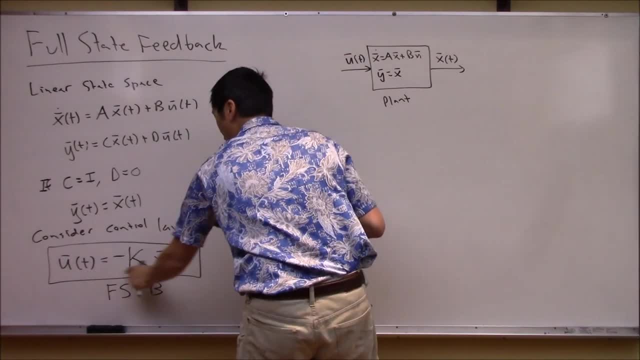 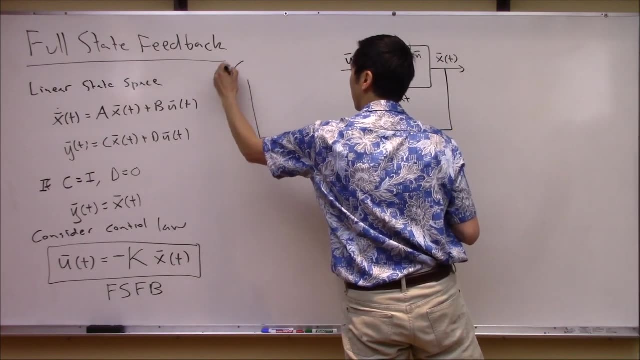 in my block diagram, we got to see that the only thing you have to do is make u equal to the state vector, And I just need it to come back through. and I'm going to put a little block here just for fun, and 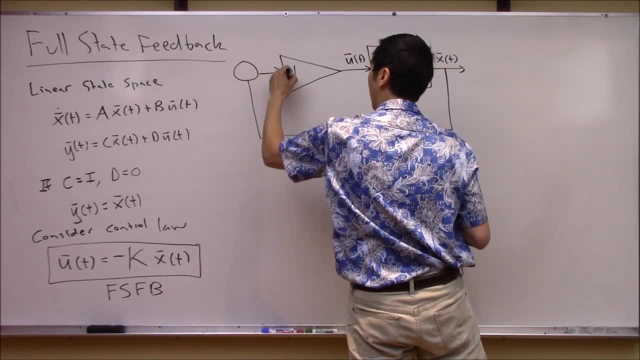 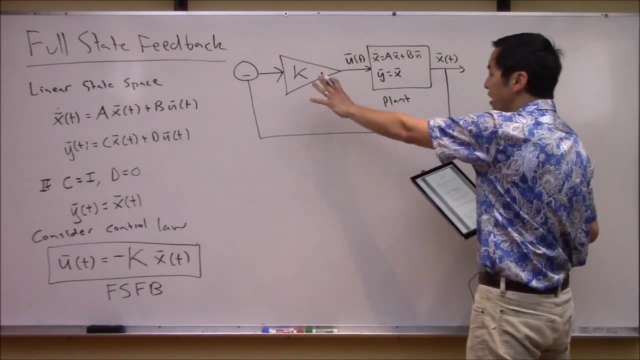 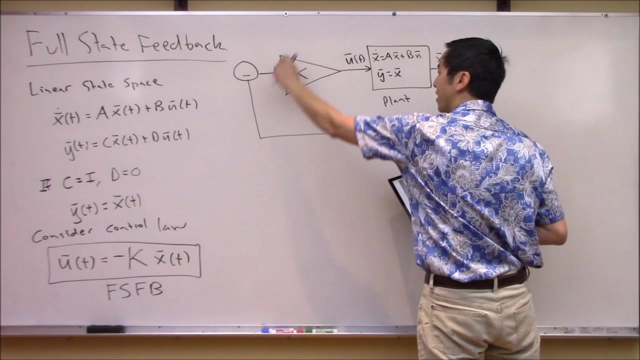 we'll see why in just a second. This goes through a matrix, k, okay. And then to pick up the negative sign here, maybe I'll just draw it like such, okay, So you can see clearly that in this diagram u is equal to negative kx. right, So this k here can be thought of as your full state feedback. 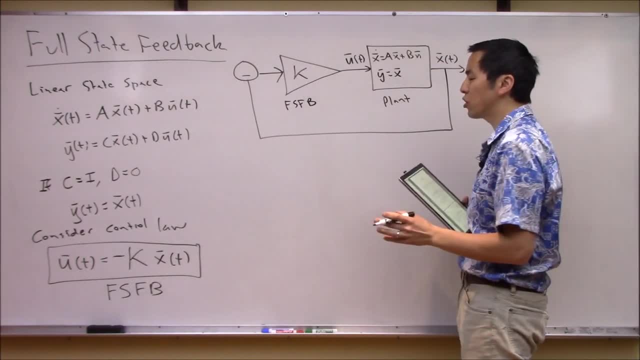 and I don't want to call it a control law, but I'm going to call this fsfb and I'm going to call it a controller really, because if you look at this picture here, maybe a better name for this would be. 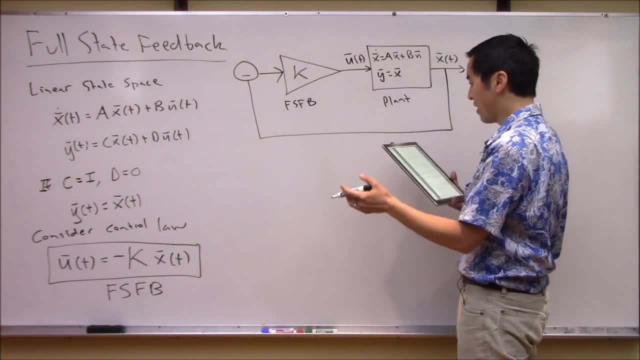 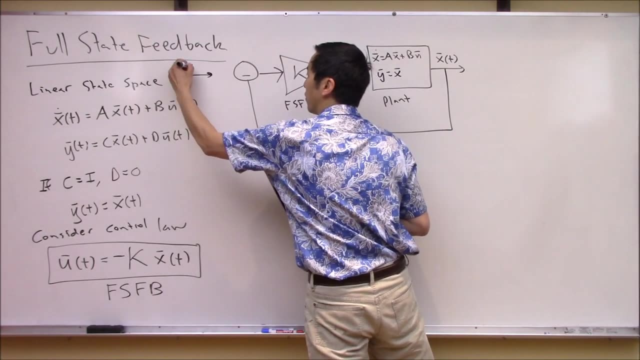 regulator, because what this thing does is that it's going to try to regulate the states to zero. There's no input signal, there's no reference signal, there's no r of t coming in anywhere in this picture. right Later on down the road maybe we'll incorporate that, but for now 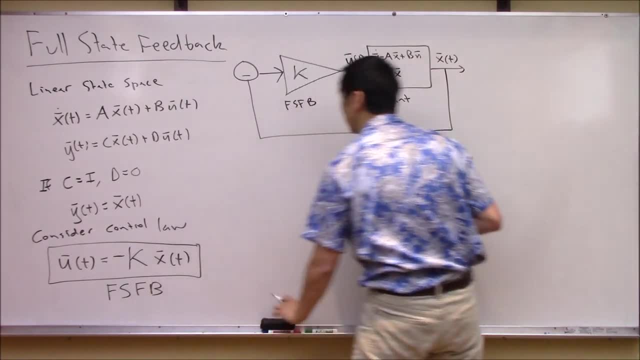 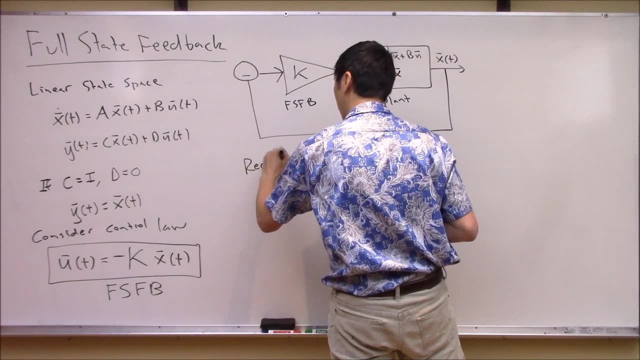 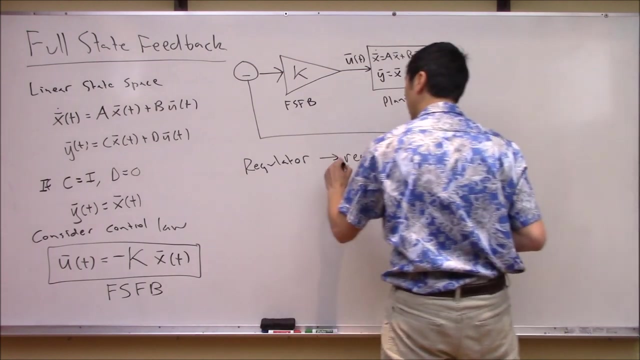 let's keep it simple and say that this is the overall system. So this is again- let's just write this down- that this might be considered a regulator, Because what it tries to do here is regulate non-zero initial conditions back to the origin. 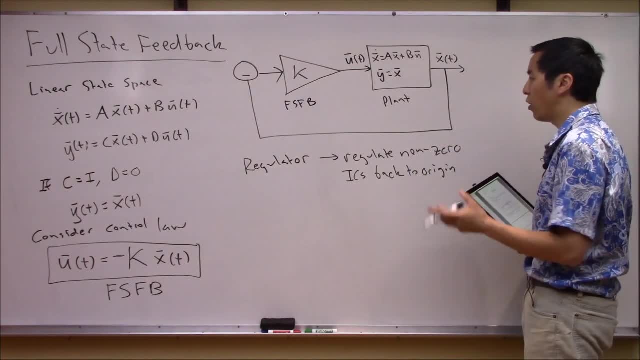 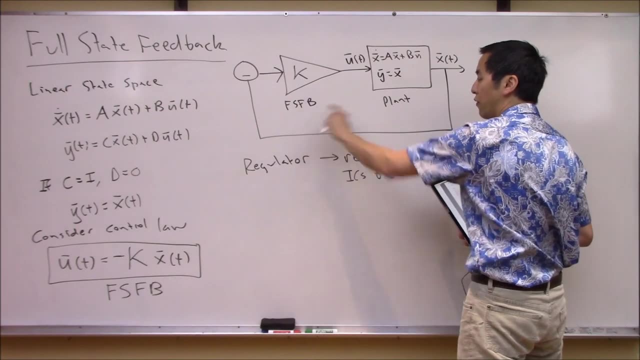 Again. so this is the concept of. there's no reference signal for it to track. All it does is, if the system starts at some non-zero initial conditions, this control law here, or this full state feedback controller or regulator, will try to regulate the states back to zero. So just a. 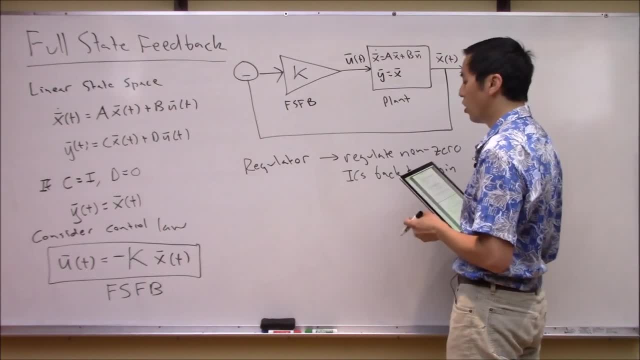 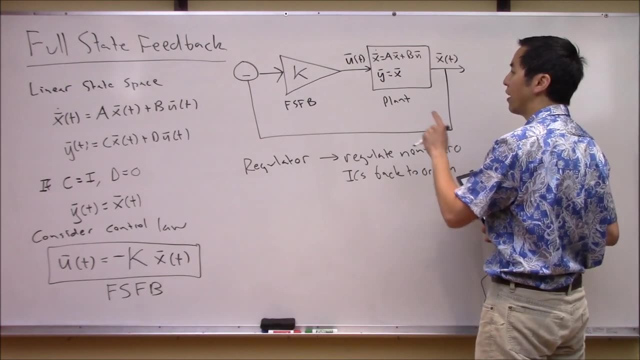 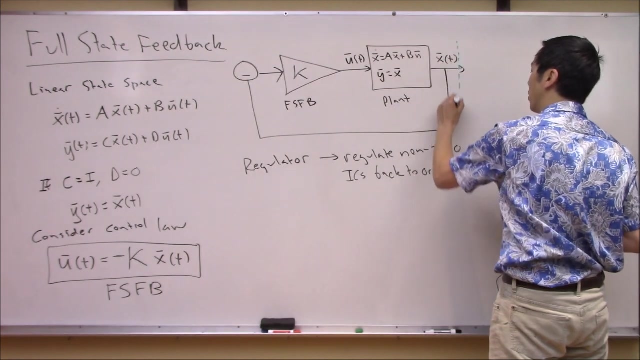 little side note that I think we I want to point out. okay, so why don't we take another step? With this in mind, we can almost ask now: how does this overall system behave? so maybe I will, maybe I'll draw a little dash box around this thing in green. 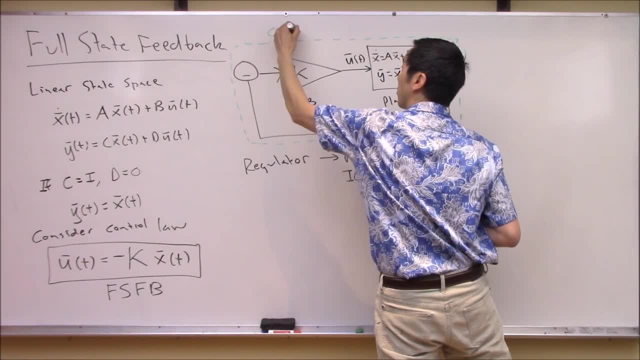 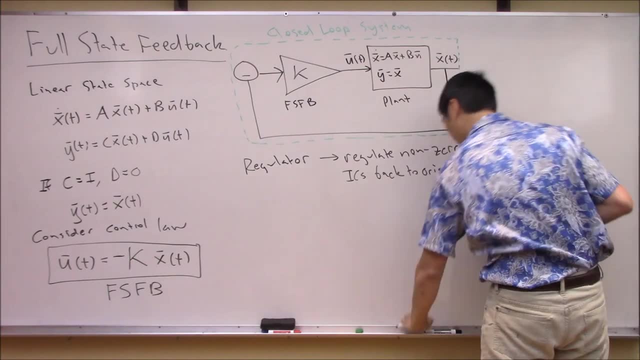 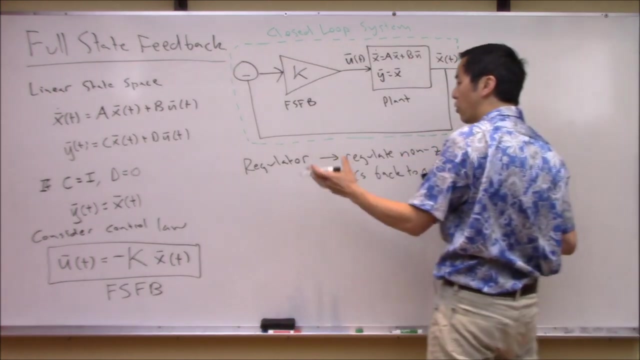 So this green you can kind of think of as the closed loop system. So actually, what's interesting about this is that I'm just going to extend this arrow out a little bit. right Again, we see that there's no inputs to the green box. right, There's no reference. 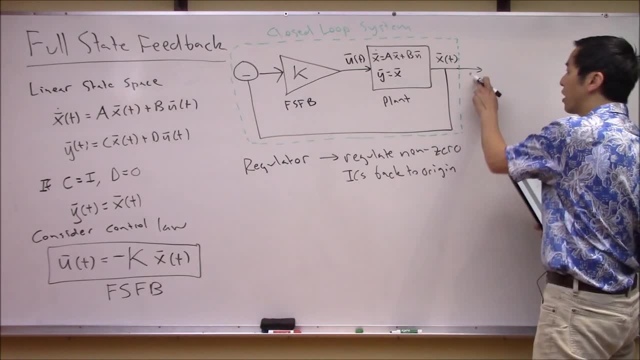 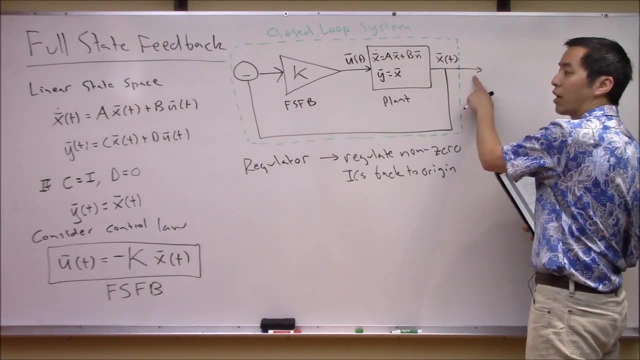 signal. There's no disturbance torques. There's no, nothing like that. The only thing that comes out of this is X, So it's almost like it's an autonomous system by itself. right, It just responds to initial conditions and it spits out what the state vector does under this control. 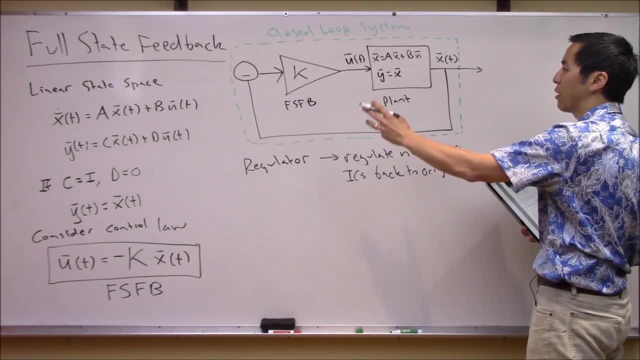 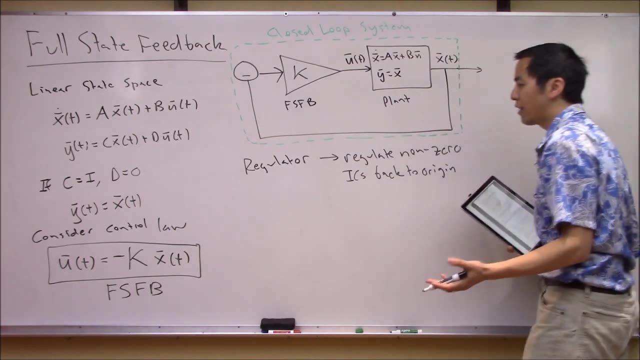 law. So why don't we try to write down what are the closed loop dynamics of how does this green box, how does the overall system, the plant that is being controlled by this full state feedback control law, how does that evolve? So it's actually pretty simple, So let's go ahead and write down. 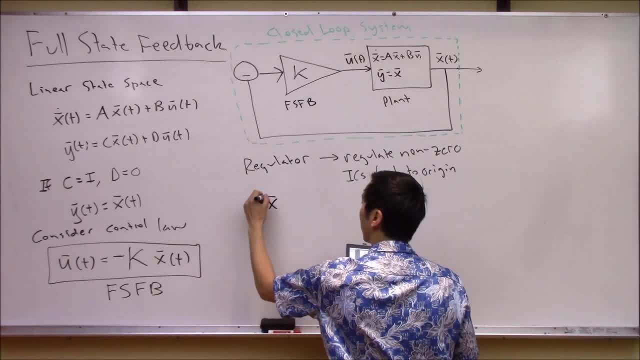 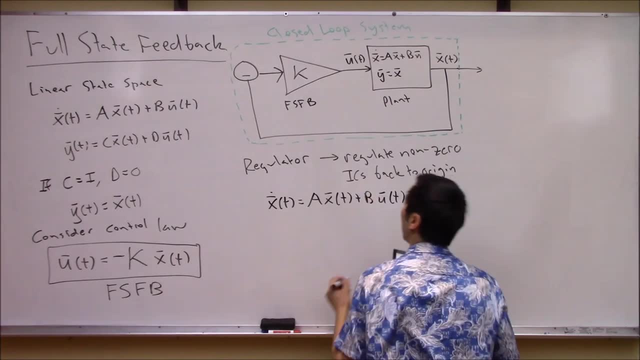 the dynamics. So we know the dynamics of the plant here. right, Our X dot is equal to AX plus BU, right, Okay, now we're going to make a note that. well, what is U? Well, our control law said U. 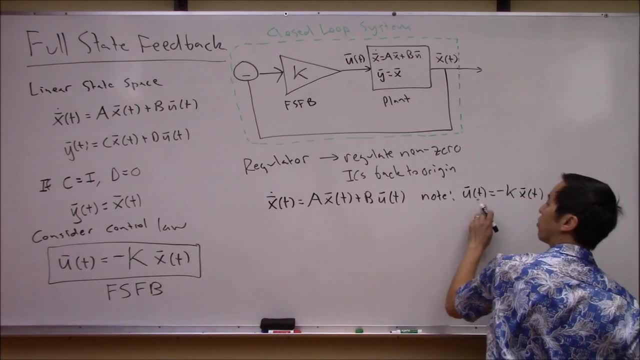 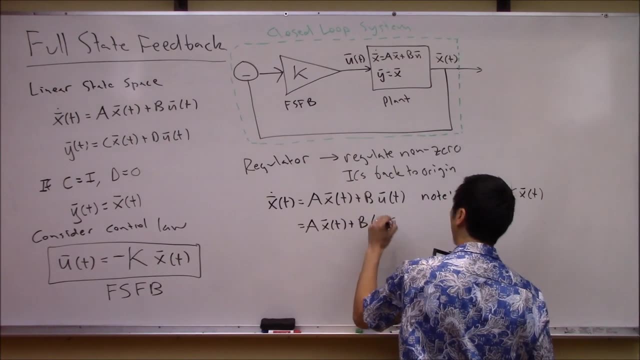 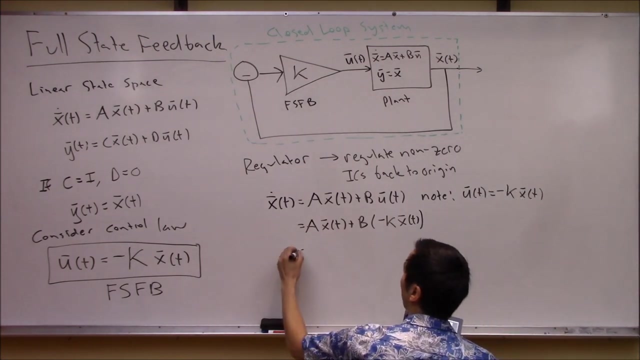 was minus KX, Right, So just substitute that in for U, So we get AX plus B, negative KX, right? Okay? so let's distribute this B through, So we got what AX minus BK? And again, make sure you're not flip. 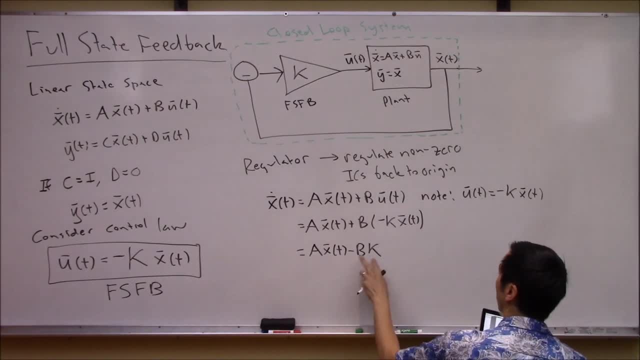 flopping. These are all matrices, right? These are matrix multiplications, So you can't just flip, flop the order. Where are we? Oh, here we go. Oh yeah, sorry, Minus BKX, right? So let's pull X out on the other side, So you have A minus BKX. 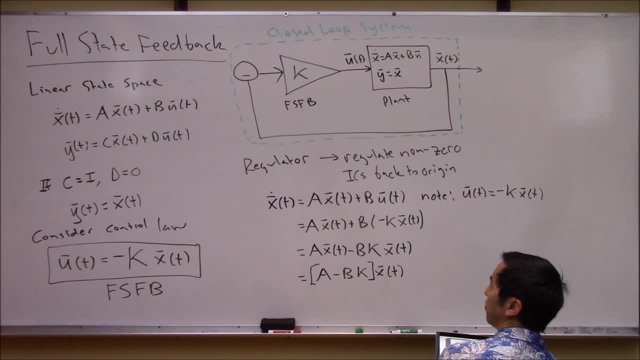 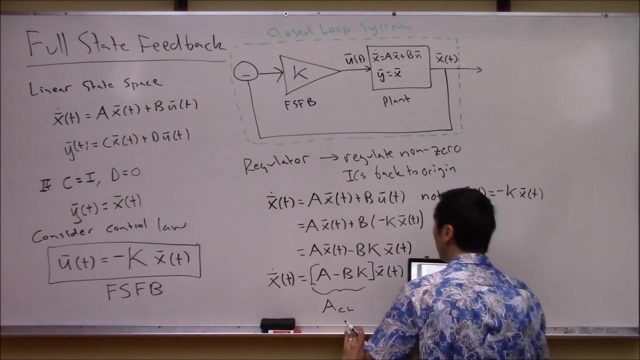 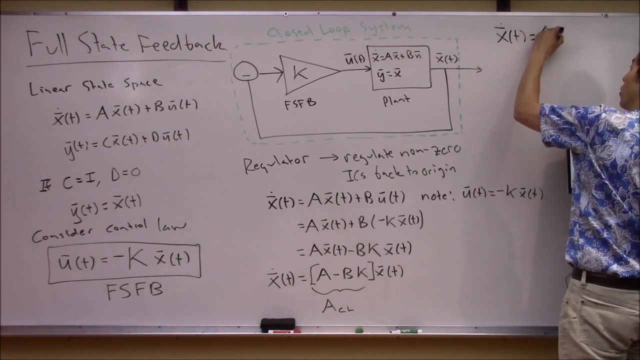 right. And now if you look at this, you have X dot is equal to some matrix X. Why don't we call this A closed loop or ACL? okay, So the overall, the dynamics of the green block are basically: X dot is equal to A closed loop, times X. 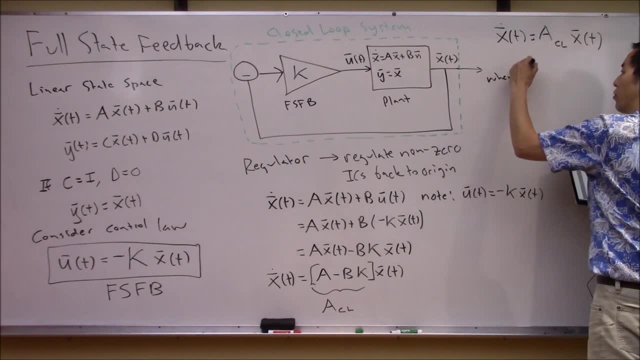 And again this back, and maybe we should make a very explicit note here. So A closed loop is A minus BK, right? So again this backs up our discussion here of the green box. There are no inputs to the system, right? It's just an autonomous system Or you can think of. 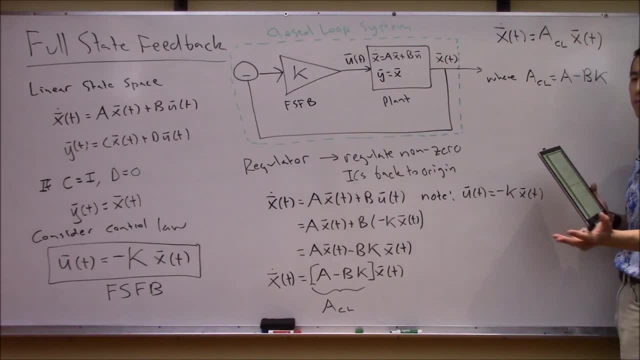 it from a differential equation perspective. It's a homogenous system. There are no external inputs to the system And you see, the only way that you get state trajectories are in response to a non-zero initial condition in your state vector, right, Okay, so this is. 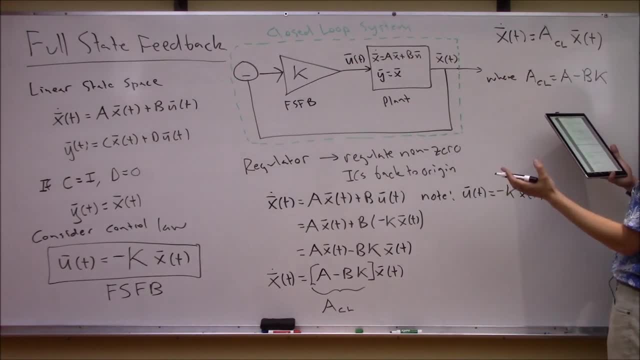 beautiful And basically, the next thing that we should ask now- and we see from this formulation here- is that we know that the way that this thing is going to evolve is basically determined by this ACL matrix right. So we should say it here that the behavior of the closed loop system is governed by ACL right. 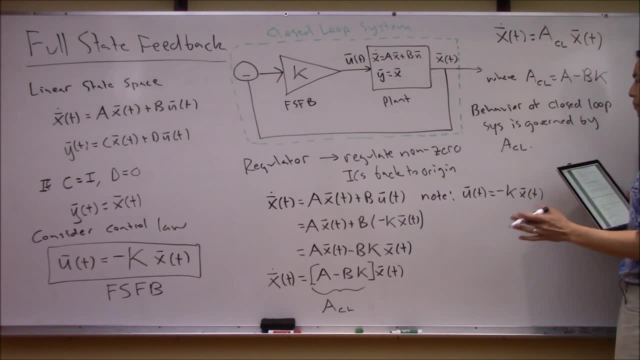 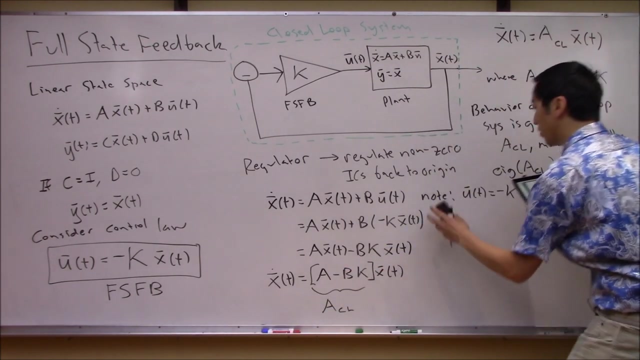 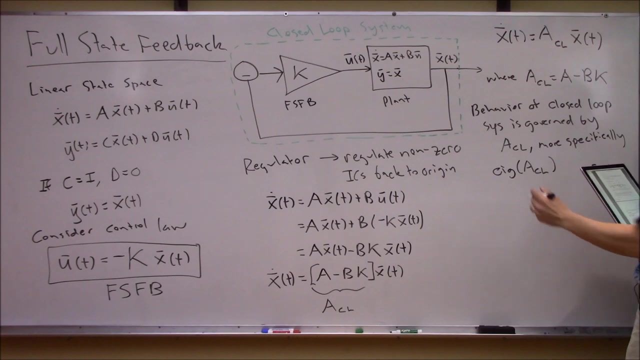 And, more specifically, the thing that we're usually caring about here is the eigenvalues, right? So more specifically by the eigenvalues of ACL, right? That's what we care about, And let me erase this because it's kind of getting in our way of our discussion. okay, So your job as a control engineer might be to ask: 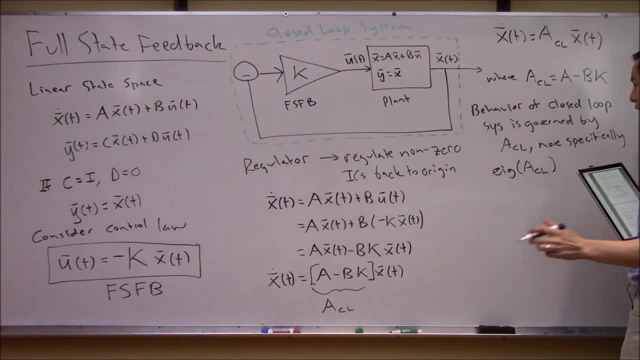 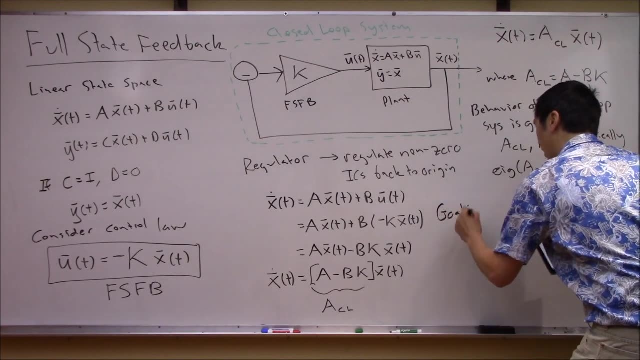 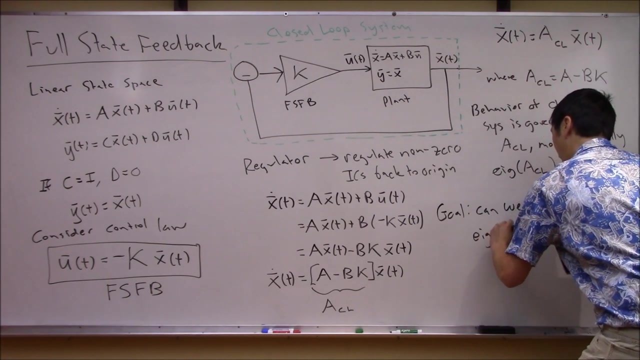 you should probably be thinking: is there some knob or can I change the eigenvalues of A closed loop right? So your job or your goal here is: can we move the eigenvalues of A closed loop right? Well, what in here do you get to play with, right, Do you get? 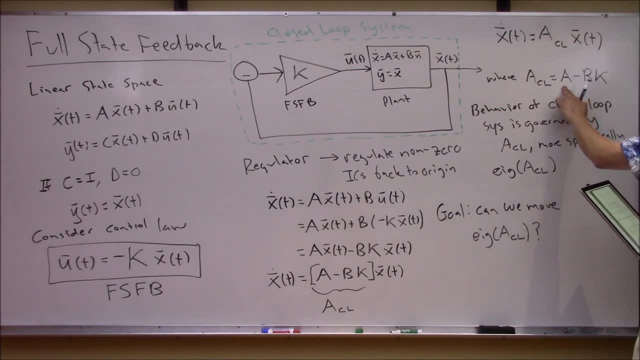 to play with A. No, Typically that's part of the plant, right? This is like the dynamics. Your aircraft has already been built, so you don't get to change the A matrix. Similarly B. The B matrix was the control matrix or the control input matrix of your original open loop plant. So again that. 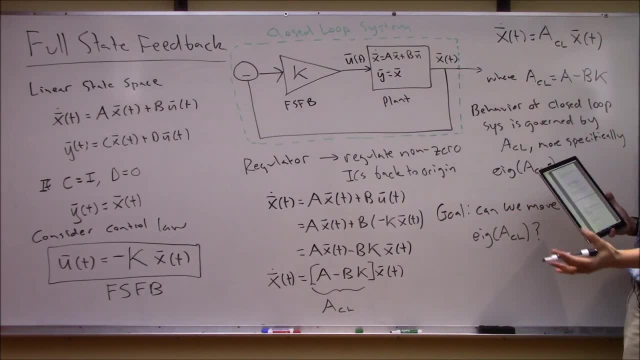 has something to do with like how many engines are on the aircraft, where are they mounted? what kind of purposes do you have all that kind of stuff? Again, you usually don't get to mess with B right, However, K right, The K from your control law that you do get to mess around with. So the 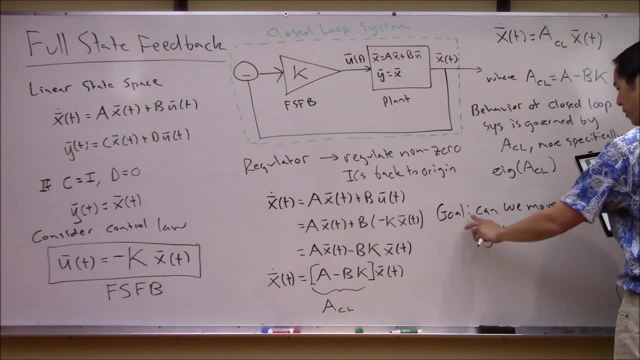 question. maybe instead of saying goal, we should pose this as a question here of: can we move the eigenvalues of ACL? Well, if you look at this, the way you can do this is by changing the K matrix. you can hopefully change the closed loop, A matrix, And now, hopefully, you should be. 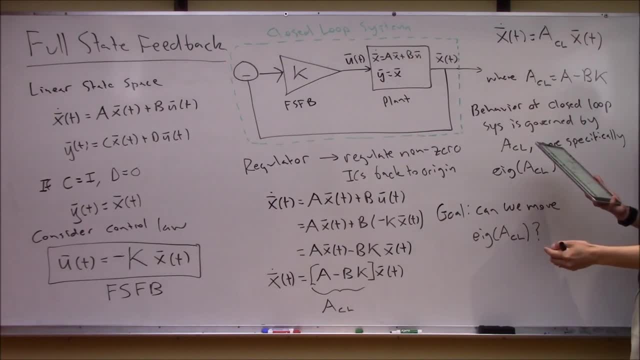 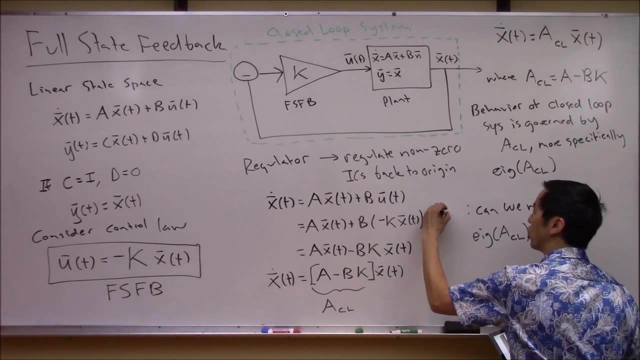 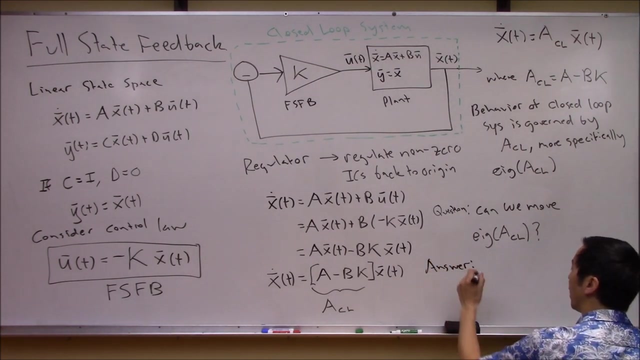 be able to change the eigenvalues of that closed loop, A matrix. okay, So yeah, maybe we can pose this again. Goal is the wrong word. Let's put this as a question, right. So the question is: can we move eigenvalues of ACL? And the answer is yes, Eigenvalues of ACL can be placed anywhere. 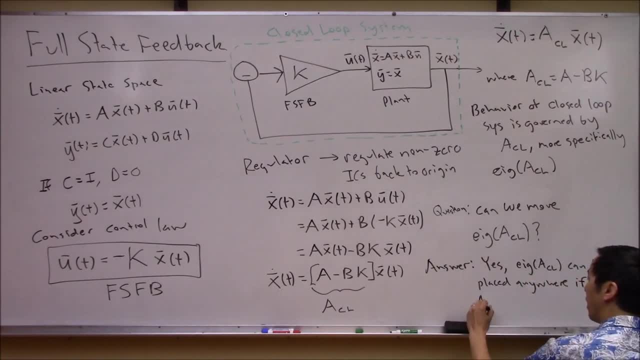 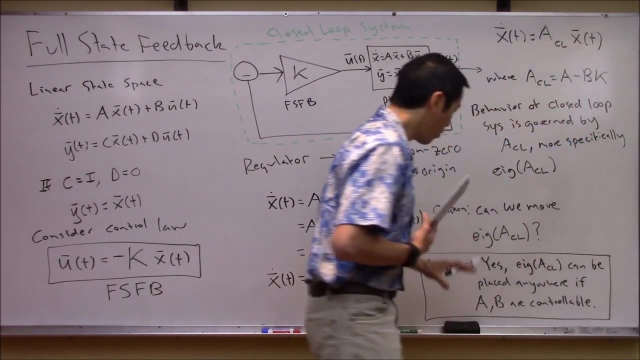 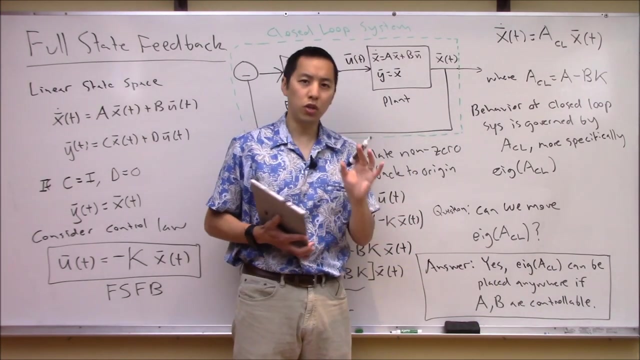 if A and B are controllable, okay. So let's, let's let's box this up, because this is is is huge and very, very interesting, Although we might need to take a take a step back here, okay. So, first off, this concept of controllable here, make sure that you've watched our other. 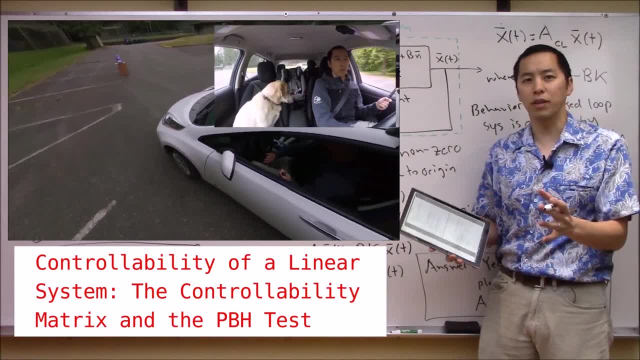 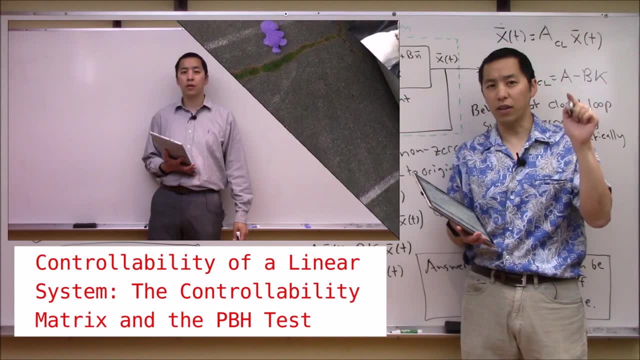 video right, This one over here that talks about controllability. right, Because you know that talked about how to test if a system was controllable, And you can get to that video again. there's a link to the URL in the description of this video or click on the card right up here. 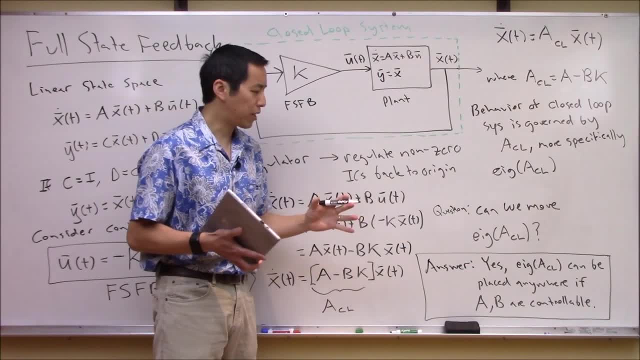 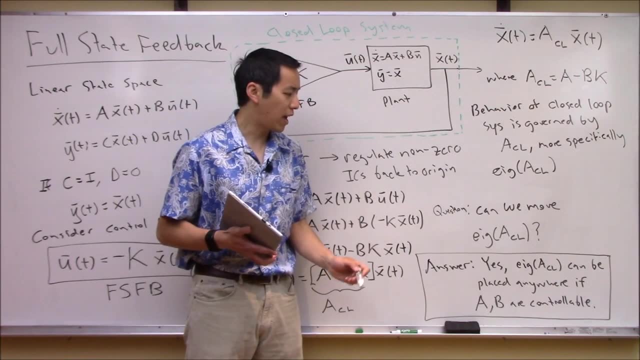 okay, So if your system is controllable, let's get back to, maybe, the ramifications and the discussion of this. right? If your system is controllable, what this claims here is that, yes, you're able to manipulate the eigenvalues of the closed loop system to anywhere, right? 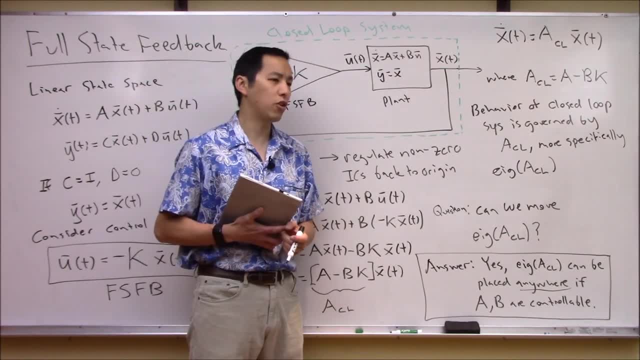 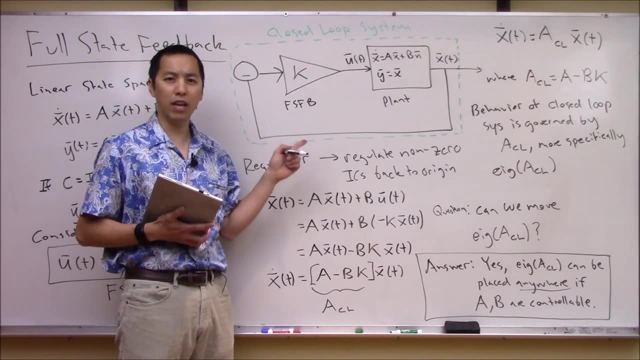 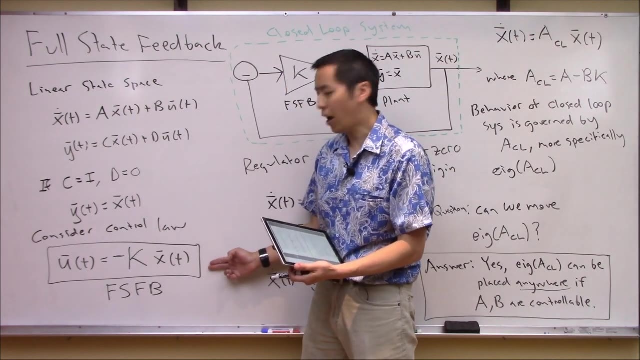 Okay, That is incredibly powerful, right? You're basically saying that I can make this system here respond or behave any way I want. I can put its eigenvalues anywhere, okay, And furthermore, let's look at the control law. right, How did we do that? How are you going to do this? You're 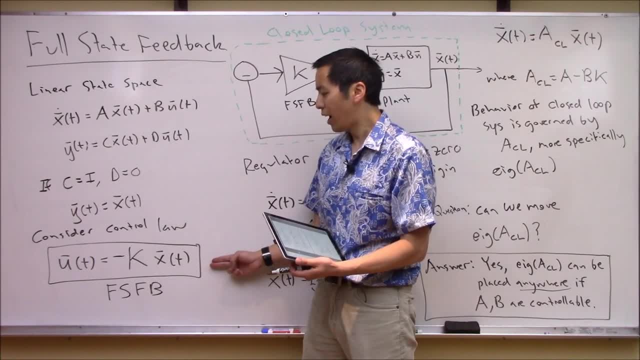 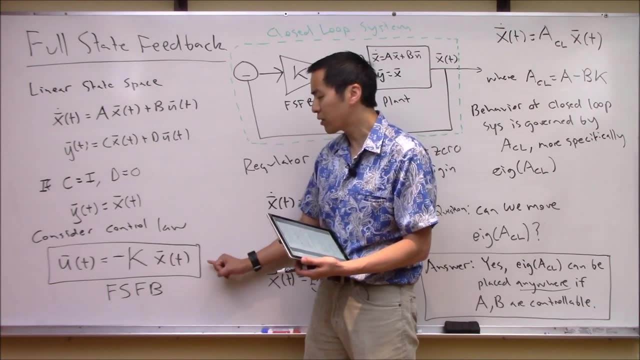 going to do this with this ridiculously simple control law. right, I don't see any integrals, derivatives, zeros, poles, any complicated behavior here. There's nothing. This is almost like, if you think about this, this is almost like a control law. You're going to do this with this. 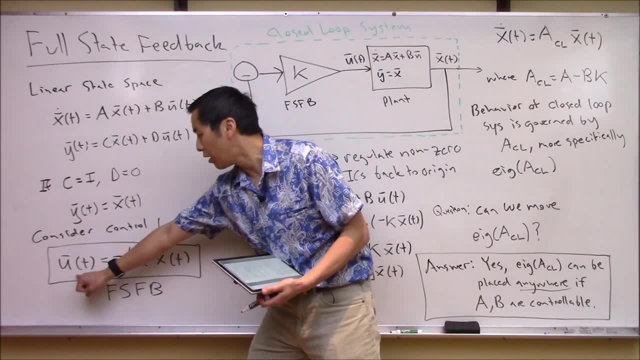 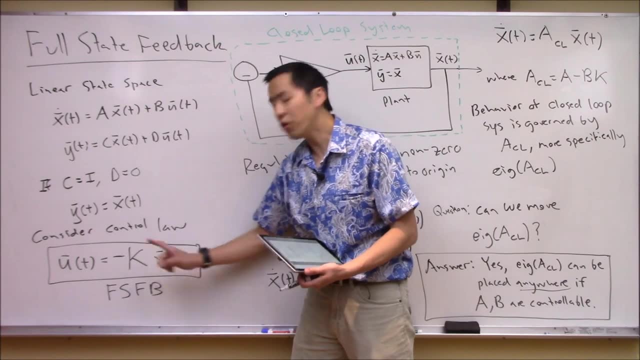 stupid proportional controller. right, Because the control law right here that you're computing at the current time, t, is just dependent on the current state right now, And all you're doing is you're multiplying it. right? This is just a big fat matrix: multiply So the control is just directly. 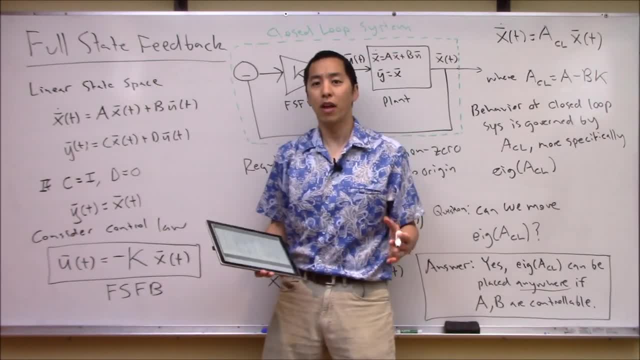 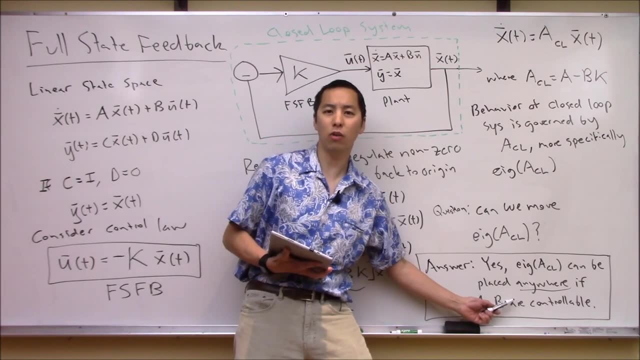 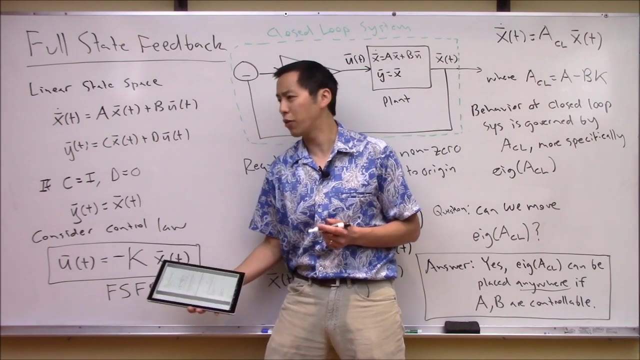 proportional to the current state. So this is what we were talking about, that you get the best of both worlds. You get power. You get incredible power to move the poles anywhere. but it's simple here, right, There's got to be some saying here that goes along with ultimate power and all. 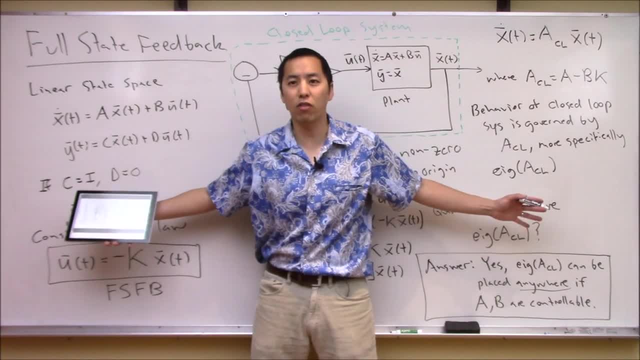 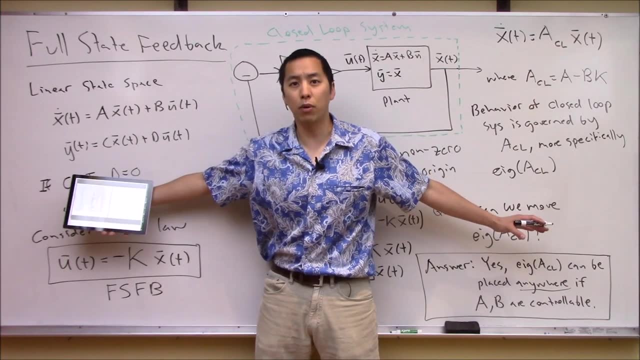 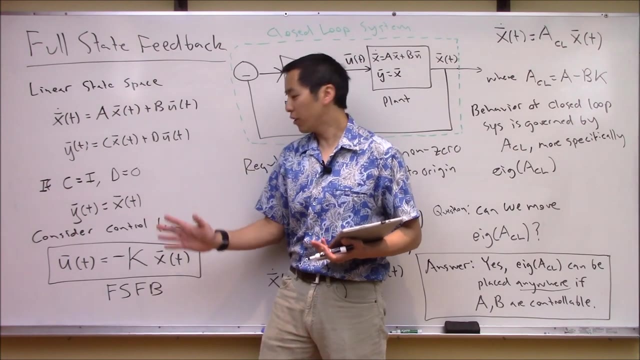 that kind of stuff. But this is the gist of it, right? So here's the large scale picture of you get incredible amount of power with a very simple controller. okay, So tell you what let's talk about now. the next thing is, now that we've got all this power, we see that, the way you get that. 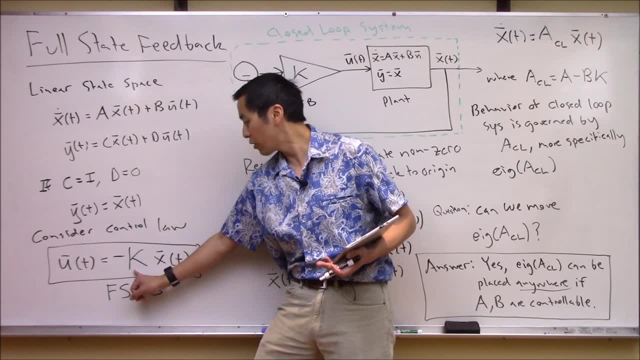 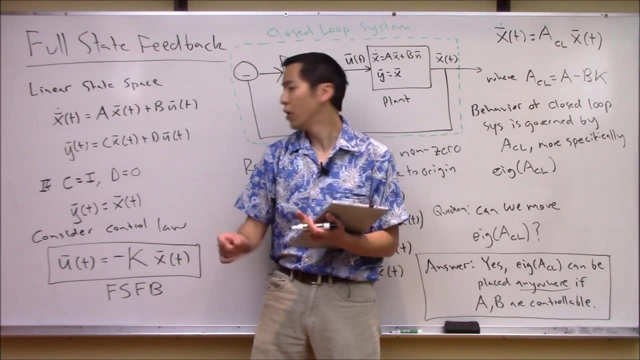 power is by intelligently choosing this matrix K. okay, So the way you get that power is by using this matrix K. So that's the whole game, with full state feedback is: how do we pick this matrix K to get us the eigenvalue locations that we want? So give me a second. I'll pause the video erase. 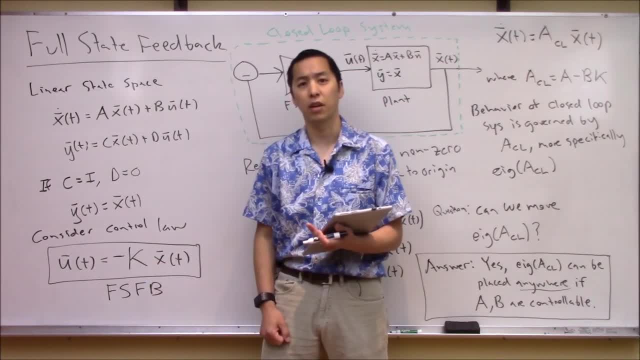 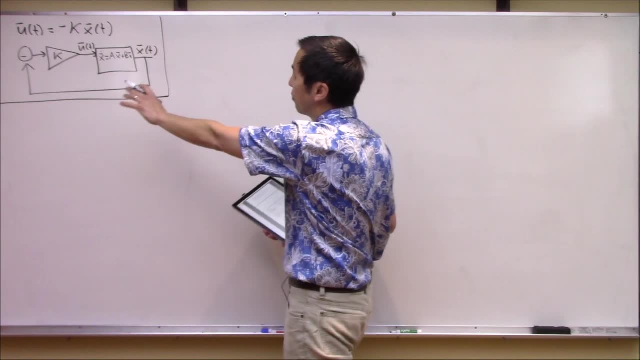 the board and let's jump into an example of how we're going to design this K. All right, so I've erased the board and I've moved the critical information up to the upper left side of the board, right, The control law again was really really simple and building the architecture to 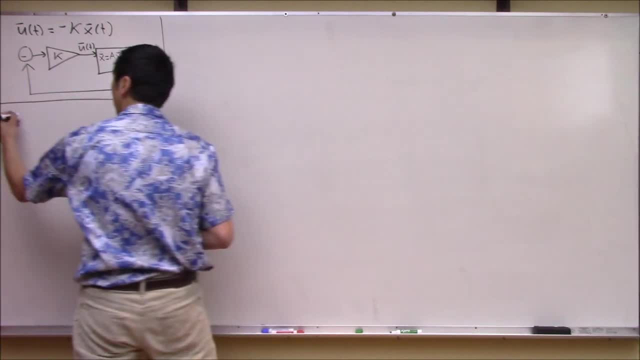 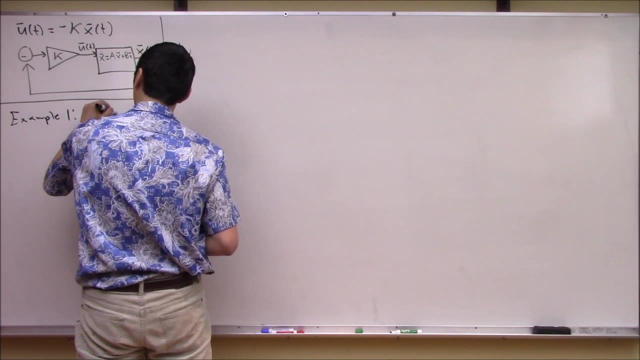 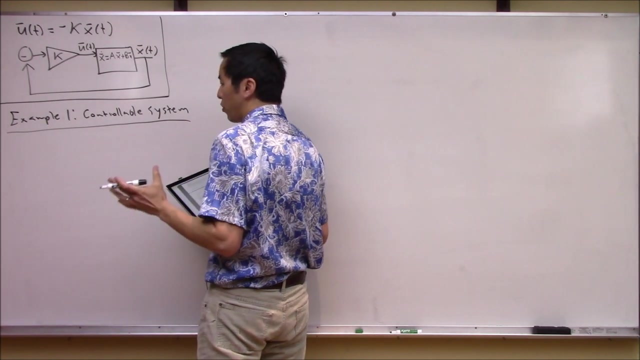 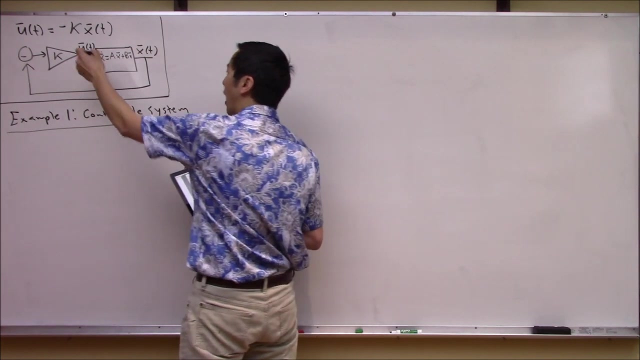 implement that control law was just as simple. okay, So the first example I want to look at is a controllable system. okay, So the idea, like we said earlier, is I need to be able to pick this matrix K here and I want to pick that K such that I put the eigenvalues or the poles of this. 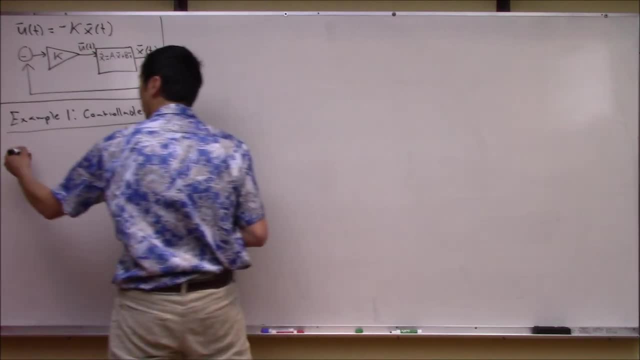 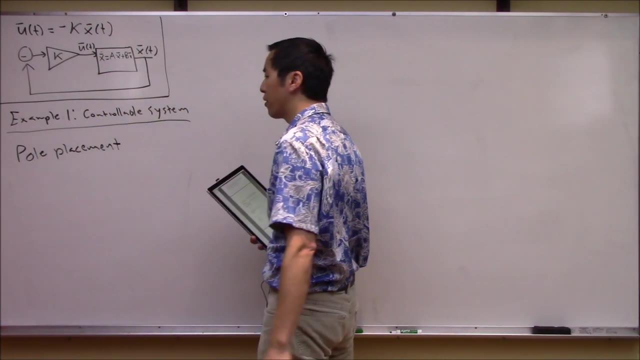 system at desired locations. This is what's sometimes referred to as pole placement, and we're going to see that in a moment. So let's go ahead and do that. So let's go ahead and do that. see that there are various tools and methods that allow us to perform this pole placement. 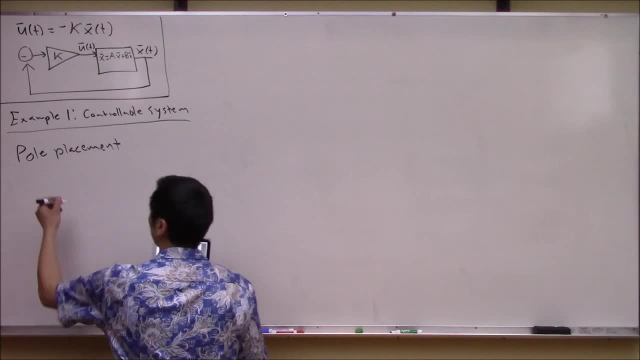 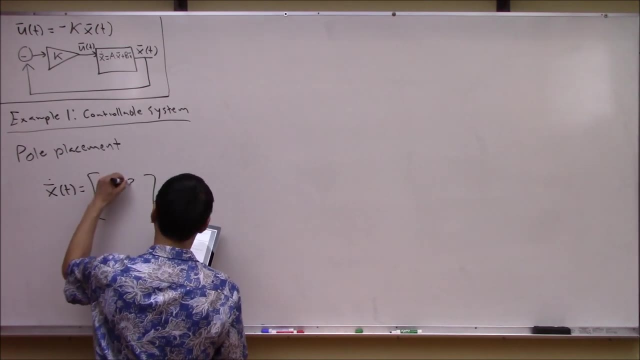 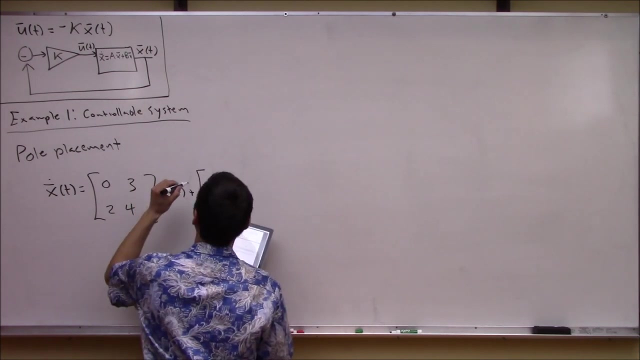 operation. okay, So let's go ahead and start with an example system. So the example system I like to look at is: let's go ahead and use our good old friend again. our linear system. x dot is equal to a, which is just a. two by two, that looks something like this, plus b, which looks something. 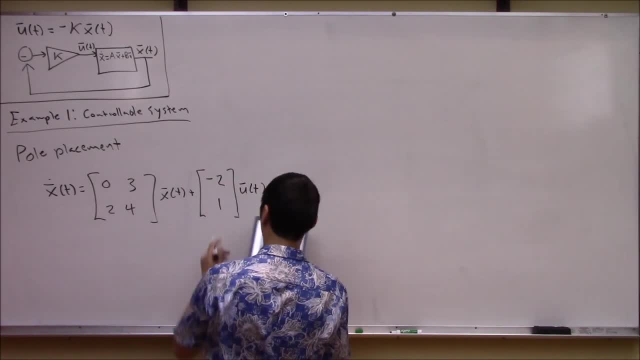 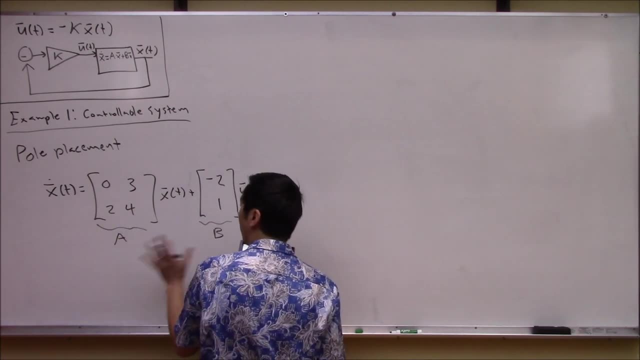 like: how about minus two one u? Okay, so here's your system. okay, So here's your a matrix, here's your b matrix. Now you remember, we said that. okay, if this pair a- b is controllable. 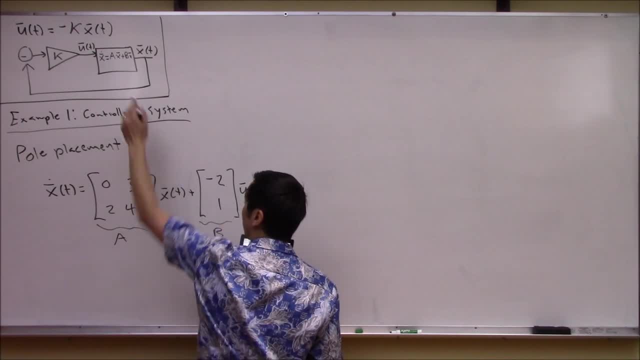 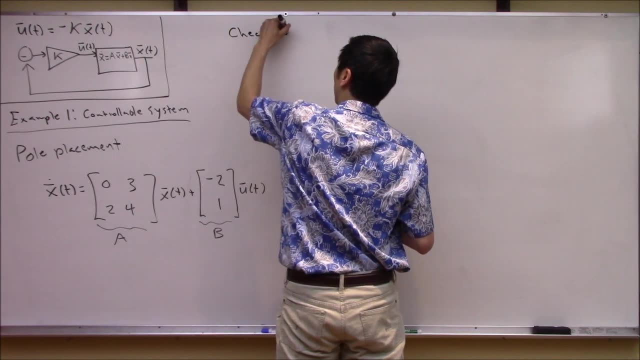 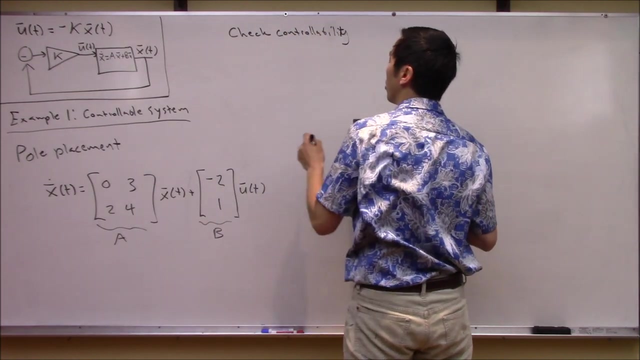 the world is our oyster. we can move these, the eigenvalues of the closed loop system, to anywhere we want. So let's go ahead and first check controllability. okay, So check controllability, So you could go ahead. and did I say ability? right, You can go ahead and use the controllability. 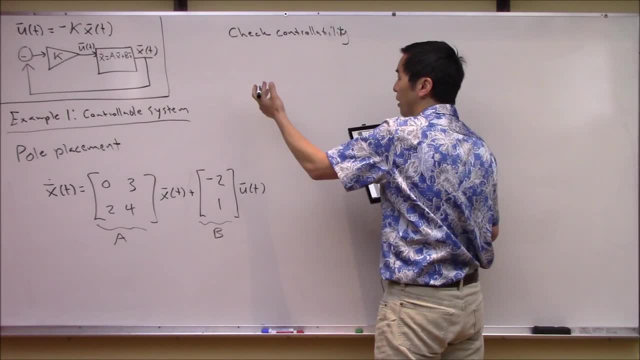 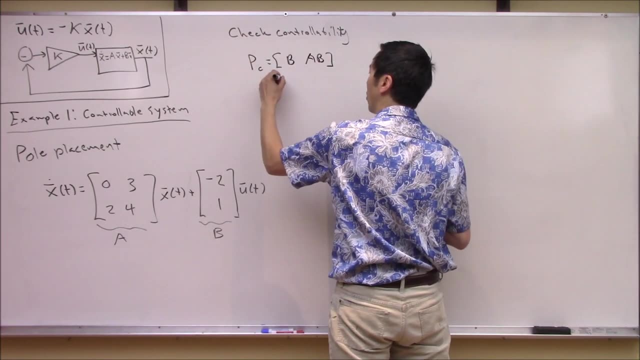 matrix or the PBH test. I think the controllability matrix is probably easier, so let's go ahead and do that. So PC in this case is going to be b and then a, b. So I think if you plug all that in, I think the b matrix obviously is pretty easy to one If you do the matrix. 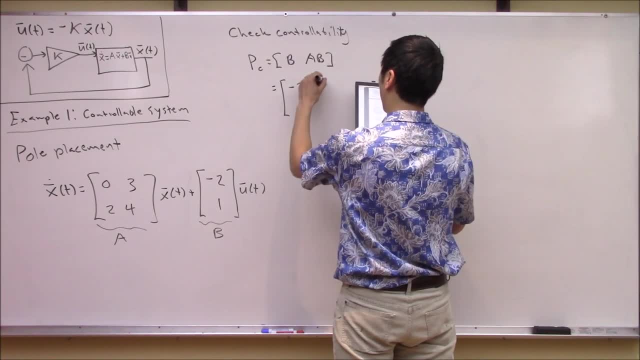 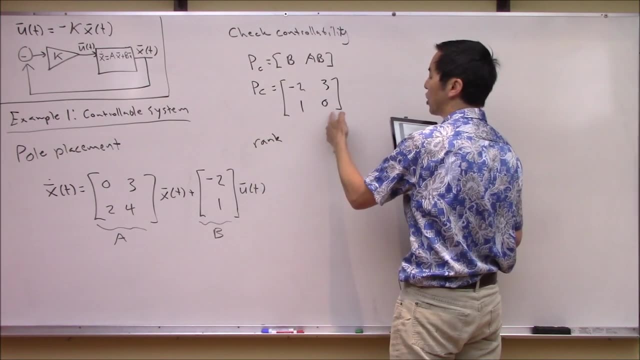 multiplication of a times b, I think you're going to end up with a three zero. okay, So here's your controllability matrix, and if you went and checked the rank- well, I guess you don't even need to check the rank- You can easily see that this first column is linearly independent of the second. 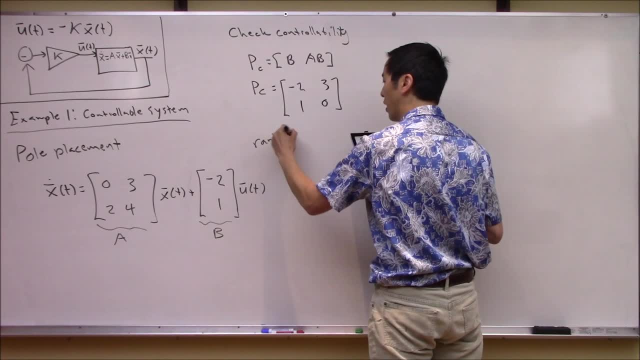 column here right. They point in two separate directions. So we see that the rank of PC is equal to two. So we're going to go ahead and do that. So let's go ahead and do that. So PC, in this case, is. 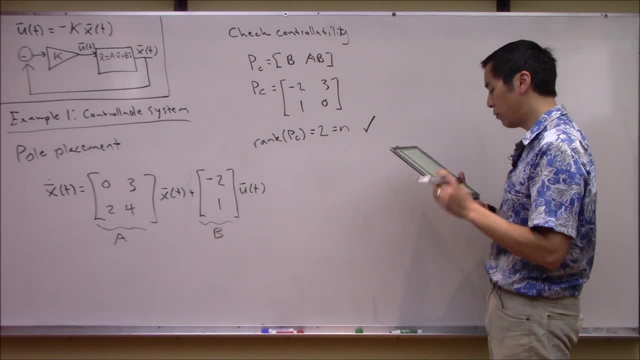 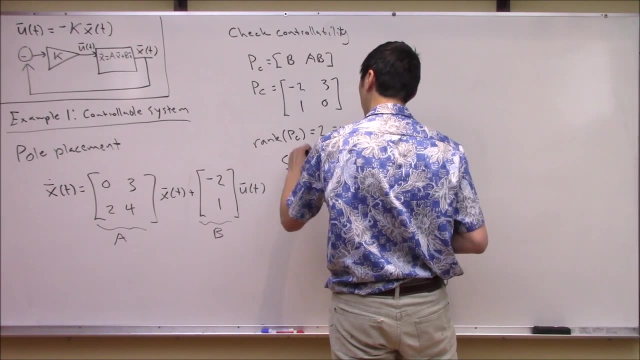 controllability matrix, which is the number of states. So yay, system is controllable. We should be good to go, okay. So now what we need to do here is we need to go ahead and try to solve for k, okay, Or we need some way to pick k. The first thing we should probably do is: what is the 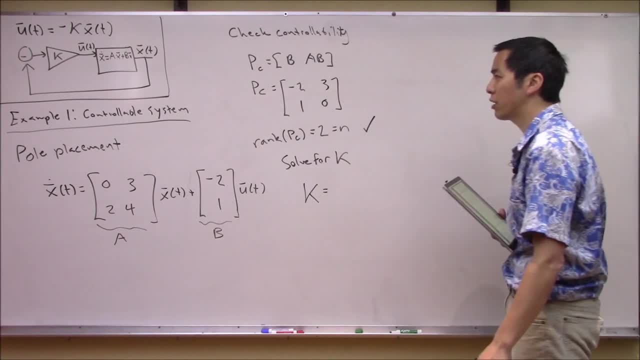 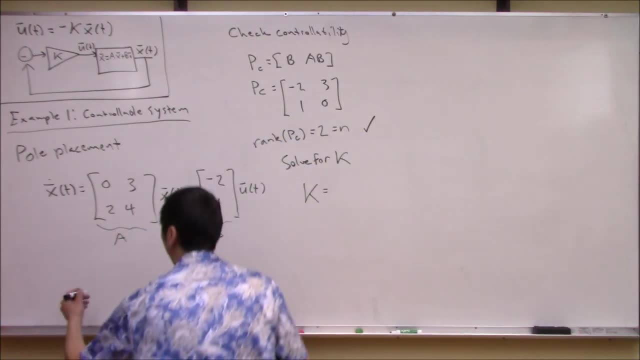 dimension of k. What does k look like? I know, maybe we should have talked about this a little bit earlier, So we said that maybe we should have. let's do it over here. Sorry, we probably should have talked about this a little bit earlier, but just looking at the, 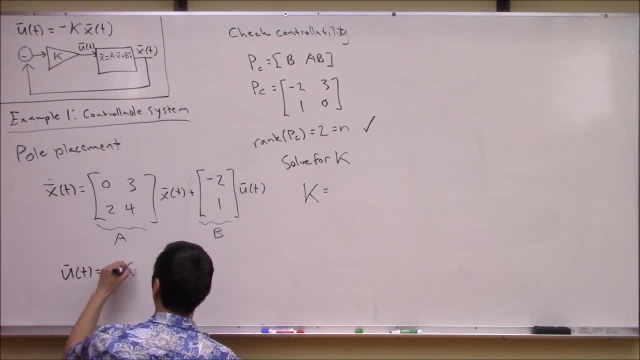 control law. right? U is equal to minus kx. okay, So if you look at this, x, that is your number of states. This is an n by one right. So x here is an n by one vector. What is u? U is the number. 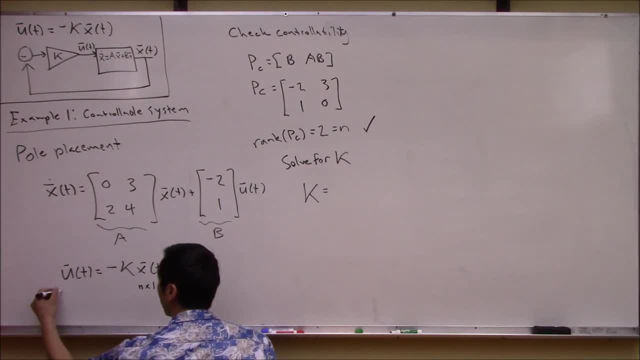 of control inputs that you have in your system, right? So u is going to be an m by one vector here. So again, just to make sure n is number of states, right And m is number of controls, right. So just to make this happen, you can easily see that k is actually. 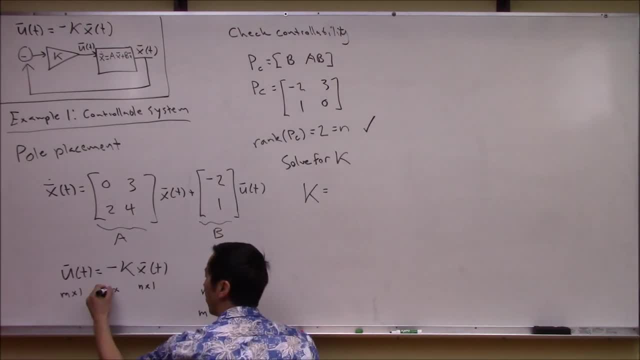 it's actually got to be a matrix of size. what M by n, right? That's what k has to be in order for the dimensions to work out right. So we see, k is going to be a matrix. It's going to have as: 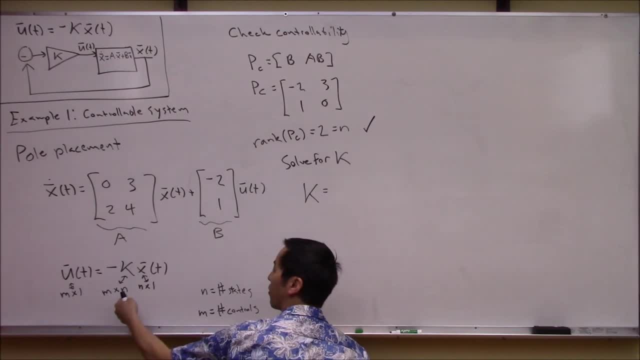 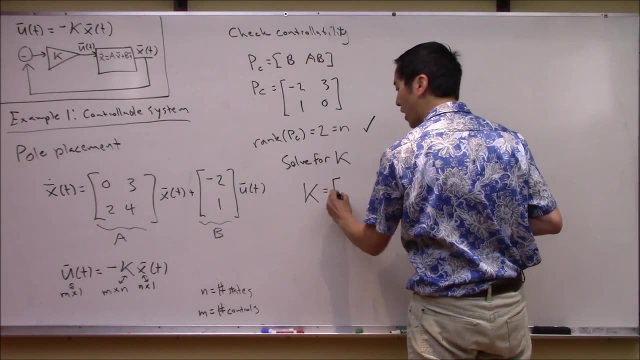 many rows, as you have control inputs and it's going to have as many columns as you have states. okay, So perfect. So in this case, we see that k is actually going to be okay. how many controls do you have? There's only one. 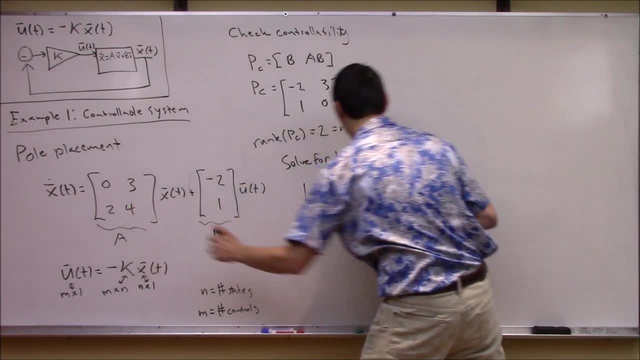 control. so it's only going to be one row. How many states do you have? There's two states, so it's going to be a one by two matrix. So there's going to be like a k1 here and a k2,. 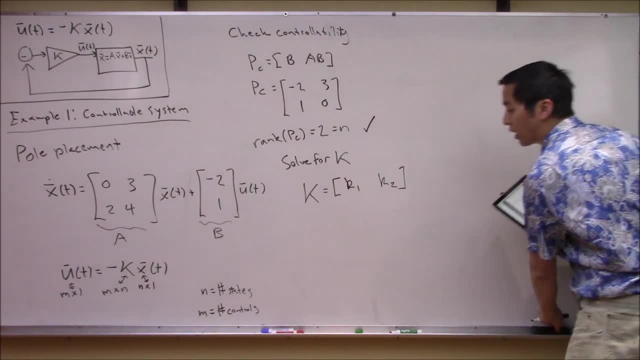 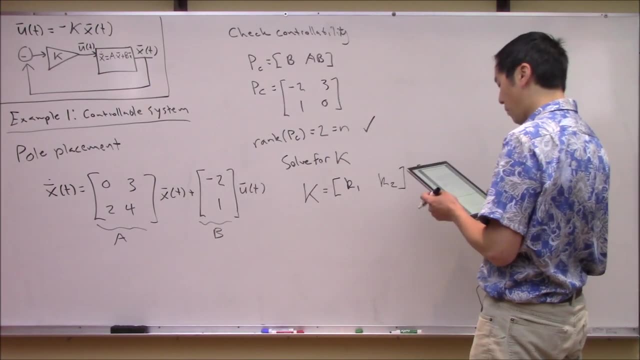 okay, So k again. keep in the back of your head: k is a matrix game, right Okay? so let's keep going. all right, Now we know that this is what our k matrix is going to look like. all right? 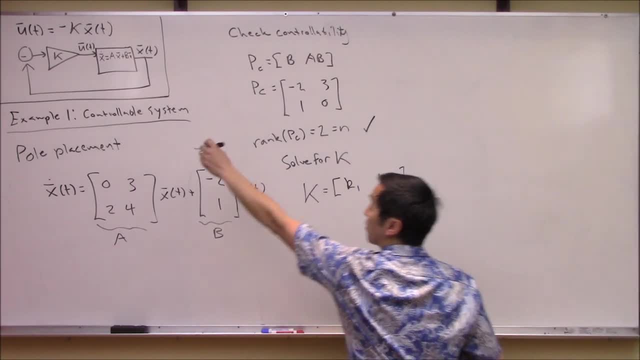 We also know from our previous discussion that we know that the closed loop system of k is going to be a matrix right. So we know that this is what our k matrix is going to look like. So we know that the closed loop of this right, its closed loop, a matrix is going to look. 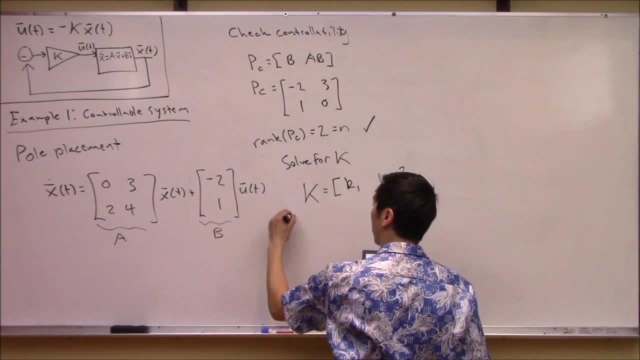 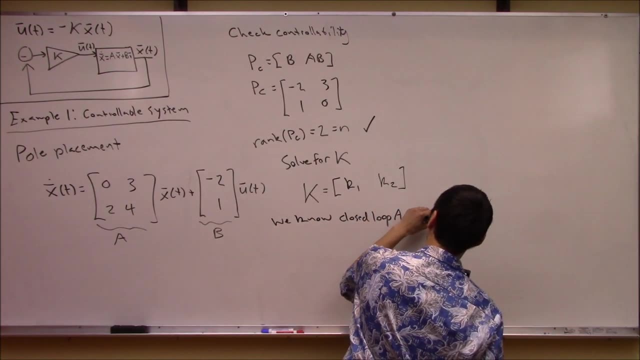 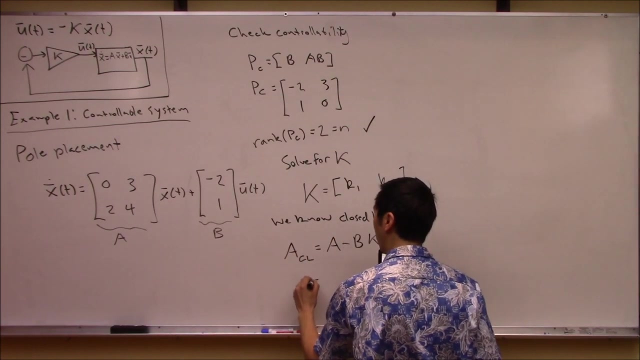 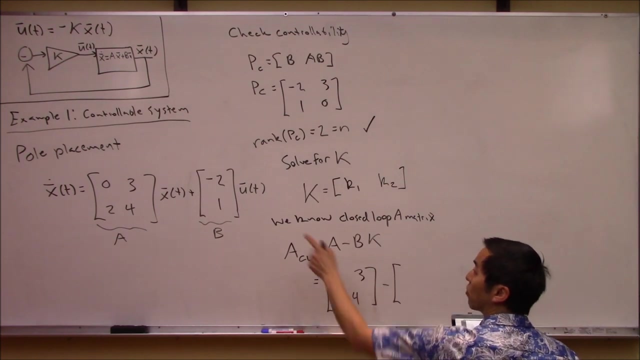 like maybe we should write this down So we know closed loop a matrix is. we called it acl, I think earlier, right, And that was going to be a minus b times k, right? Okay, so your a matrix is pretty simple. It is going to be a 0,, 3,, 2,, 4, minus. what's your b matrix? So it's a minus 2,. 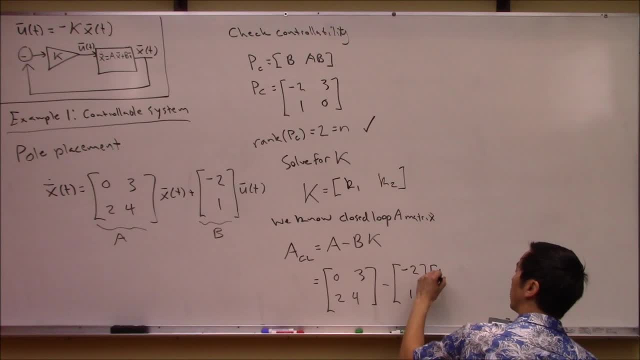 1.. And now we know our k matrix. here is a 1 by 2, it's k1, k2.. So again we see the dimensions work out. So this is boring algebra. let me skip it. You can go over to a mathematic and do this. 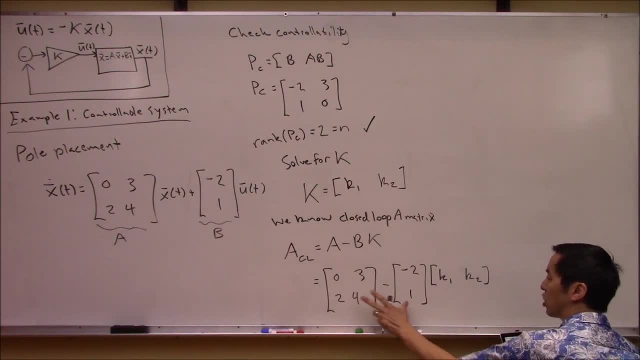 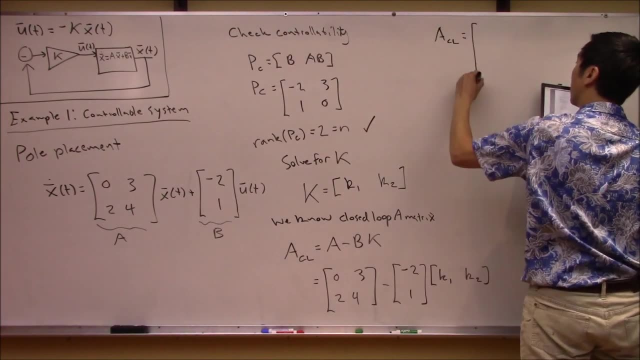 or heck, do it by hand. It's pretty easy to do this matrix multiplication and then the subtraction, But you would basically get that at the end of the day, your acl. this is going to look like again. it's a 2 by 2, all right, So it's going to look like 2k1,. 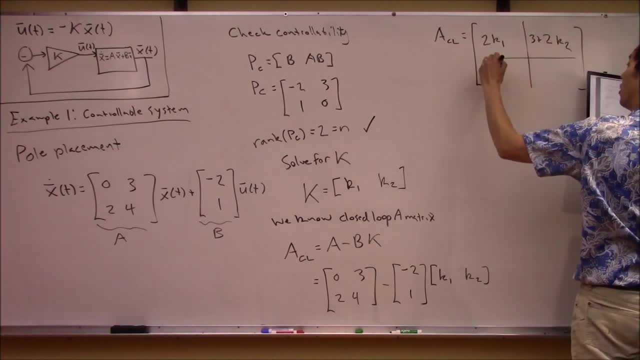 3 plus 2k2,, 2 minus k1, and then 4 minus k2.. Great, So you see that the k's weasel their way into the a matrix, right. So again you should start thinking that: oh wow, you can easily see. 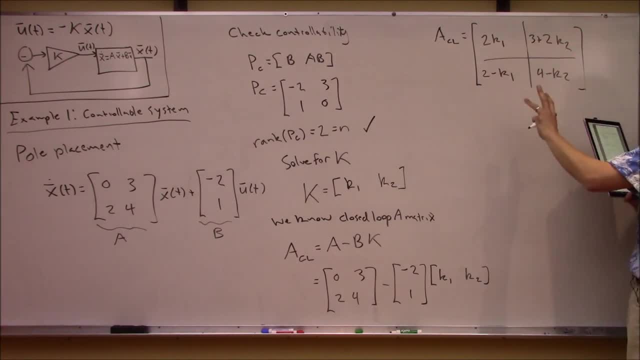 that If I start screwing around with k1 and k2, I change the a matrix. therefore I hopefully change the eigenvalues. So we want to directly change the eigenvalues, then right. So what we should maybe do next is we know that the eigenvalues come from solving basically. 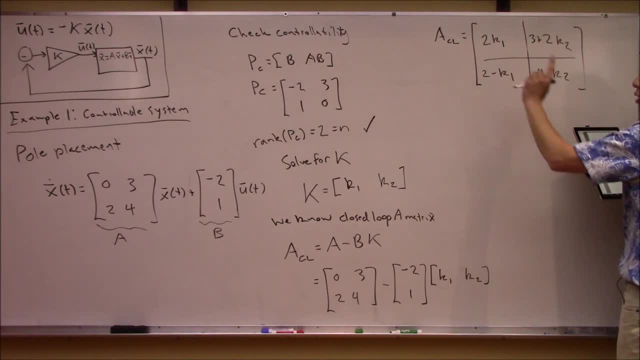 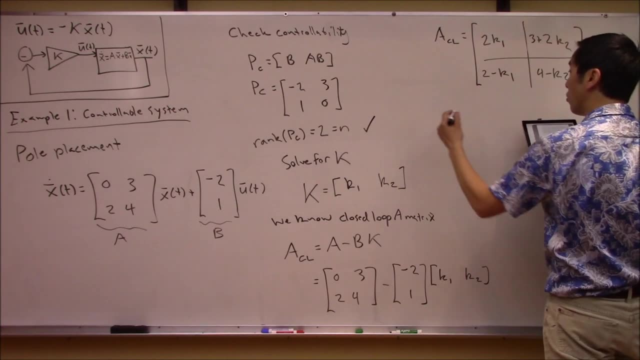 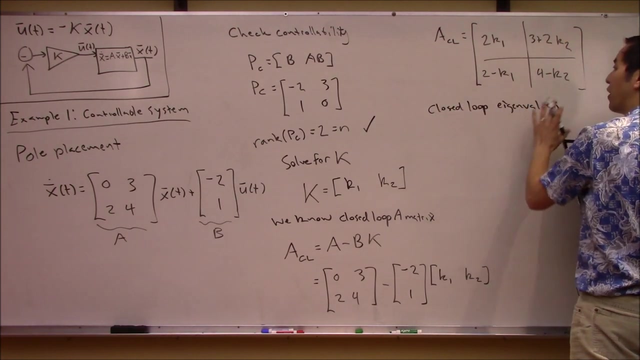 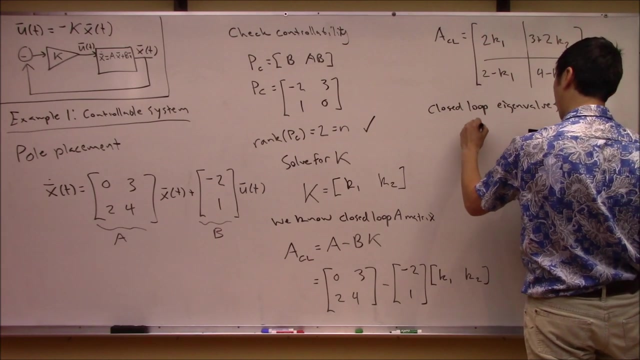 the characteristic equation of si minus a. all right. So why don't we write this down here, that the closed loop eigenvalues right. If you want to find the eigenvalues of any matrix right, you're basically solving lambda. i minus the matrix, right, And you want to solve this thing. 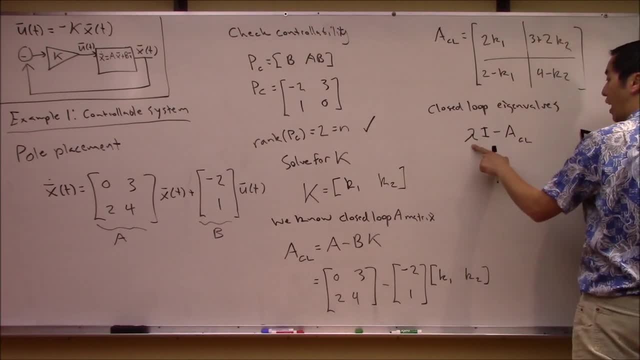 actually you want this to be singular right. So the eigenvalues are the values that make the acl singular. So in other words, I want the determinant of this thing to be equal to zero right. So the determinant of this thing should equal zero right. So those will give me all the 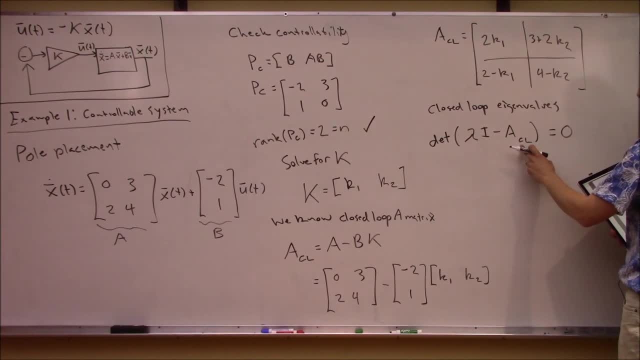 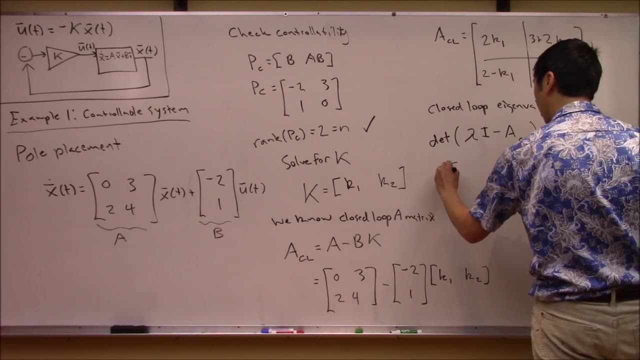 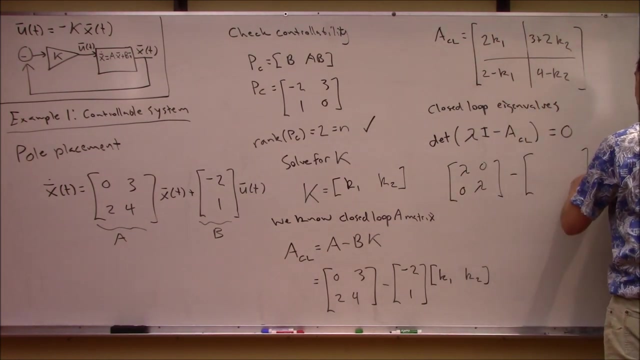 eigenvalues of the acl matrix. right, Okay, so this is pretty simple. So, again, let's go ahead and just do this. So lambda i. so this looks like really simple. It's a lambda, i, right. So lambda 0, 0, lambda minus acl, which is this thing up here, right, 2k1,, 3 plus 2k2,, 2 minus k1,. 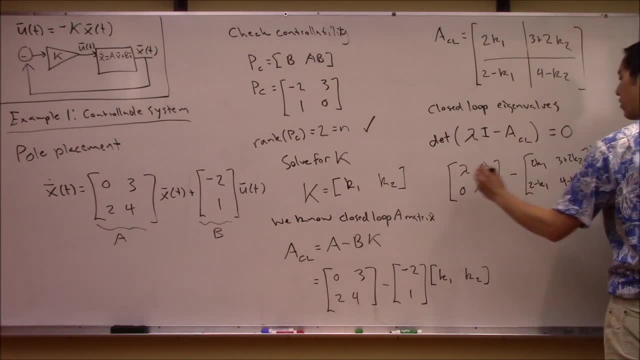 and then 4 minus k2, right. And then I still got to take the determinant of this whole thing and set that equal to zero. So again, you can see that it's not complicated, It's just algebra. at this point, right, Subtract these two, take the determinant, right, Do the diagonals. 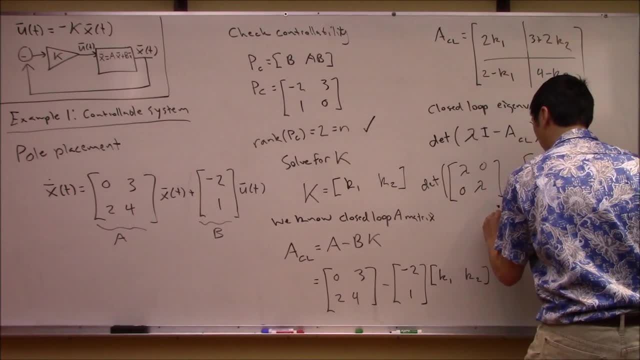 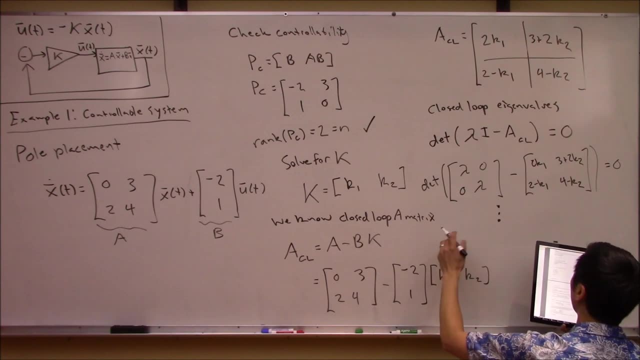 and you will basically end up with again. I'll skip this. The nitty gritty is here in my notes, but I think you can see that it's very simple matrix operations. at this point, You could get this thing to look like: 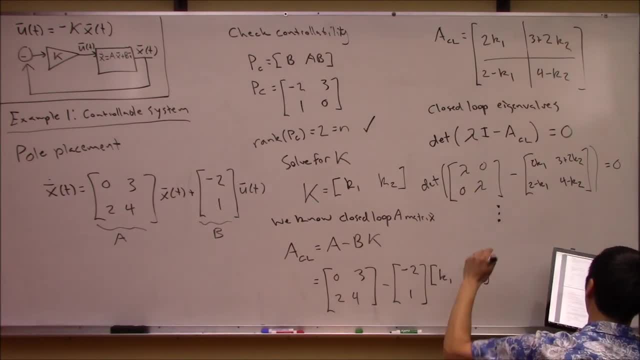 you'll basically see, you'll get a second order polynomial in lambda, right? So what I'm going to do is I'm going to write this in the form of: what do we end up here? We end up with lambda squared plus negative, 4 minus 2k1 plus k2 times lambda. 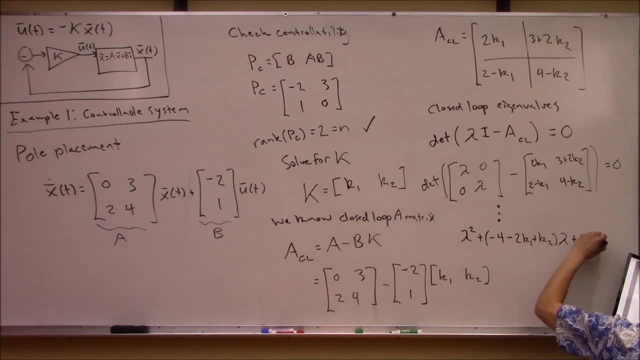 plus 11k1, minus 6, minus 4k2, okay, There we go. Okay, Why don't we call this? this is like your characteristic equation? right, Because this is what I need this to be equal to zero. right? You solve for the lambda values. that gives you the eigenvalues of the closed. 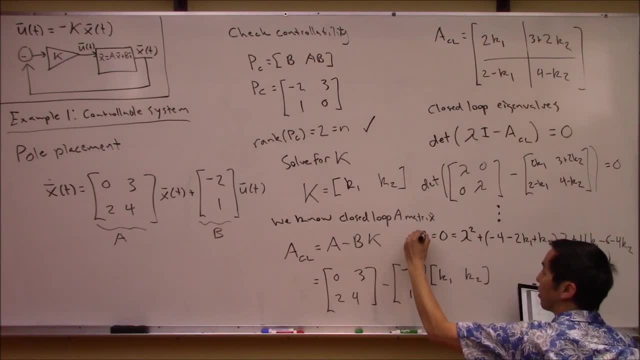 loop system, okay, So let's call this. how about p of lambda? right? So let's box this up, okay, And maybe we'll make a new equation, right? So let's call this: how about p of lambda? 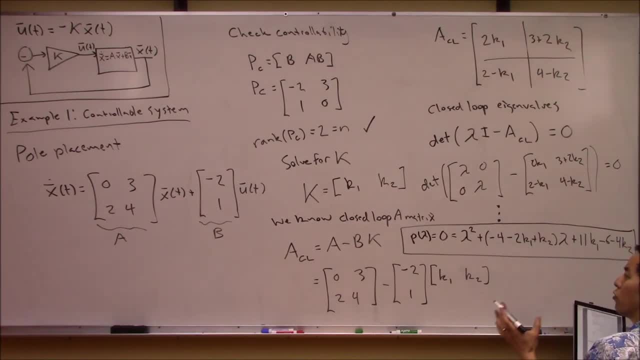 and note here that this is the characteristic equation of the closed loop system using full state feedback of k1,, k2, right? So this is the characteristic equation of closed loop system under full state feedback, right? Okay, And actually, you know what? Let's erase some of. 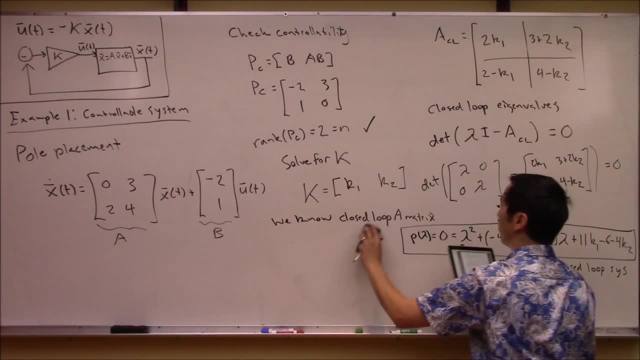 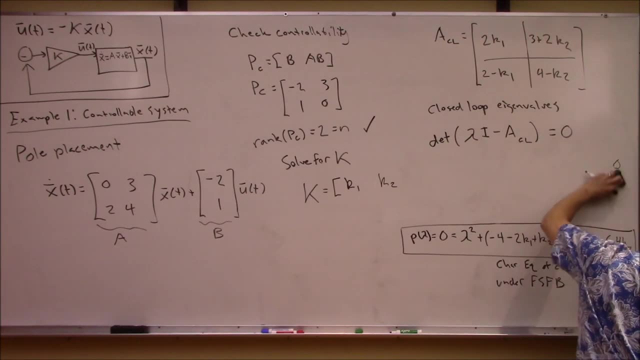 this because I want to isolate this thing by itself, because this is the important bit, okay, Okay. So, all right, We've got ourselves the characteristic equation of the closed loop system. When we use full state feedback, it's going to look like that. So again, you see that. 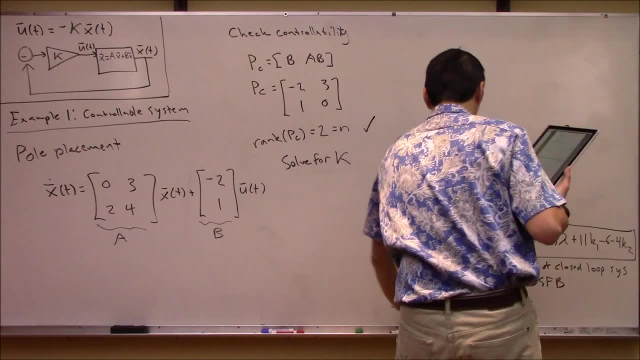 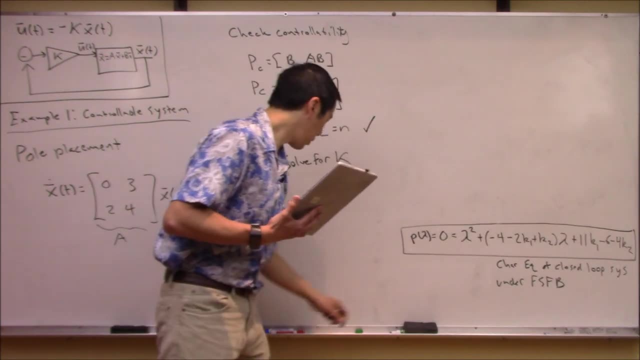 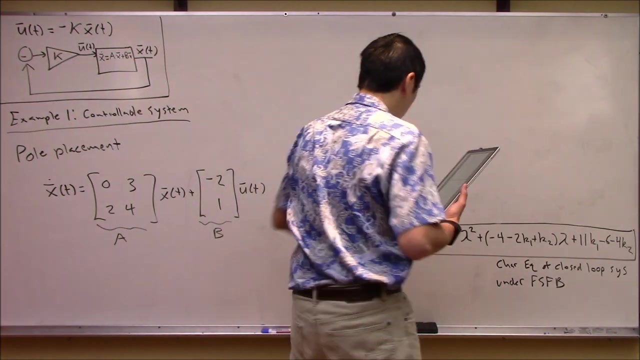 basically, by manipulating k1 and k2, you can change the characteristic equation. Therefore, you can change the eigenvalues of the system. okay, So now the question is: where do we want those eigenvalues to go? okay, This is where full state feedback is so powerful We can now. 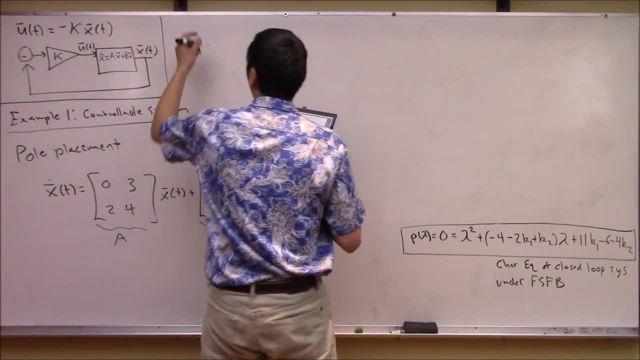 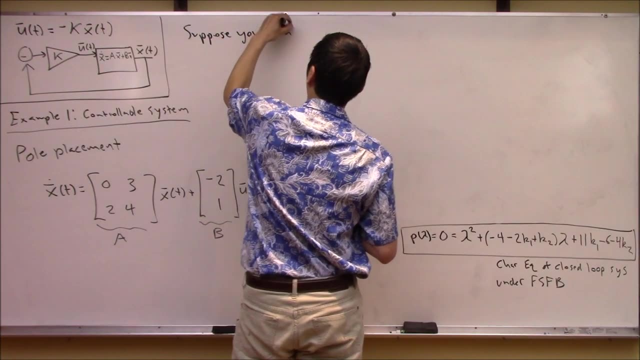 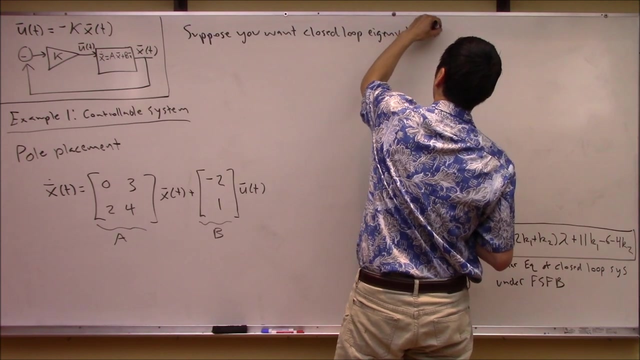 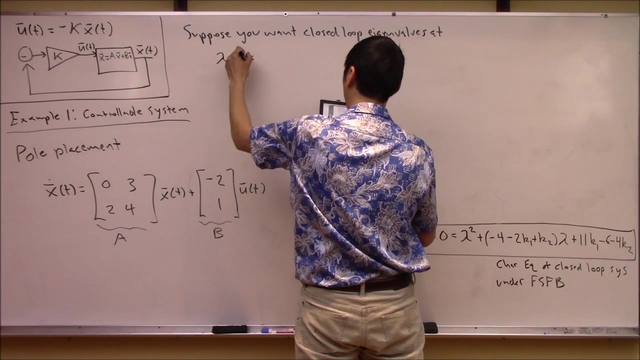 choose. where do we want the poles to go? So, for example, let's say, or suppose, that you want closed loop eigenvalues at a specific location. Let's make something up. How about? I really would like the closed loop eigenvalue, the first one to be here at. I'll make something up. How about minus five? 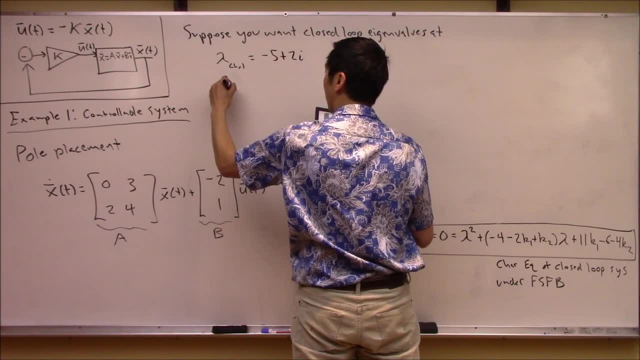 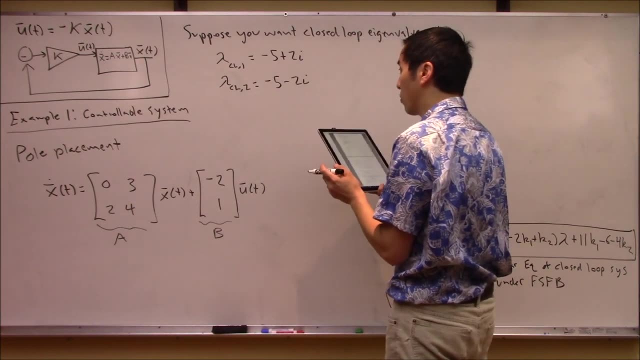 plus two i. And then I would really like the closed loop eigenvalue to be here at. I really like the second closed loop eigenvalue to be at minus five minus two. i right, That's where I want this system to have eigenvalues. I want this overall system here by the time I. 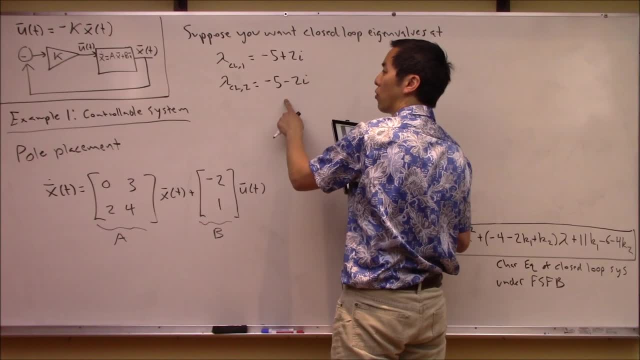 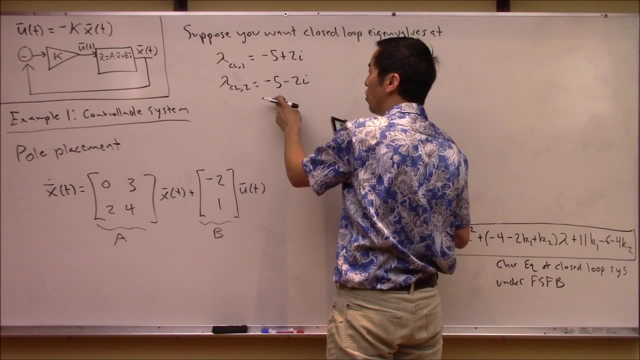 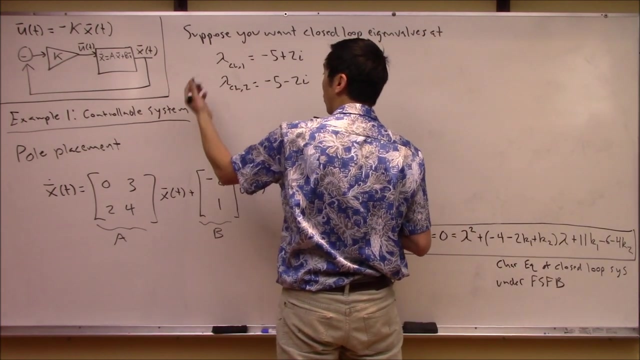 close the loop and do everything. I want it to behave like it's got pole or eigenvalues at these locations, right? Well, okay, If you were going to be able to move this location, what is the characteristic equation that is going to yield these two eigenvalues, right? So the other way? 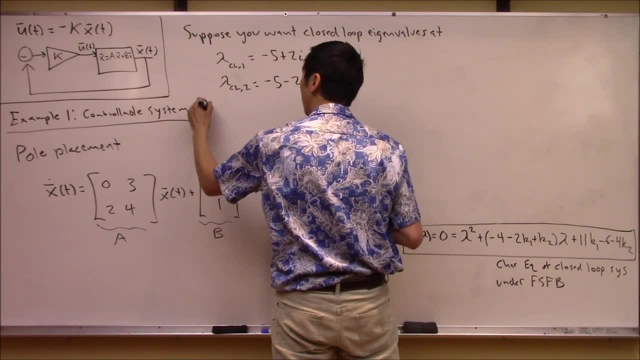 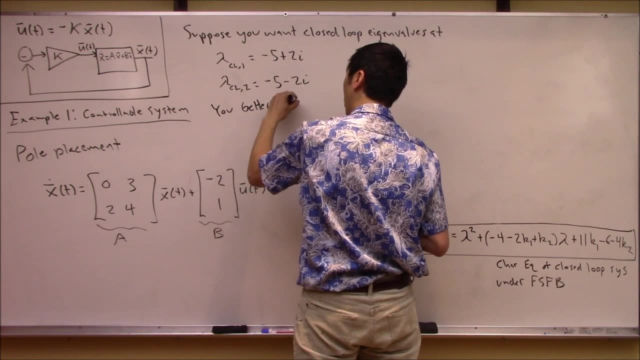 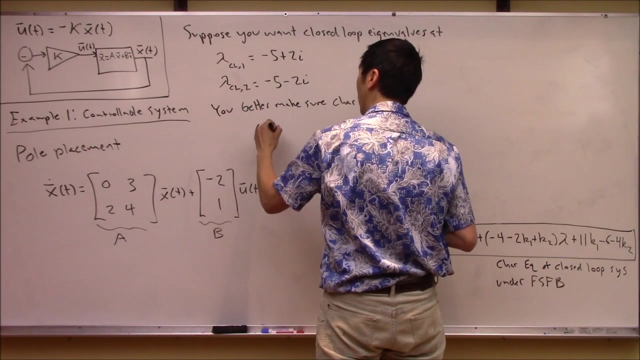 to think about. that is, if you want these eigenvalues to be at a specific location, you want to make sure that the characteristic equation looks like this right. So you better make sure the characteristic equation is well. it better be lambda. what plus five minus two? i right, And 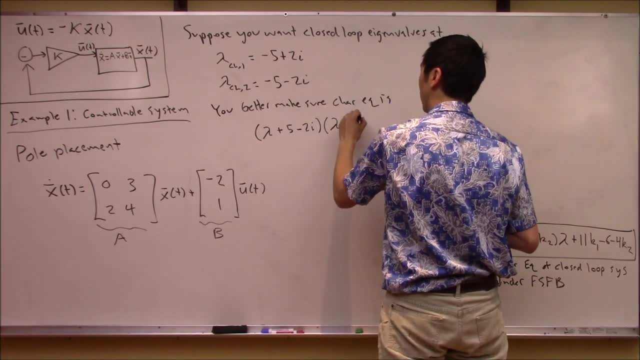 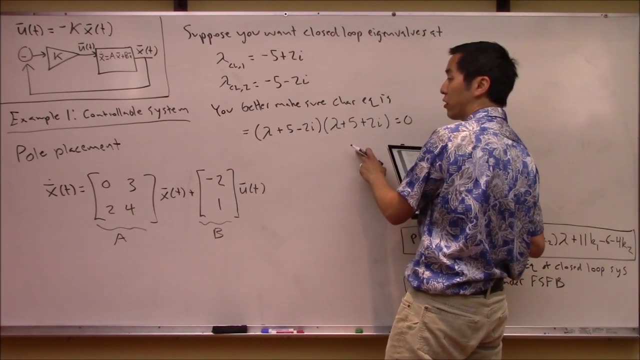 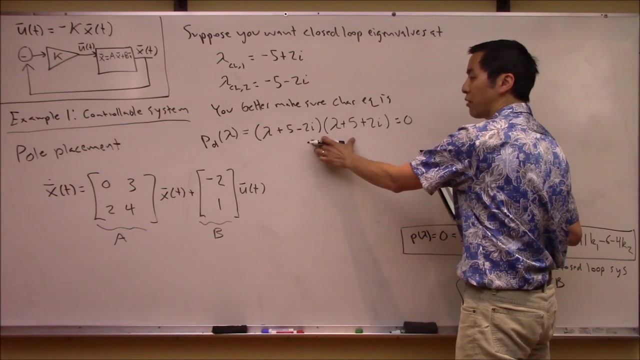 then lambda plus five plus two- i right- is equal to zero, right? This better be the, the characteristic equation, right? Let's call this thing, maybe p desired of lambda, right, You really want the characteristic equation to look like this, because if you do, if you got, if you 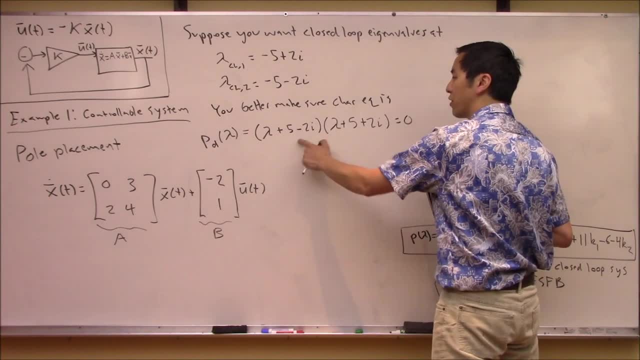 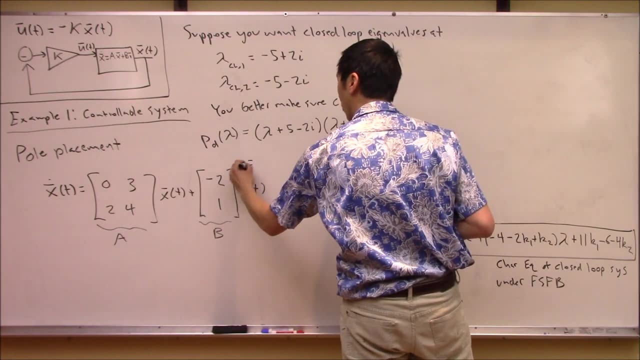 get a characteristic equation to look like this. I can tell you right now: yeah, the roots of this characteristic equation are exactly where you want it to be right. Okay, so tell you what. expand this thing out. So you could also write this thing to look like: uh, it would be lambda. 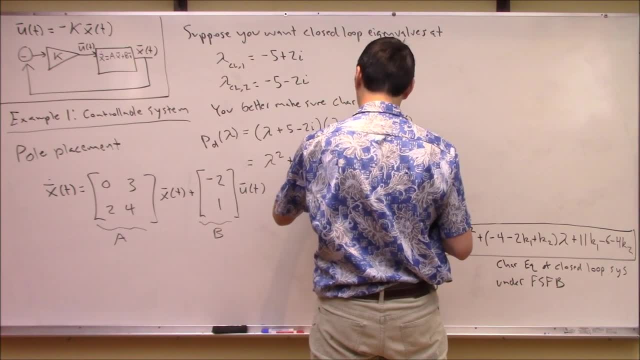 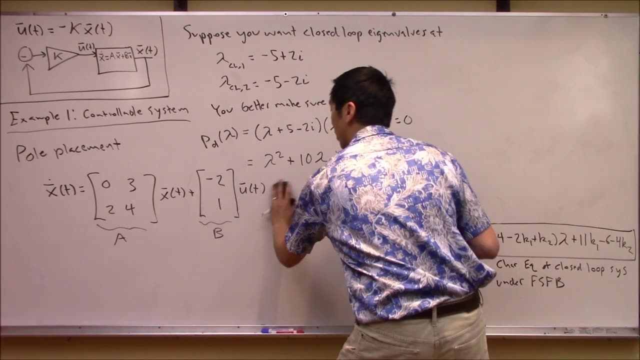 squared plus 10 lambda plus 29.. By the time you just boil this thing out, right, You do the expansion, and I think that's what you would end up with. Okay, so tell you what again. let's erase the junk that we don't care about any longer. 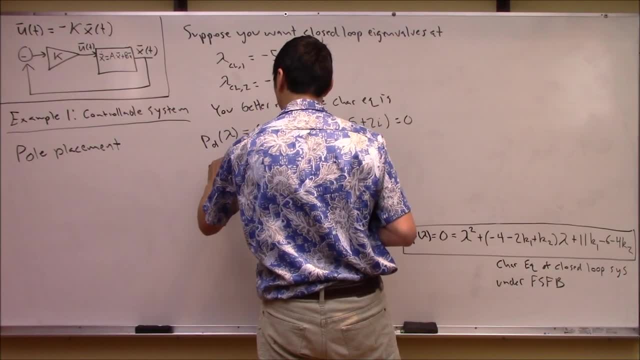 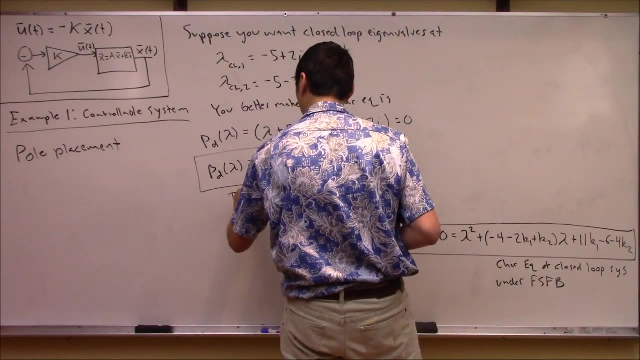 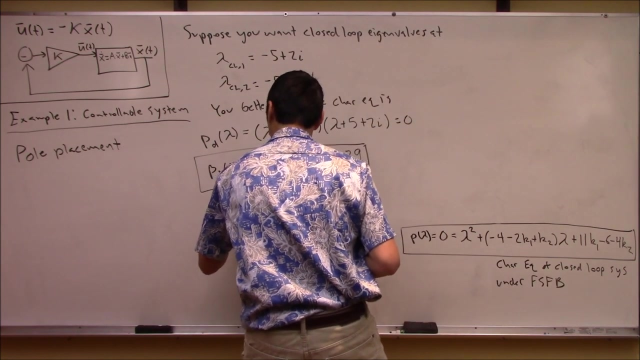 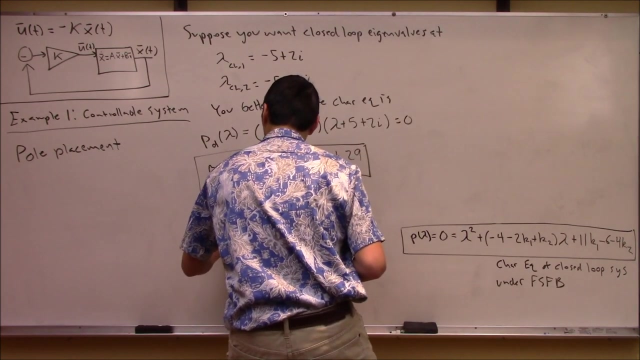 Okay, so here's p desired of lambda right, And let's box this up right And again. let's make a note here that this is the desired characteristic equation in order to place poles, slash eigenvalue right At desired locations. 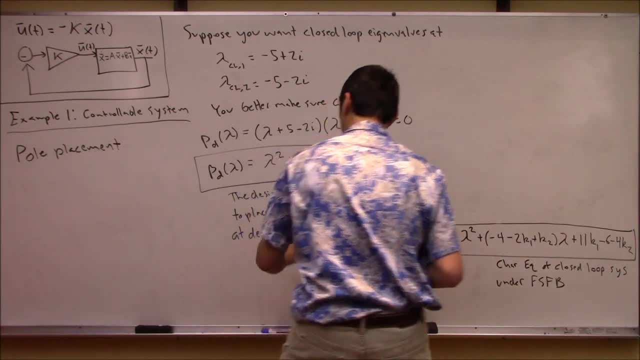 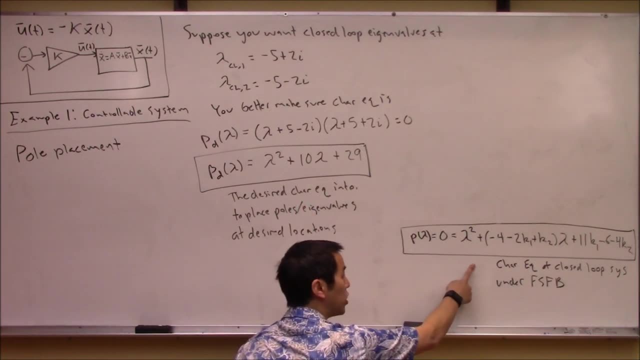 right? Okay, so here's the characteristic equation that we want. Here's the characteristic equation you get under full state feedback control, So I just need to make these two equal to each other, right? So, in other words, all I need to do is: you know what? Compare the. 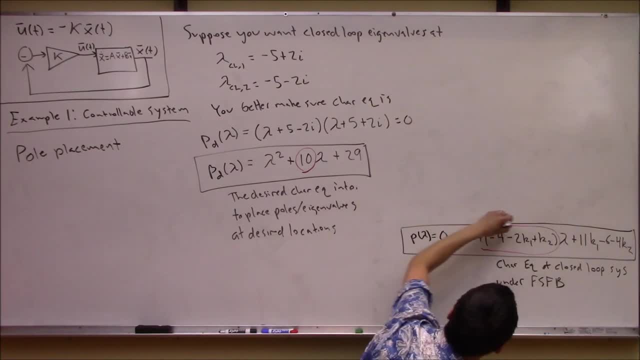 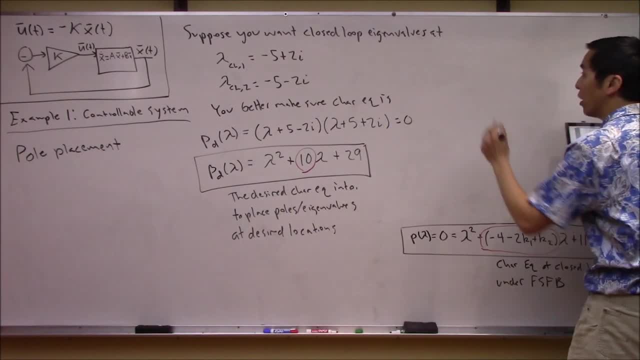 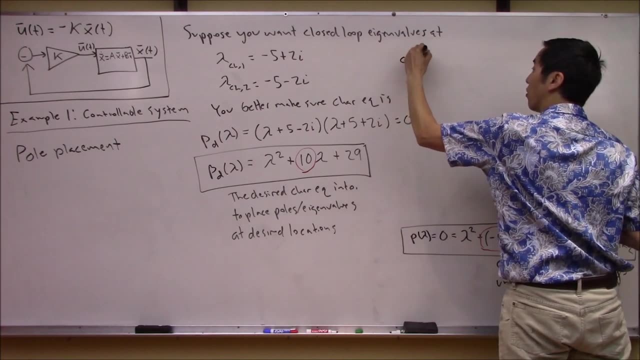 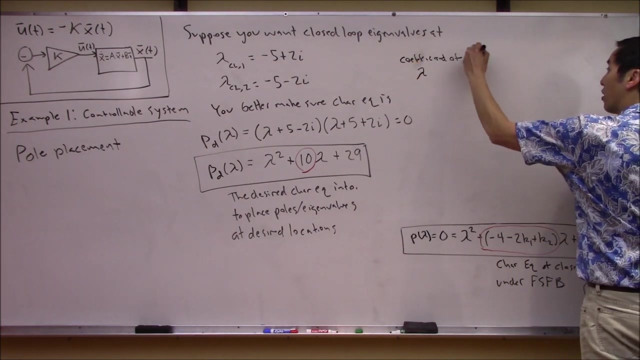 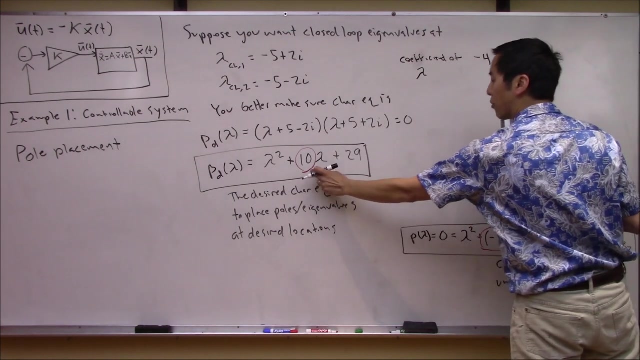 So we get one equation here. So if I compare the coefficient of lambda, maybe I'll just write it like this: We basically get an expression here that, all right, you get minus 4,, minus 2k1, plus k2 had better equal. the coefficient of lambda over here had better equal 10, right. 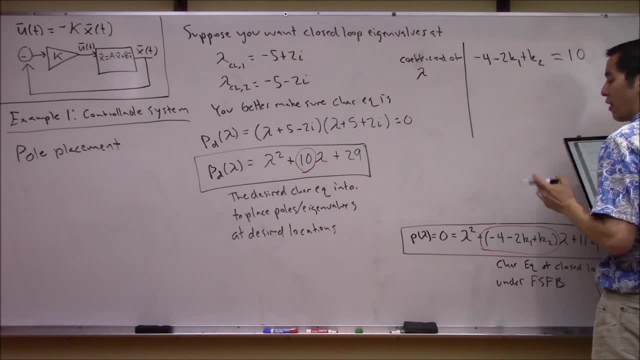 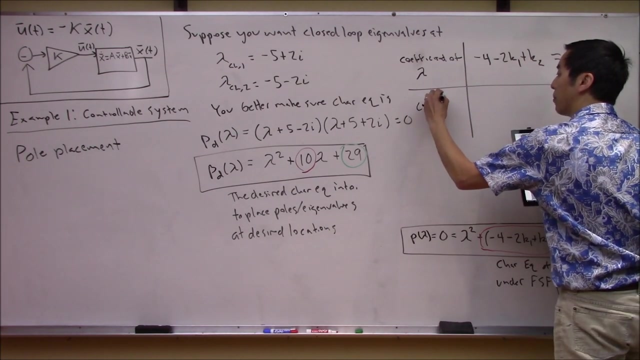 Okay, and then our second equation here is the constant right. Let's do it in another color. The constant of what I want had better equal the constant of what I've got right. So if I look at the constant term right, 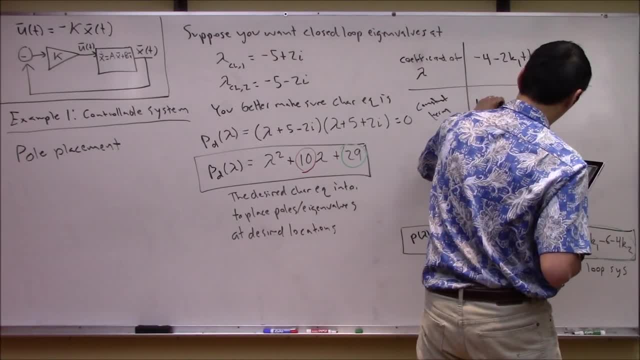 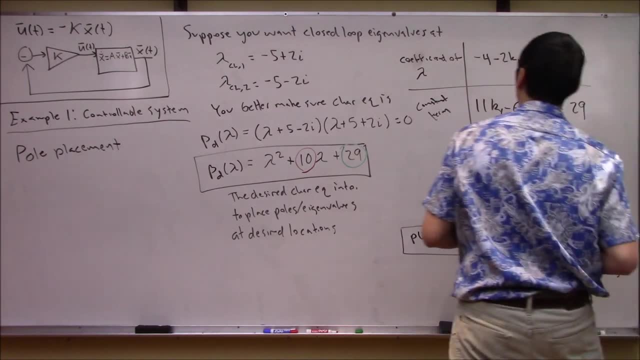 Again, we end up with. what do we end up with? It's 11k1 minus 6 minus 4k2. had better equal the constant here of 29, right, Great. so, if you look at this, all this thing is it's two equations, two unknowns, right? 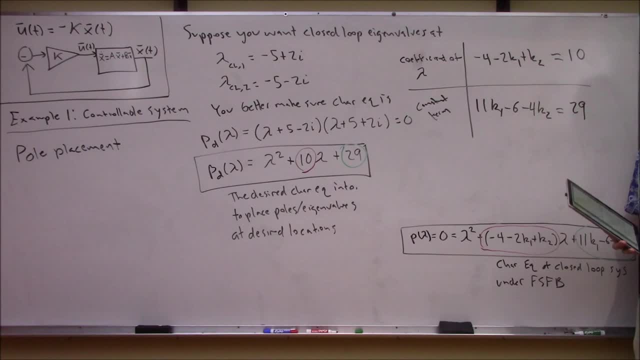 And, in fact, this is even easier. They're two linear equations And, since the system was controllable, you can pretty much guarantee that this is going to be solvable right And, furthermore, there will be- in this case, there's going to be- a unique solution here. 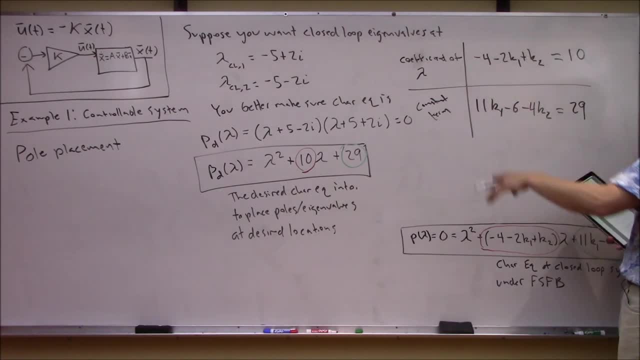 So run to your favorite package right. Go ahead and write this in matrix form and row reduce. Do whatever you want to do to solve two equations for two unknowns, And you'll end up with what do we end up with here? 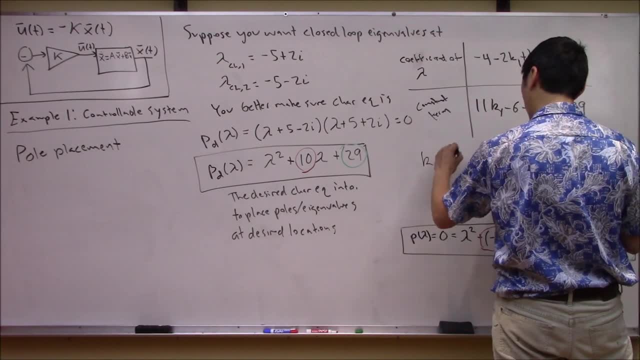 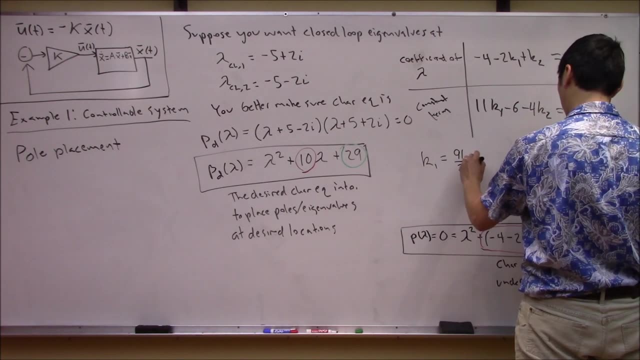 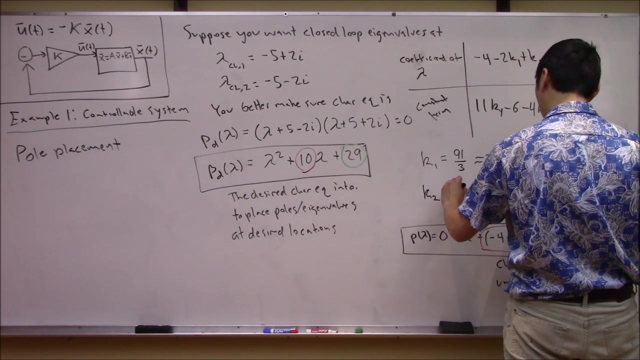 So I think you'll end up with this. You'll end up with: k1 has got to be equal to 91 thirds, which is about 30.33.. And k2 has got to equal 224 over 3, which is, again, this is approximately 74.67.. 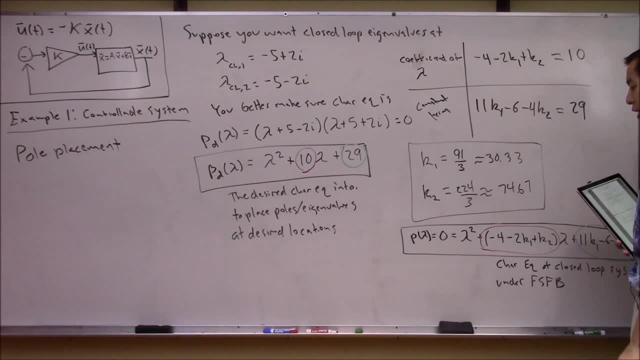 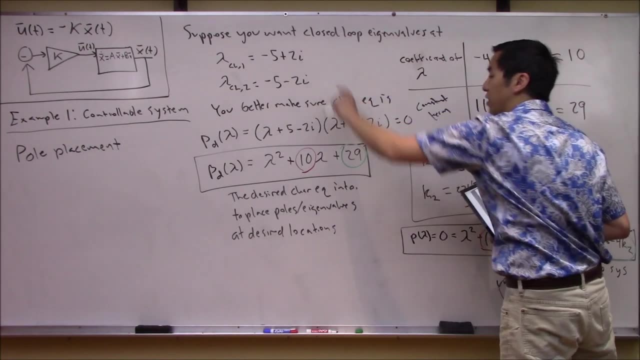 Okay, so here we go. This went ahead. We solved now for the The k matrix that will get us the eigenvalues to be placed in exactly these locations, right, And you saw that it's actually not that bad a procedure, at least in this case, right. 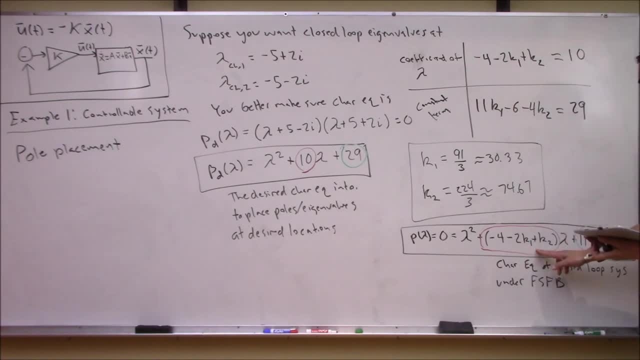 All it's doing here. all you need to do is look at what is the characteristic equation you get under full state feedback control. compare it to the characteristic equation that you want, right, And just make the two of them equal to each other. okay. 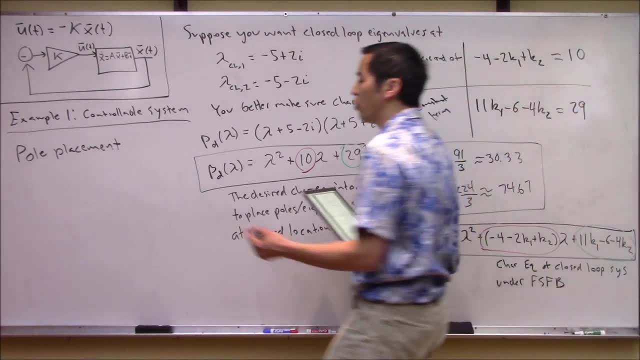 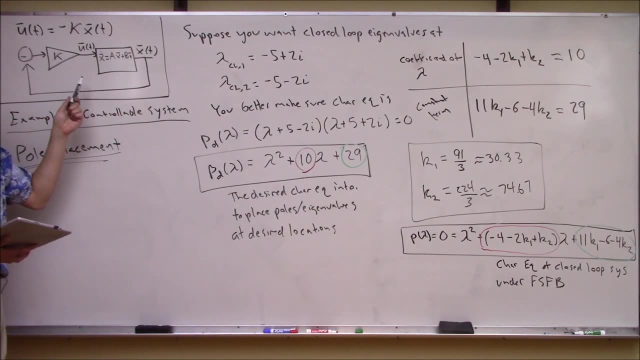 Now to support this workflow again we talked about. this whole workflow is referred to as pole placement, Right, Because that's exactly what we're doing. We're placing the poles of this closed loop system to wherever we want it to be. 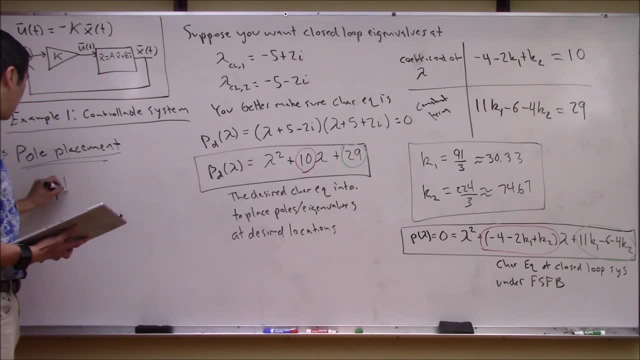 MATLAB's got a nice routine that will allow us to do this, called place. Okay, So I'll tell you what. Let's run over to MATLAB and do this exact example and see if we can just use the place command to automate this process for us. 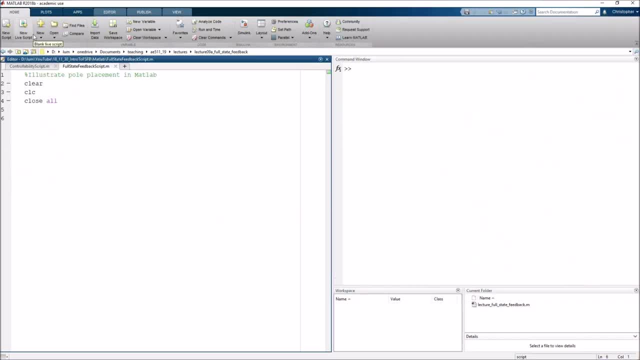 All right. So this is actually really, really simple in MATLAB. So let's go ahead and first define our a matrix- So I think this is what we ended up using- And also let's define our b matrix, And now what we should probably do here is check controllability. 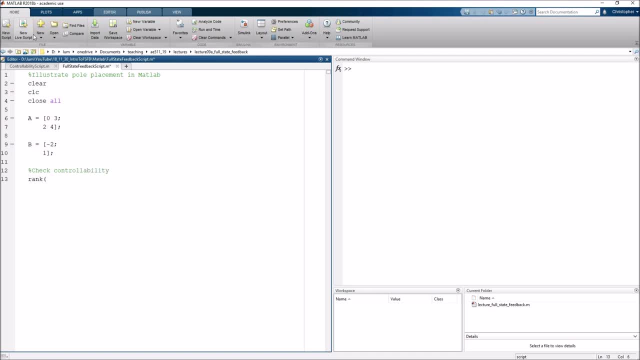 Right, We talked about how that is a critical component. So let's check the rank of the controllability matrix And again, if you would like a refresher on rank or CTRB, please go ahead and check out our controllability lecture. 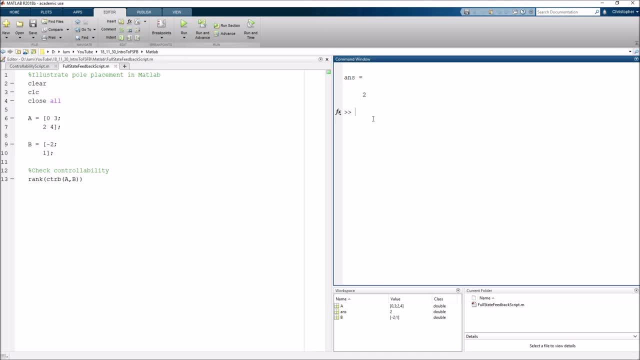 So let's go ahead and run this And we see: yep, full rank. So this system should be controllable. So what I can do now is I would like to perform pull placement. Okay, So to do that, like we said, MATLAB has this nice command called place. 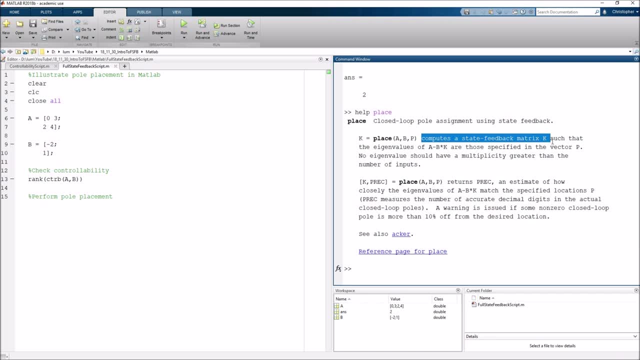 And place will, as it says, compute the feedback matrix K to put the eigenvalues of the closed loop system where we want. So what I need to do here is make a- Let's call it p- desired Right. This is the location of where I want to put the pulls. 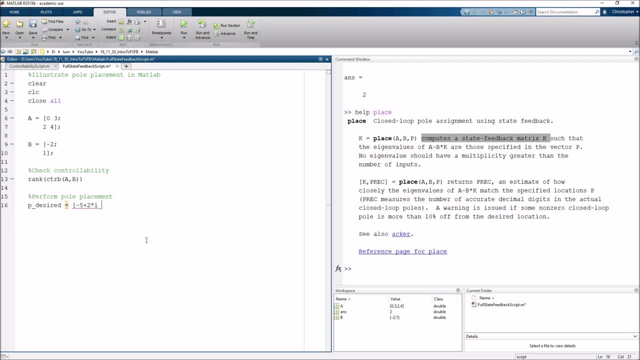 And I think we said it was minus 5 plus 2i and minus 5 minus 2i. Right, That's the locations where I want to put the pulls. So now it's really, really simple. I go ahead and say place A, whoops A, B and then p- desired. 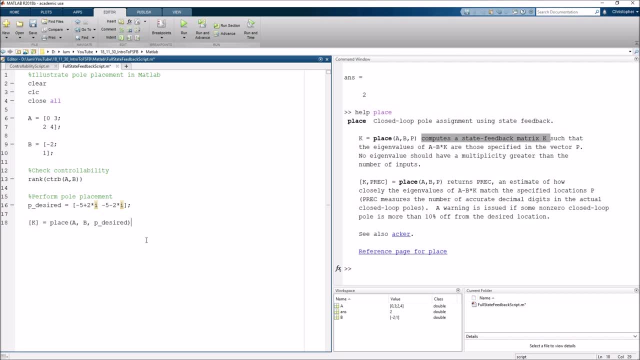 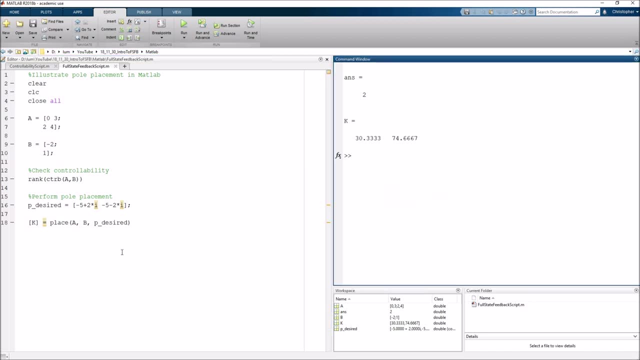 Right, And what this will return for me is the matrix K that should place the pulls at that location. So if I run this, here we go. These are the gains that we computed on the board, And maybe what we should just do. one last double check before we leave MATLAB is check that the closed loop eigenvalues. 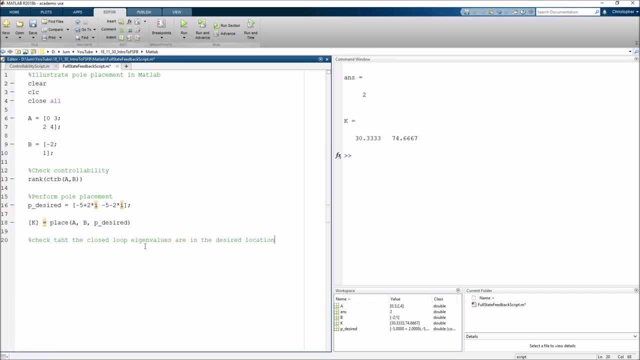 Right, Are in the desired location Right. So to do that, all we need to do is: First let's make A closed loop Right- I think we said that was A minus B times K, Right? And then let's just look at the eigenvalues of the closed loop system. 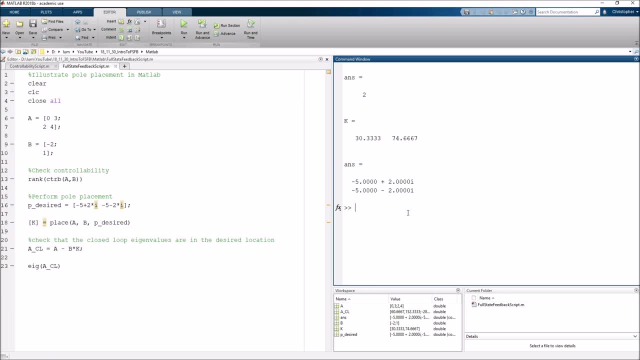 So if I run this, yay, look at that, That is exactly where we want it to go. Okay, before we leave this, maybe what I will mention is there's actually another command you could also use in MATLAB, Besides the place command. 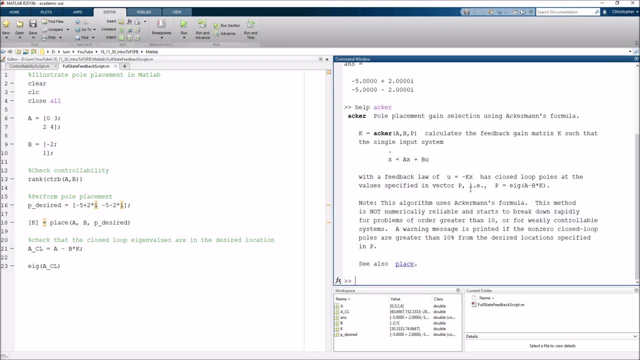 And that is ACKER A-C-K-E-R. So this is using Ackerman's formula to do a similar operation. So, for example, we could come up here and, instead of calling place, Let's go ahead and I will copy this and let's paste it below. 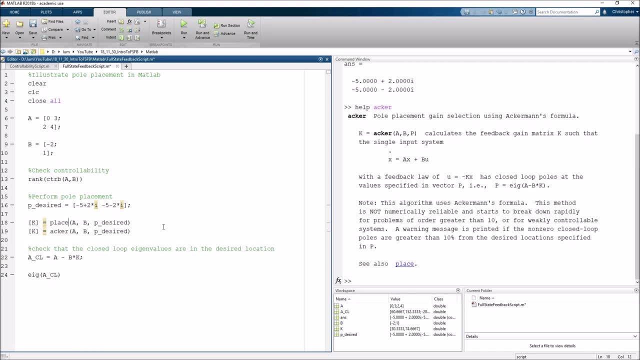 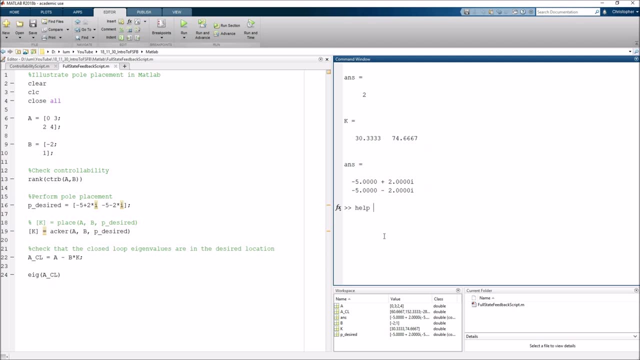 You could also call ACKER, which should hopefully get you similar results. Okay, So if we run this again, yep, we get the exact same results. Just a quick note here. I think if you read the help on ACKER, it says that it's not reliable for larger order systems. 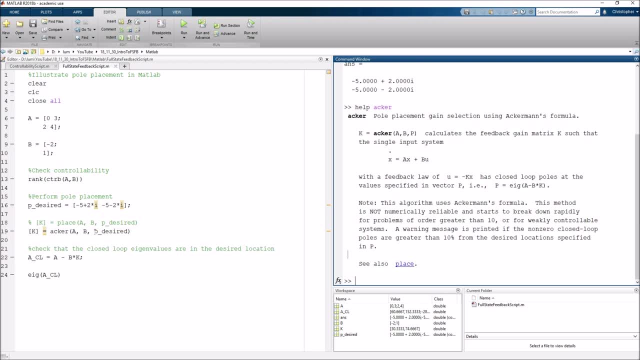 So place might be a better way to go. But again, I just wanted to point out that there's more than one way to ride this donkey. You can either use place or you could use ACKER. Okay, so this worked quite well for a controllable system. 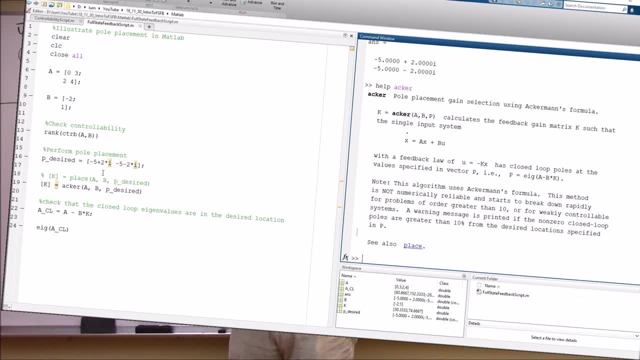 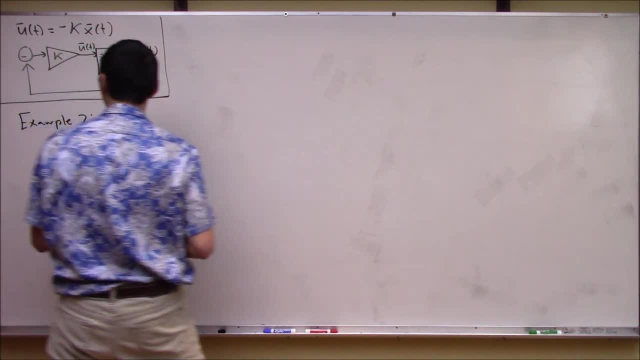 Let's jump back to the whiteboard and look at a system that maybe is uncontrollable. All right, so let's look at another example, because I bet you're just dying to know: Does this, Does this? What happens if you have a system that's uncontrollable? 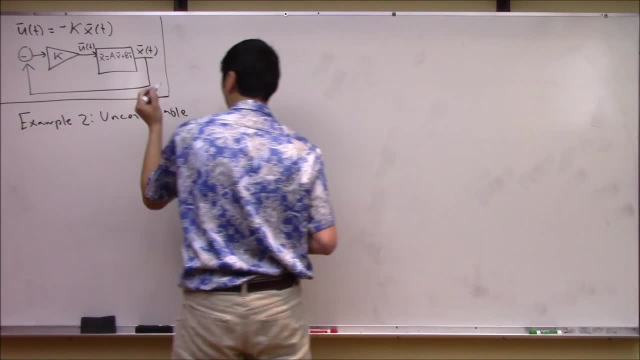 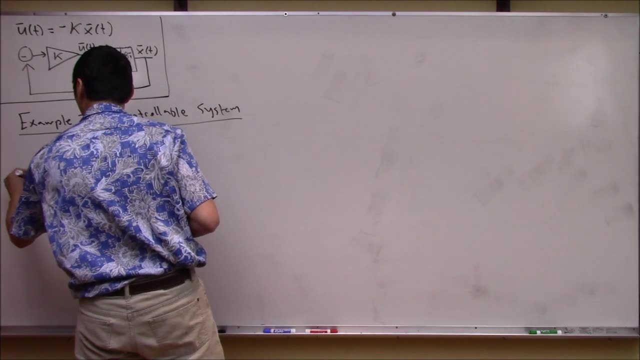 Does it still work? And the answer is actually no, But let's go ahead and walk through this, just to show where this breaks down. So let's consider a very similar system. Right, We'll keep the exact same A matrix we had earlier. 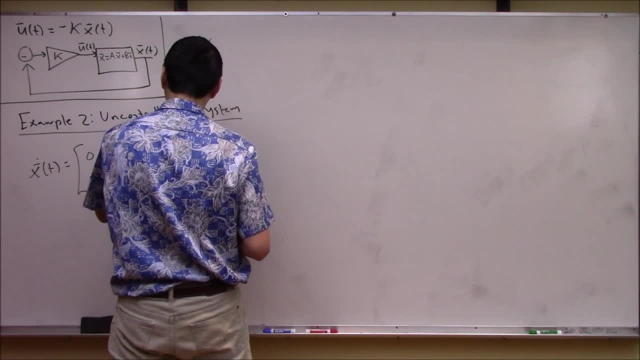 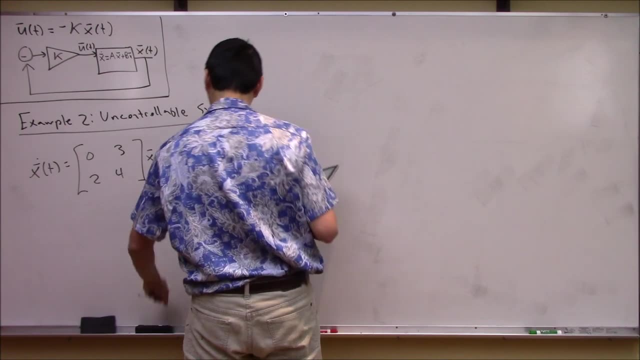 But now what I'm going to do is let's choose a B matrix that is uncontrollable here. So this B matrix is going to be: Oh gosh, I need a little. I need a little bit more room actually, because it's actually a little bit involved here. 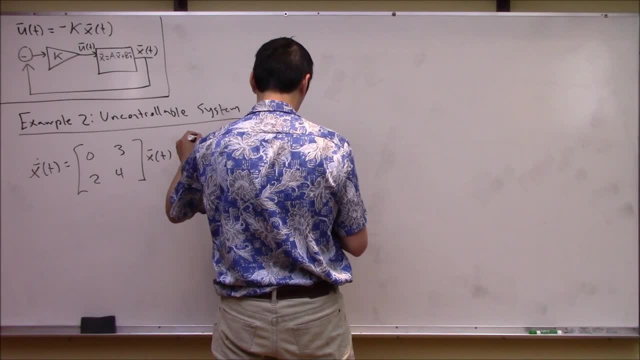 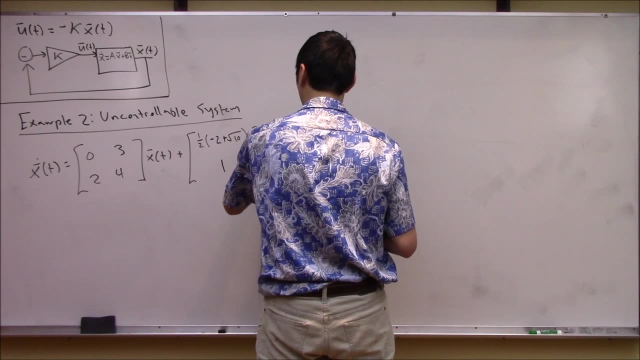 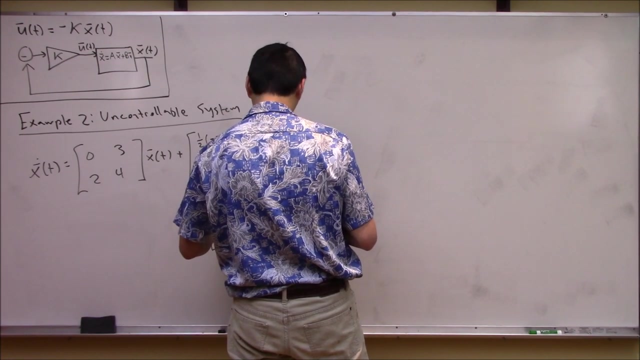 It's still a 2 by 1 here, but this is now 1 half times negative 2 plus square root 10.. And then 1.. U Okay, This I think. if you wanted to write it out numerically, I think this comes out to about 0.5811, and then a 1.. 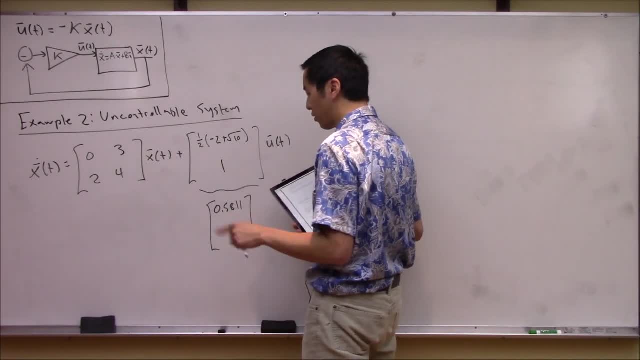 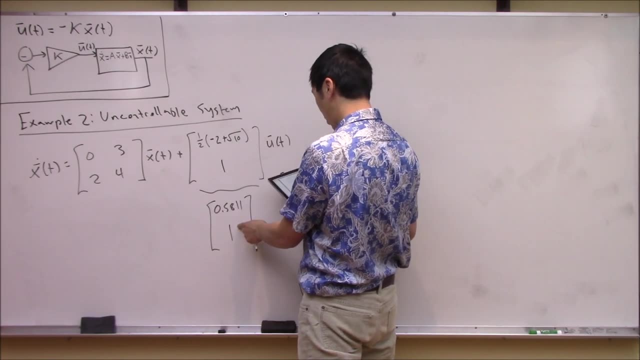 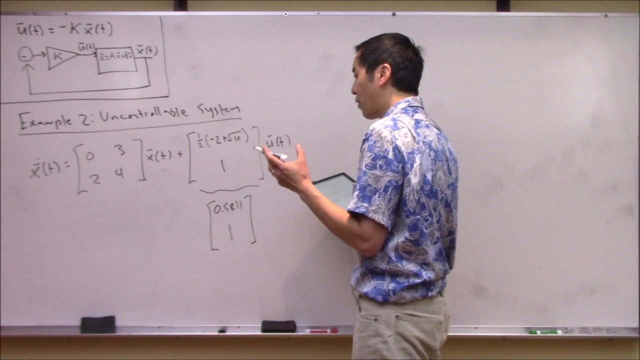 Okay, Interestingly, I guess as a little side note for those of you who have watched the controllability Lecturer, this is actually an eigenvector right corresponding to one of the eigenvalues, And I think we showed last time that if you have a 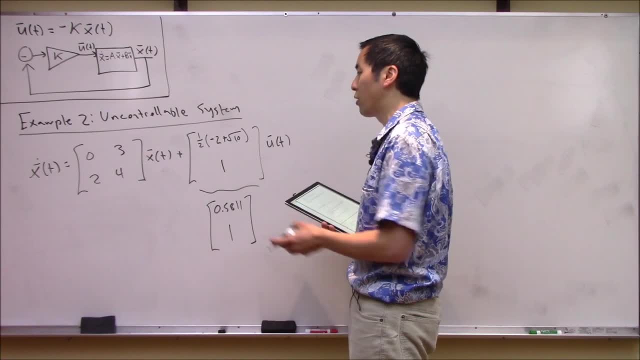 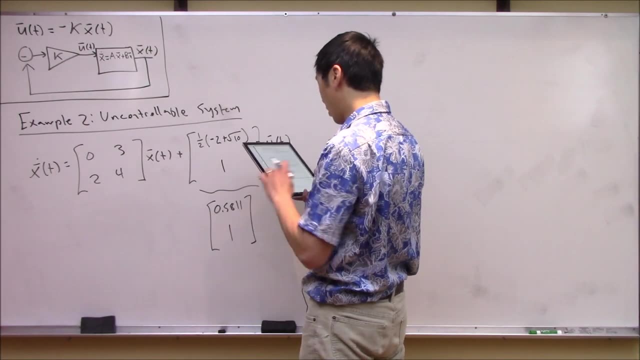 Basically, if your B matrix is exactly an eigenvector, right, you end up with an uncontrollable system. So this system we claim is uncontrollable. We'll check the controllability in a second. Actually, you know what? 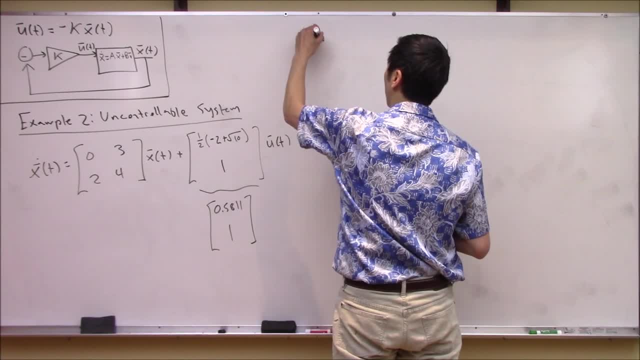 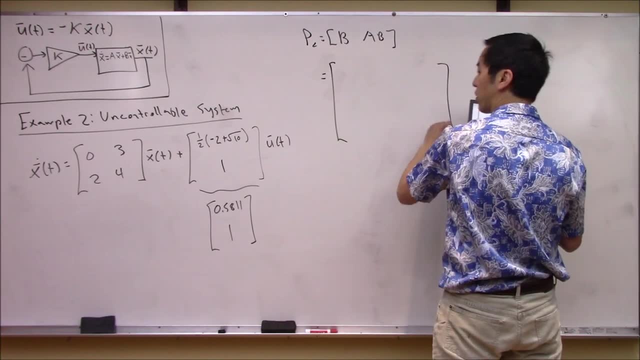 Maybe we should do this right now. So again, let's check controllability PC. here You do the exact same thing: B, A, B, Right, And what you end up with here is you end up with: Okay, the B matrix again is pretty simple. 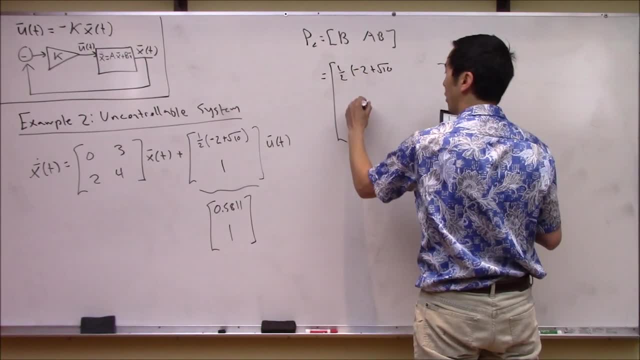 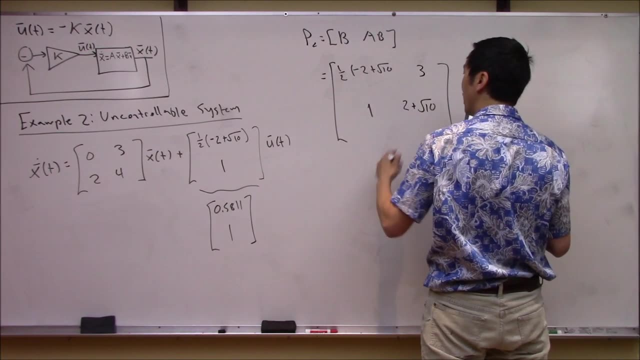 It's 1 half negative, 2 plus root 10, and then 1.. And then A times B. when you do that multiplication I think you get 3, and then 2 plus root 10.. Okay, And you check the rank of this thing and it's only 1.. 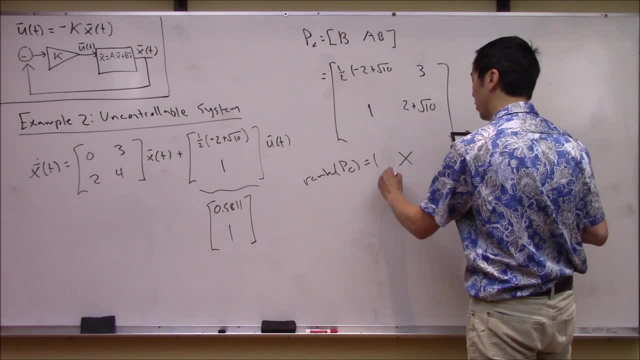 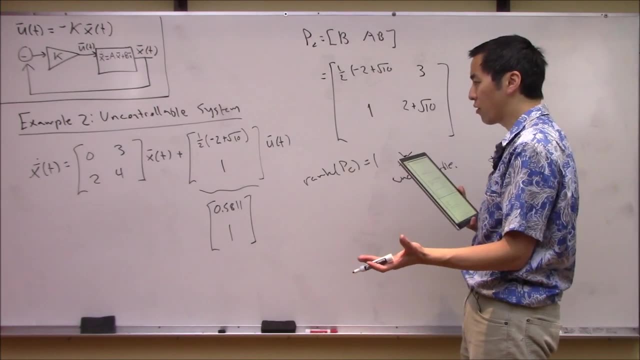 Right, So it's rank deficient, so the system is uncontrollable. Okay, So you can do the exact same operations we did earlier And let's see where this is going to degrade and break down. So you perform the same pole placement. 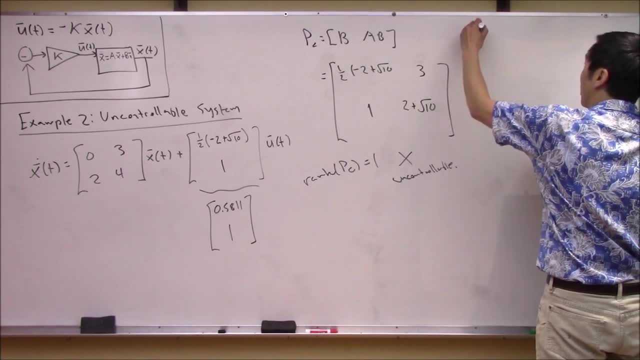 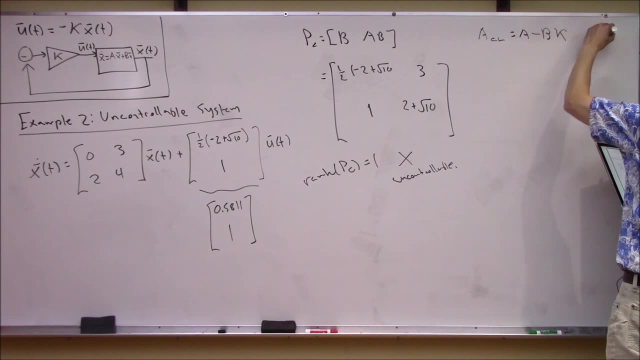 So, if you remember, all we did last time was we computed A, C, L Right As being A minus B, K Right, And we know here that K is again a K1 and a K2. Right. 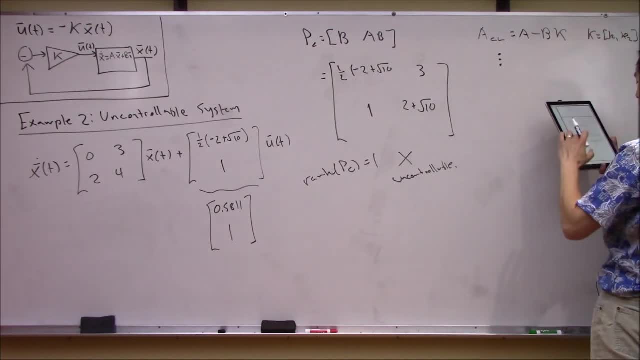 It's just a 1 by 2 matrix. So you do that math Right And let me see Is it ugly or not. I have it here in the notes. I guess it's not horribly ugly. Tell you what. 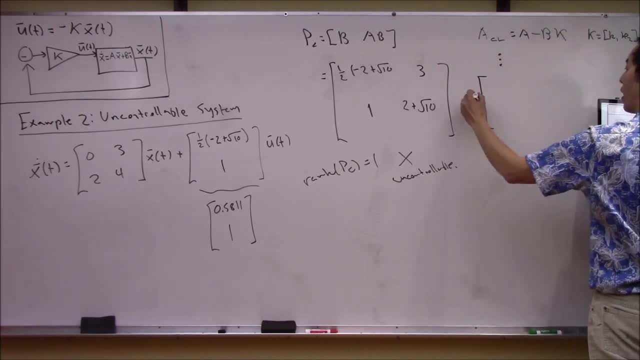 Let's, I'll just write it out for you. I'll just write it out for completeness, just so everyone can follow along here. So A closed loop. what you would end up with still a 2 by 2 here. 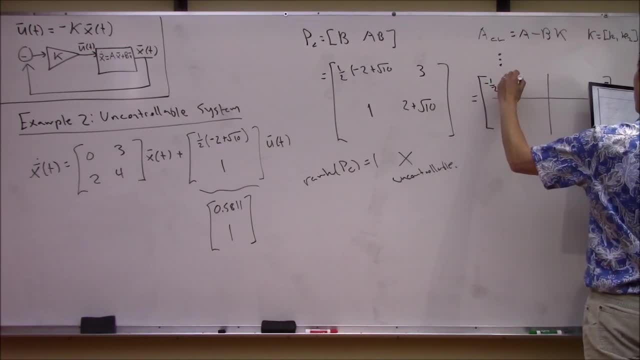 So this is going to be minus 1 half times negative, 2 plus root, 10 times K1. And then you'd end up with 2 minus K1. And then in this entry up here, you get 3 minus a half times negative, 2 plus root, 10 times K2.. 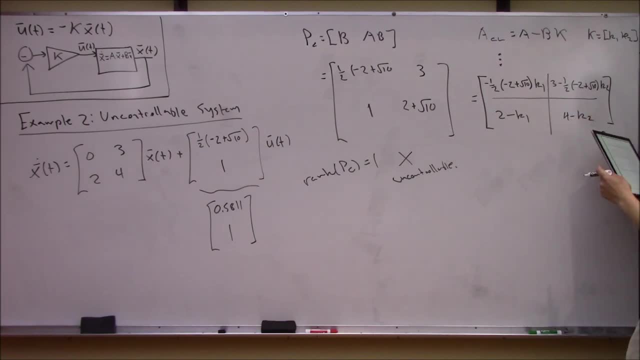 And then you'd end up with 4 minus K2.. Okay, Okay, Let's close the loop. Now what we would do is we would compute the characteristic equation for this system here. Right, I'd go ahead and do: determinant of lambda, I minus A closed loop is equal to 0.. 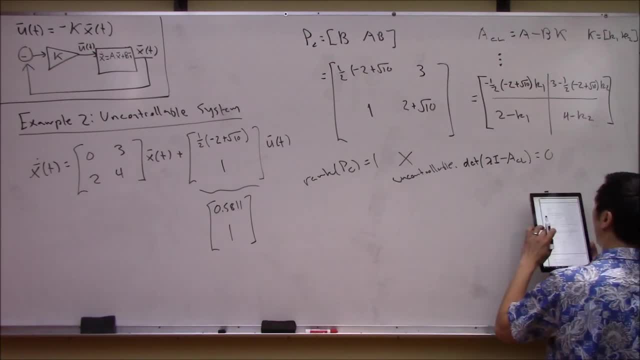 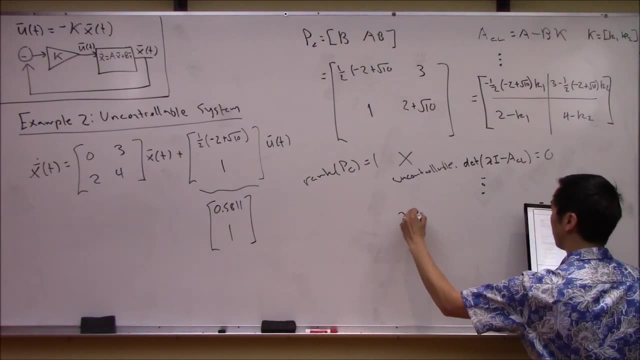 Okay, So again, that is something ugly. But basically what you can do is, after a bunch of algebraic manipulation you can get this thing to look like lambda squared plus this quantity here. So it's minus 4 plus. 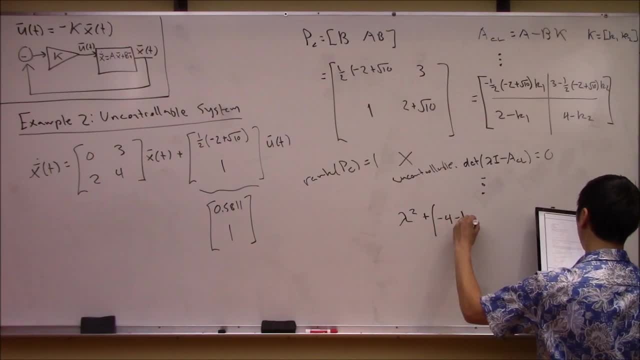 Whoops, that's a minus Minus K1 plus root 5 over 2, K1 plus K2.. This is times lambda plus Gosh. a constant. I ran out of room, So the constant. So it's a second order polynomial. 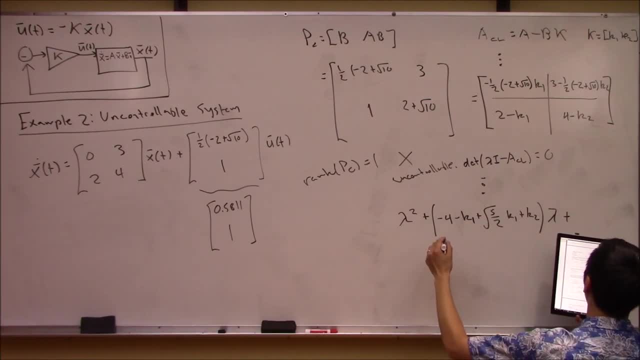 So the constant here, or the zeroth order, this is what Minus 6 plus 7 K1, minus 2 root 10 K1, minus 2 K2 plus Root 10 K2.. Again, something Right. 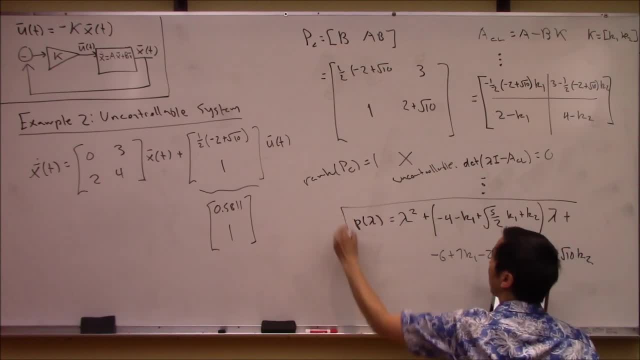 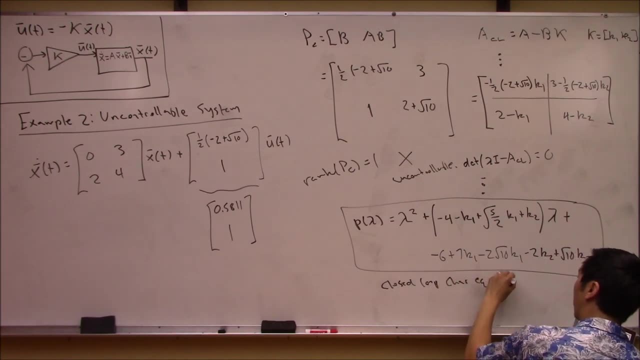 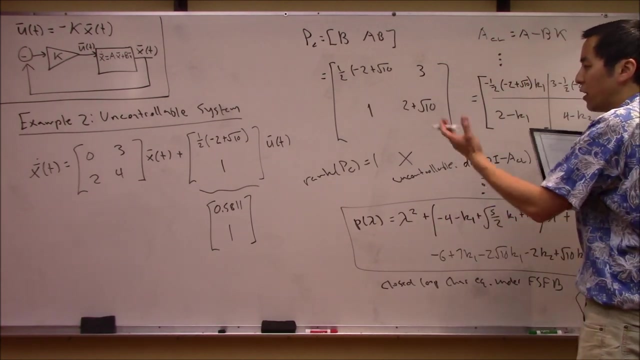 This here is P of lambda here, Right? So again, this is the closed loop characteristic equation under full state feedback, Right, And now we need to just compare with what we want. So let's use the exact same poles that we wanted to earlier. 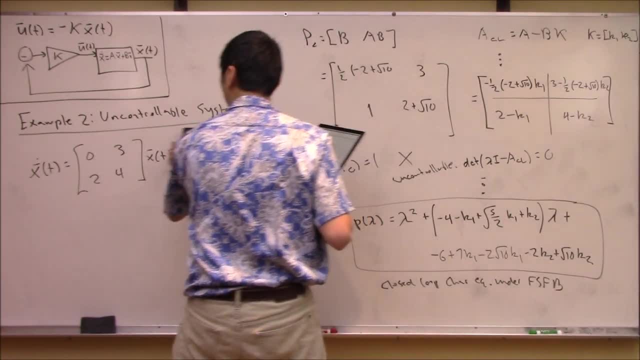 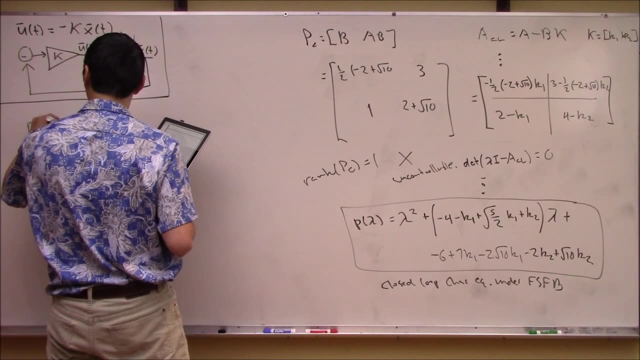 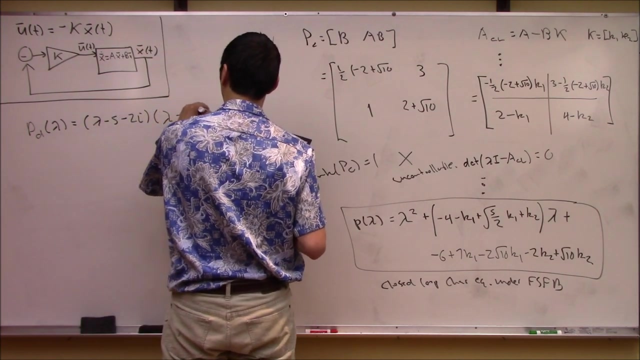 That we considered earlier. So let's just say I want to place this system At P desired of lambda at lambda minus 5 minus 2I. lambda minus 5 plus 2I. Right, So I have poles at. 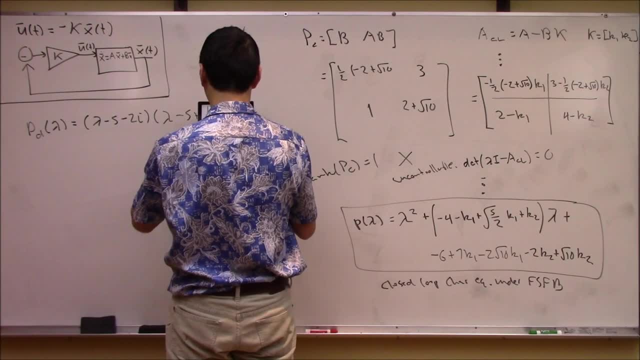 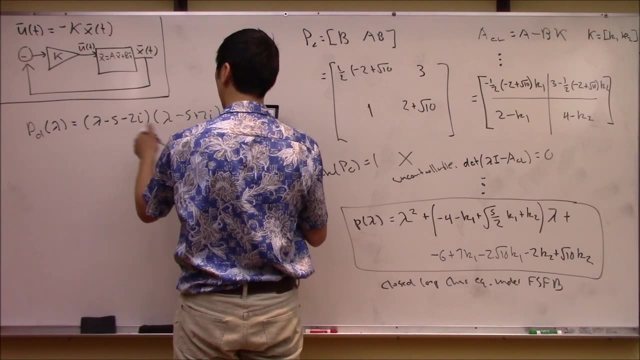 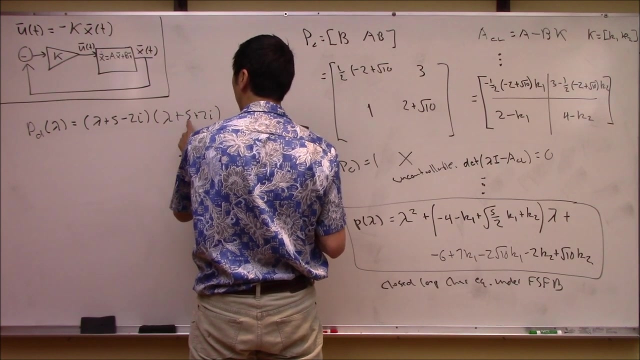 Wait a second. What did it do? Hold on, Is that a plus? I think it's a plus. Didn't we want the poles at positive? I have to make sure, Did I mess this up in the last one? We wanted the poles at. lambda is equal to minus 5 plus or minus 2I. 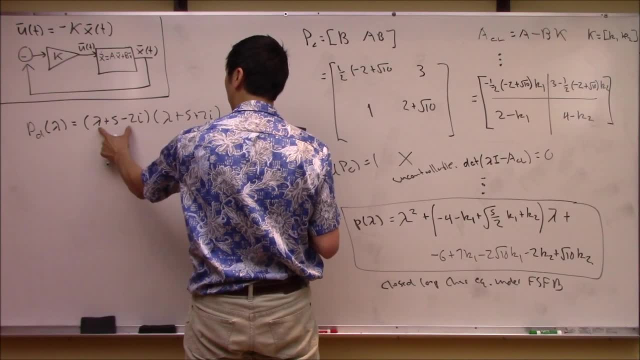 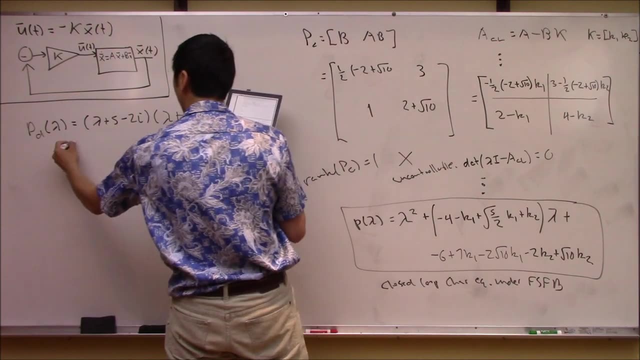 So it's got to look like this. So I'll have to double check the video to see: Did I drop this plus sign in the earlier one? If I did, I'll correct it. Okay, Anyway, Again, this is the exact same characteristic equation we were considering earlier. 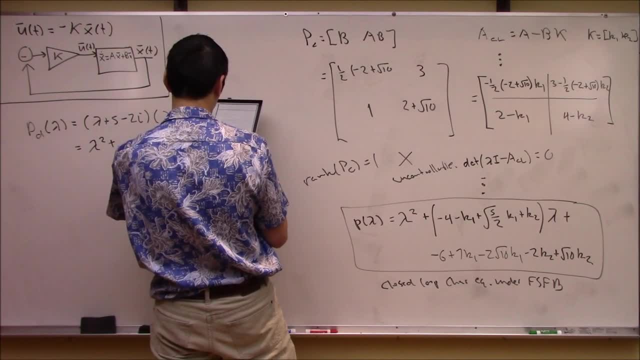 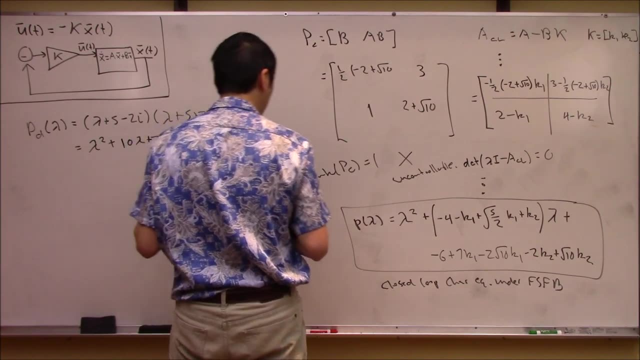 Right, So that is, If you expand it out, it's lambda squared. Come on, Where did I put this thing here? Oh yeah, Plus 10 lambda, plus 29.. Right, So again you do the exact same thing. 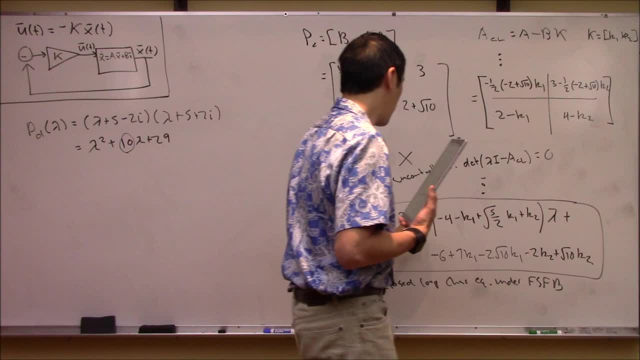 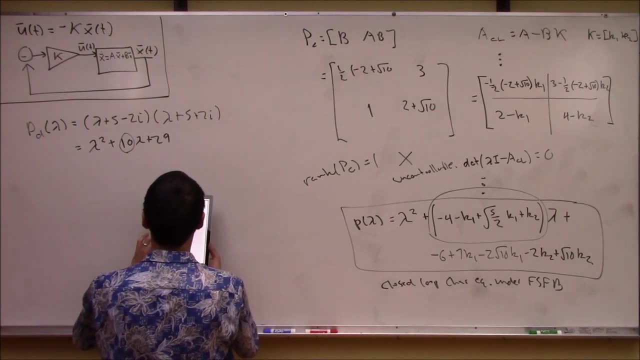 You compare the coefficient of S or the coefficient of lambda with the coefficient of lambda here. Right, Okay, So what we would end up with is: So, that's two equations and two unknowns. So we end up with minus 4, minus k1, plus square root of 5 over 2k1 plus k2 has got to equal 10.. 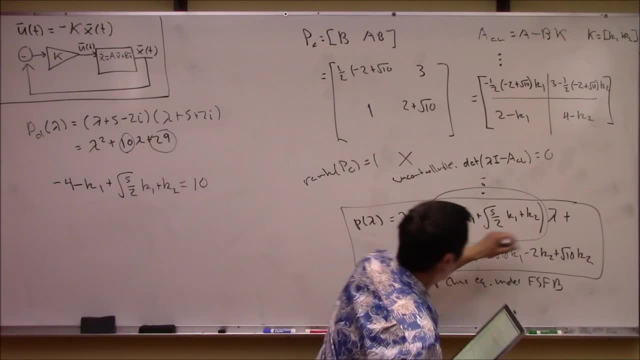 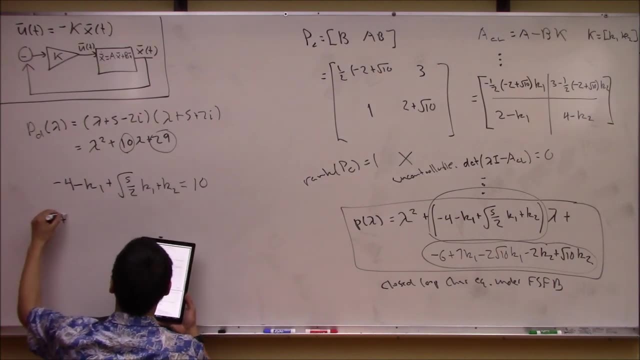 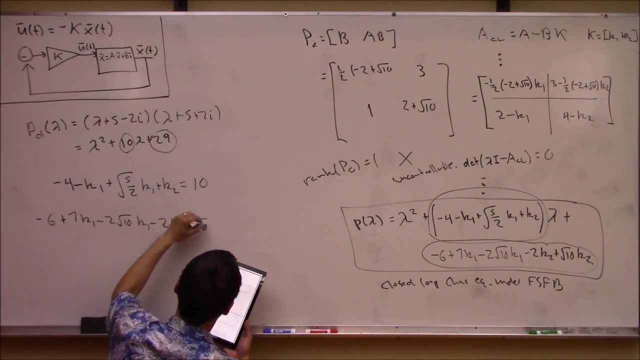 Right. And then we're going to compare the constant here, or the zeroth term, with this term, Right? So then we end up. So then we end up with minus 6 plus 7k1, minus 2 root 10k1 minus 2k2 plus root 10k2 has got to equal to 29.. 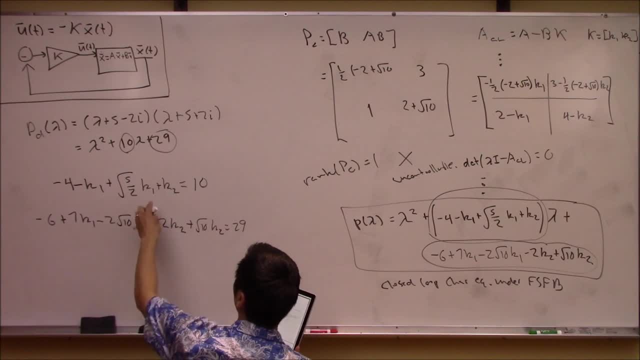 Right, Okay, So now we just need to solve these two equations for these two unknowns, k1 and k2.. And it might be easier if we write this in matrix form, Right? So I think if you want to write this in matrix form, you could write: 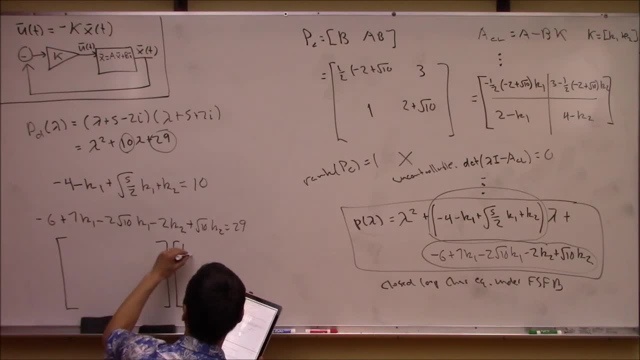 Let's pull this out. So you got this, We got k1, k2.. And actually you can see there's actually this constant over here. There's a minus 4 and then a minus 6 here. Right Has got to equal 10 and 29.. 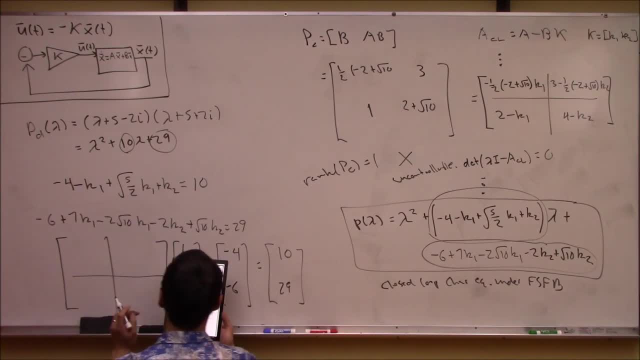 Right, And then this entry right over here. I think if you had gone ahead and done this, you would end up with root 5 over 2 minus 1,, 1, 7 minus 2, root 10, root 10 minus 2.. 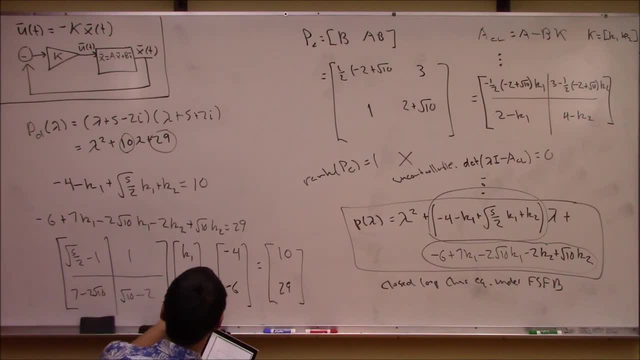 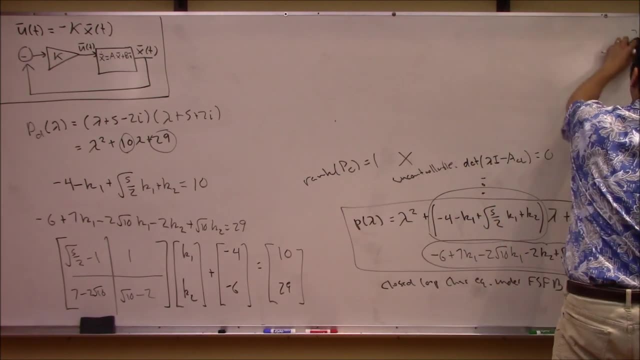 Right, Okay, So let's move this to the other side so we can get this to look like an ax. So what you would end up with then is you'd end up with a matrix expression that looks something like: Okay. 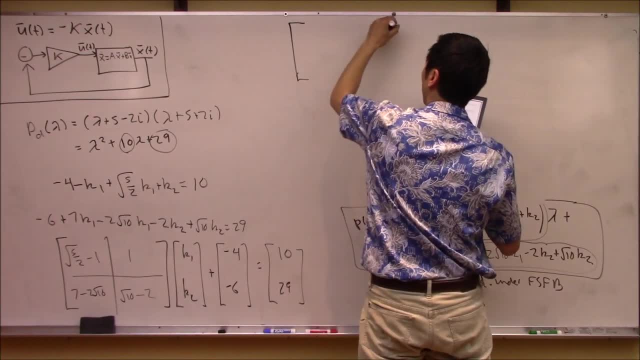 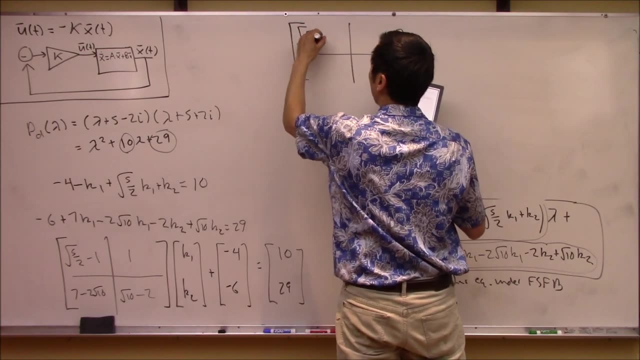 Whoops, That's probably a little bit big. We don't need it that big, Okay. So this, this, So this is the same thing. Root 5 over 2 minus 1, 1, 7 minus 2 root 10.. 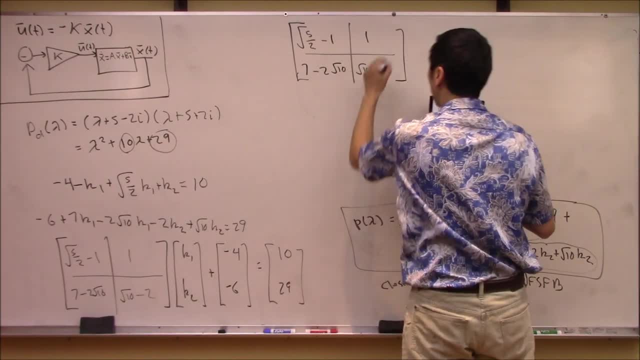 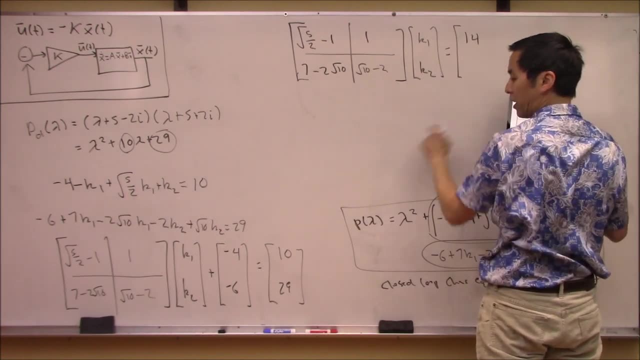 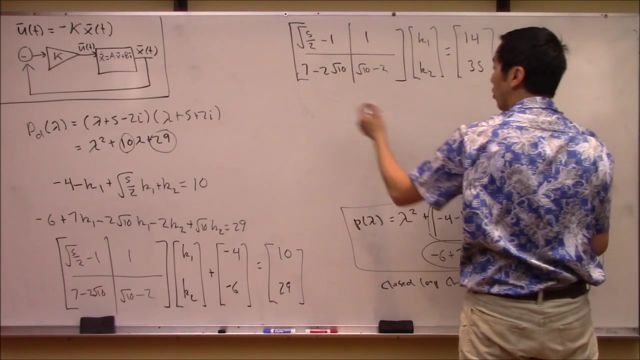 Okay, Root 10 minus 2 times k1, k2 is equal to what is that? 14 and then 35. Right, Okay, So now this looks like a big ax is equal to b problem, Right. 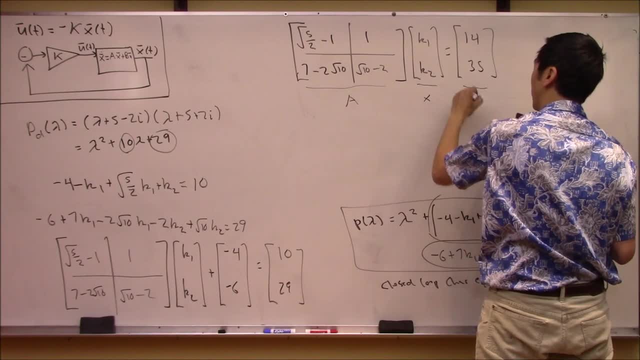 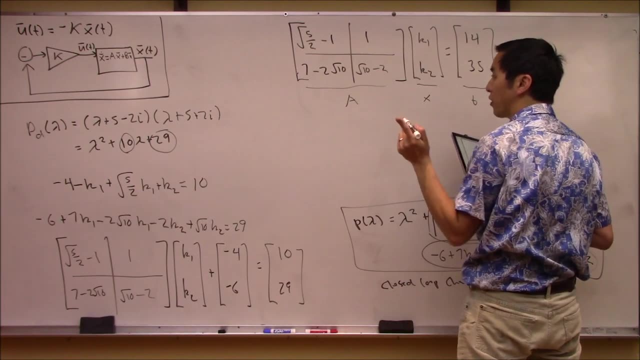 So here's your a, here's your x and here's your b. Right, This looks like ax is equal to b, But if you solve for or if you try to compute the rank of a, you find that it's. 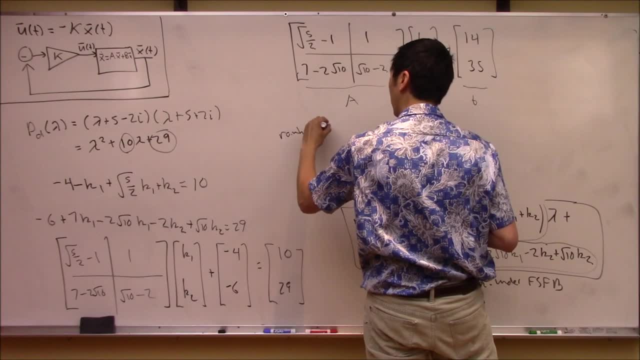 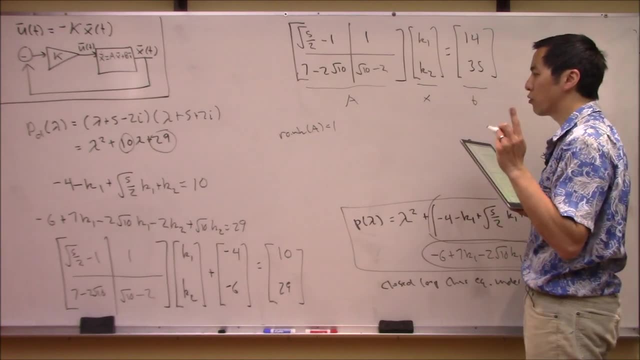 only rank 1 here. So you see that rank of a is equal to 1.. So the inverse doesn't exist. So now we're into one of two situations: There's either infinite solutions or there's no solutions. 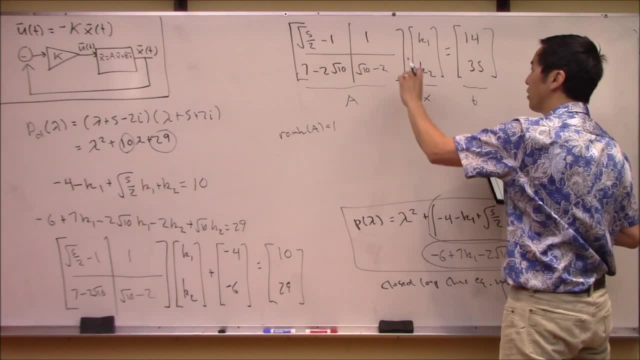 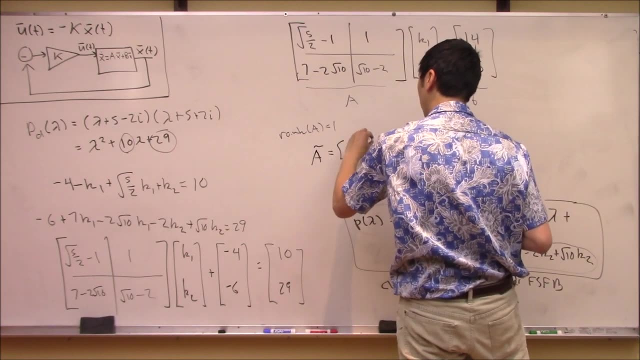 So the way we can figure that out here is: let's create our augmented matrix by putting the b matrix over here. So I'm going to consider our augmented matrix a tilde to be a, b Right, And then I'm going to row reduce that thing. 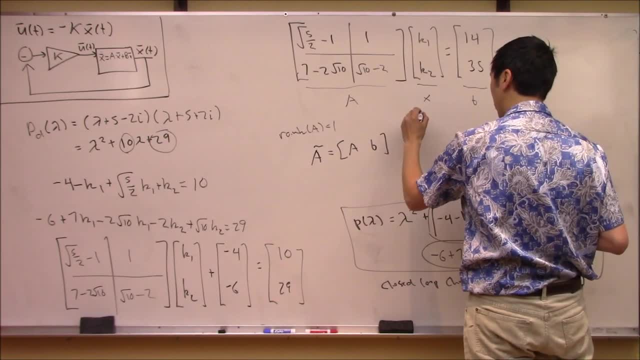 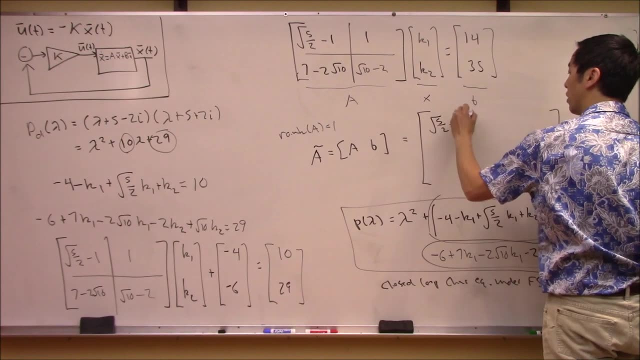 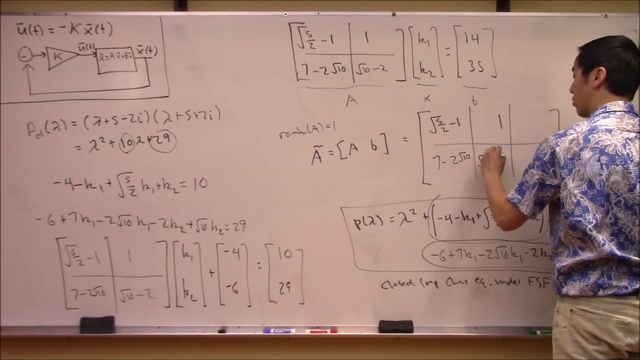 So, again, all that entails is, maybe let's just do one more step to make sure we're all all on the same page, Right? So I'm just going to augment this thing: Rout 5 over 2 minus 1, 1, 7 minus 2, root 10, and then root 10 minus 2.. 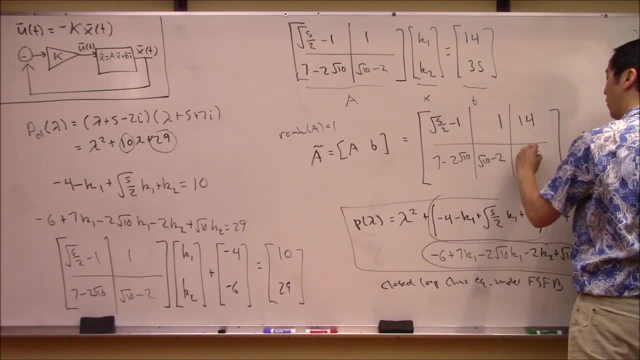 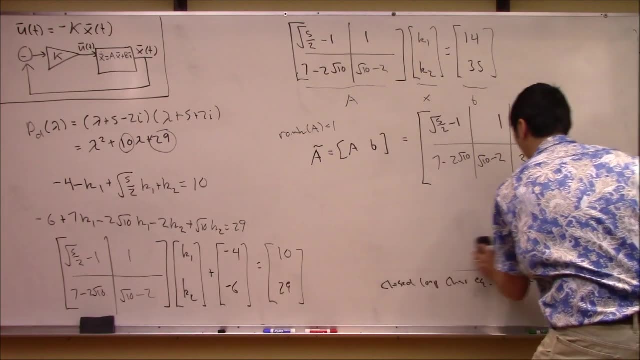 So here's the a, and then I'm going to augment this with the b vector on this side. Okay, So here's my a tilde. This is the augmented matrix, And what I can now do is run over to any mathematical package or, if you want to do the elementary. 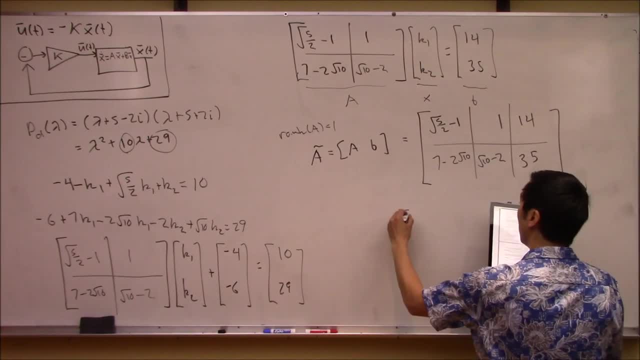 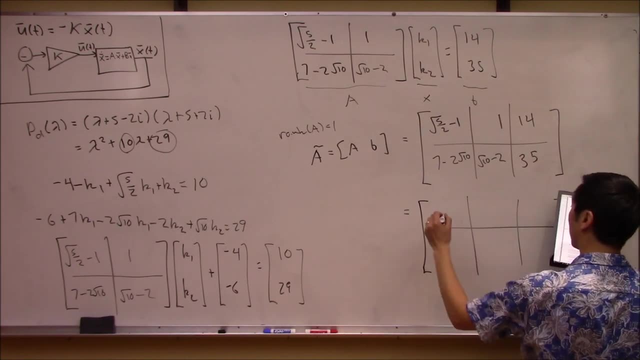 row operations yourself and row reduce. this thing you're free to, But you know, I did this in Mathematica And what I ended up with was this came out looking like 1, 2 over negative 2 plus root, 10, 0, and then 0, 0, 1.. 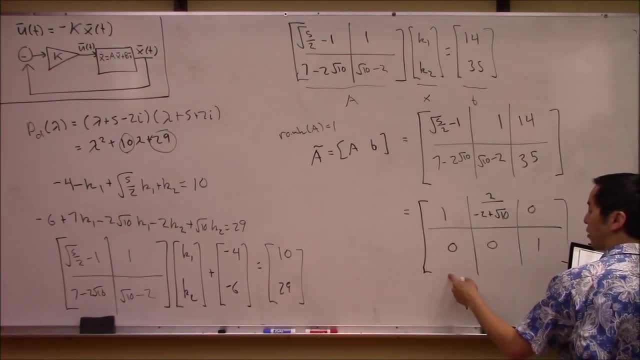 Right. So clearly this is inconsistent. Right, Because if you look at this bottom line, this bottom line basically reads: k1, or basically it reads: 0 is equal to 1.. Right, It's: 0 times k1 plus 0 times k2 is equal to 1.. 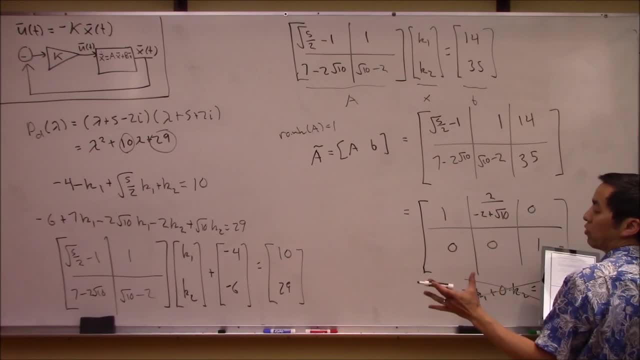 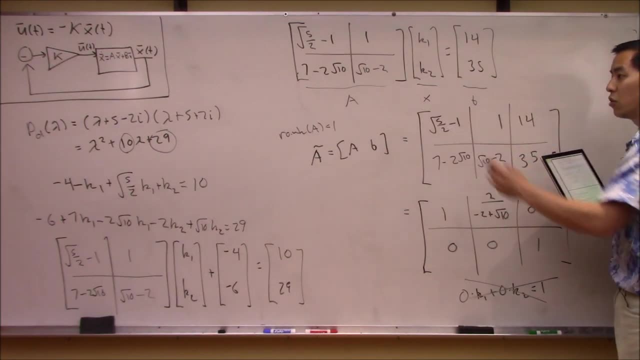 So this is clearly inconsistent, Right, So there's no solution. So in this case the system was uncontrollable. So I can't find a k matrix that is going to move the eigenvalues to the locations that I desire. 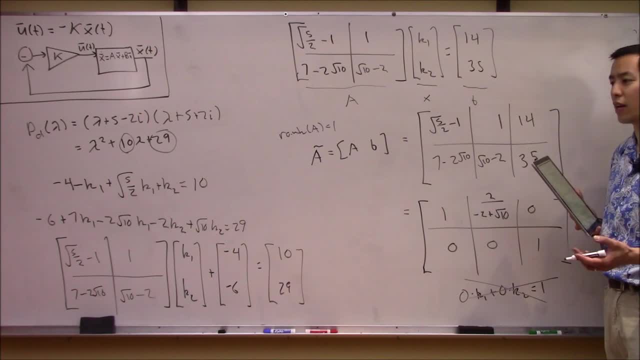 And if you try this in MATLAB, it's also going to choke and just going to yell at you and say: hey, system's uncontrollable, You know? And if you don't believe me here, tell you what. let's run over there and let's do it. 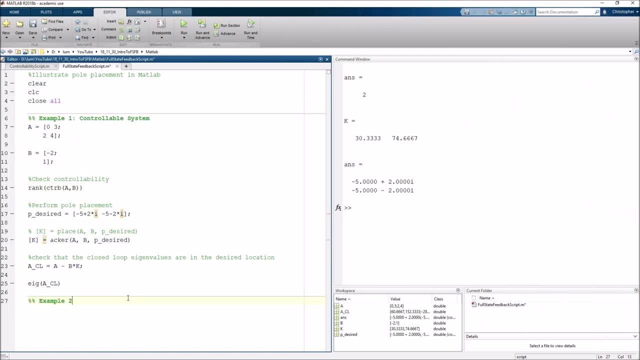 real quick. All right, So let's go ahead and start example 2, which was an uncontrollable system. Okay, So we said the only difference here was the b matrix. So the b matrix now is this weird 0.5 times negative, 2 plus square root of 10 and then a 1.. 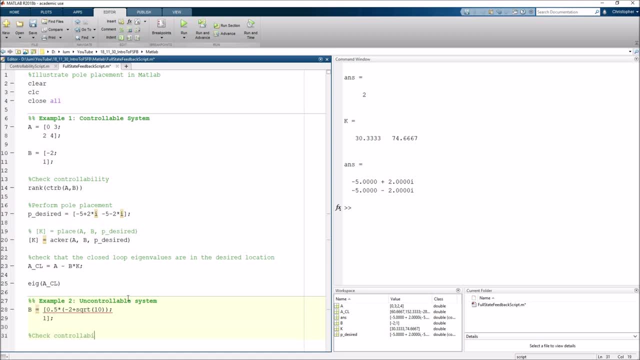 Right, That was our b matrix, So now let's again check controllability, Right? So I'm going to look at rank CTR b of ab And this should be deficient, And indeed it is rank deficient. 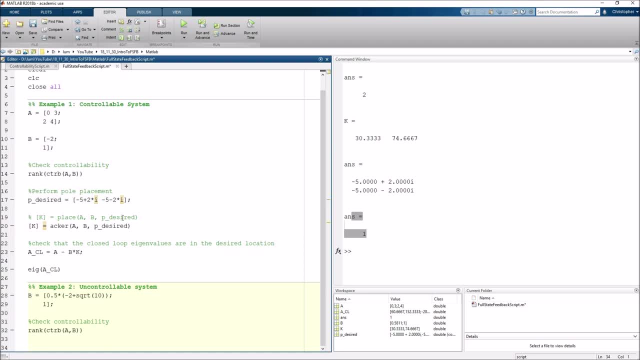 So now, if we go ahead and try to perform pole placement, basically this command up here- let's just go ahead and copy that exact command, because that's all I'm trying to do, is the exact same thing, So I'm going to copy that exact same thing again. 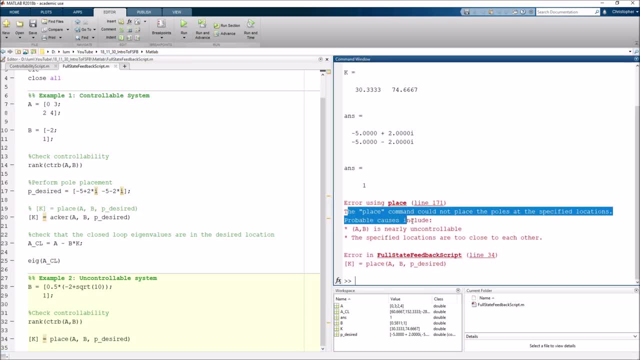 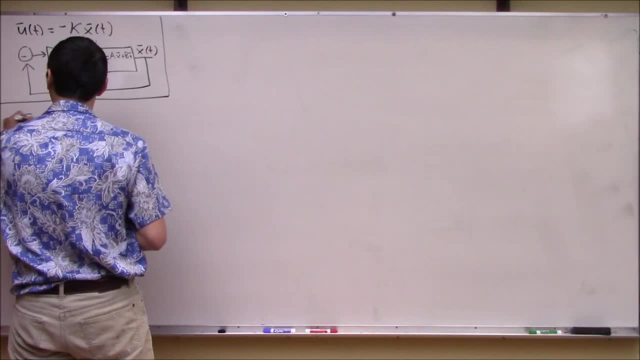 MATLAB is going to not like this And you see, error Right, It couldn't place these because it's uncontrollable. Okay, So let's look at one more example, So example 3.. So this one is going to be again. let's revisit our controllable system. 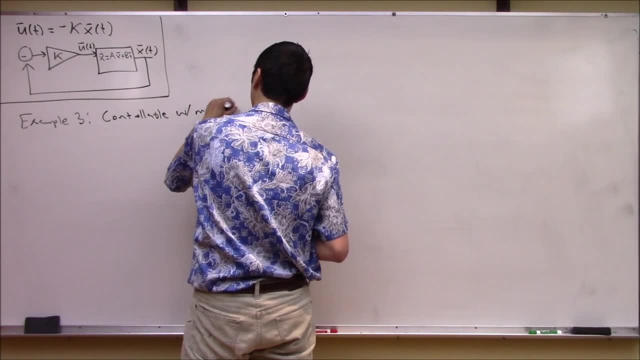 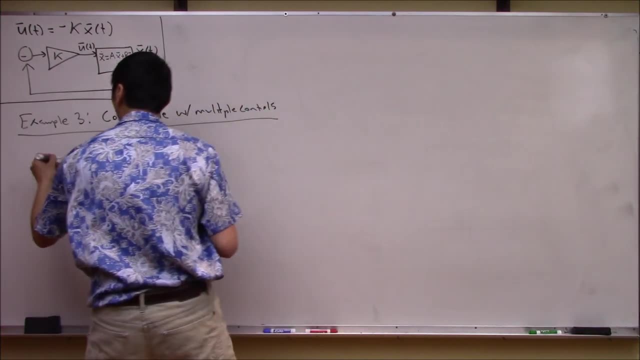 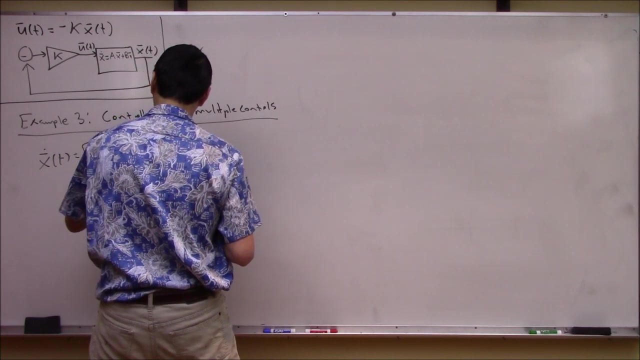 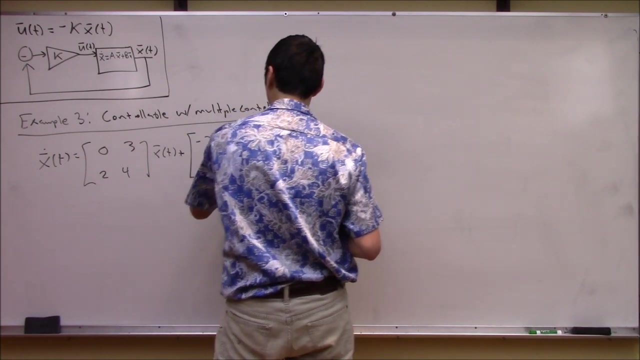 But now let's use multiple controls, Okay, And see what happens. So let's go and revisit the system we had in example 1.. Right, So I think the example 1 we said was something like 0,, 3,, 2, 4, x, plus negative 2, 1, u. 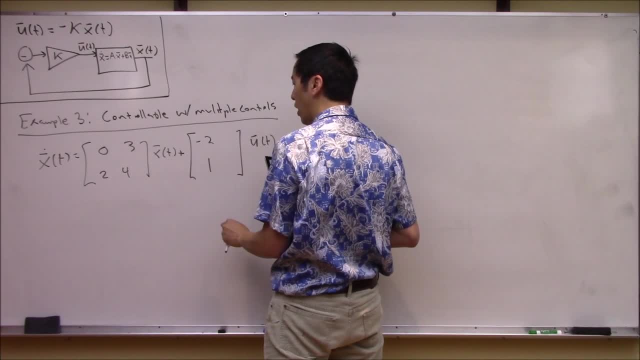 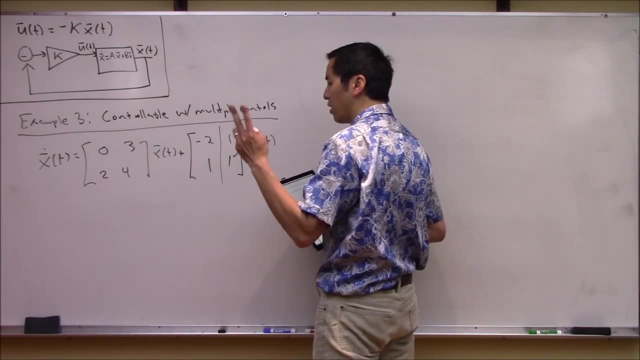 Okay, But now what I want to do here is, instead of just having one input, let's add another column to this b matrix and do something like this: Right, So now, in this case, you see, we've got two control inputs. 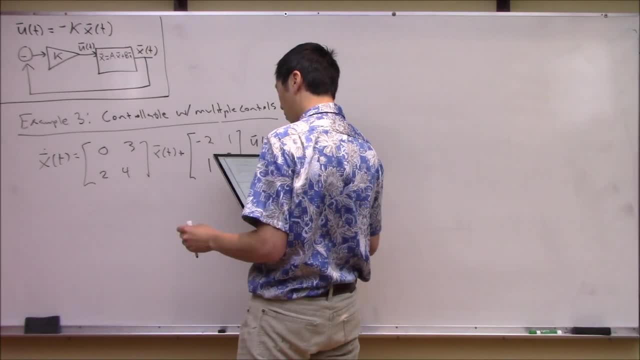 Okay, So in this case now, where I have two control inputs, So again we could check controllability, And you know what I'll tell you: Let's save it until we get over to MATLAB, because MATLAB is a lot quicker than me. just 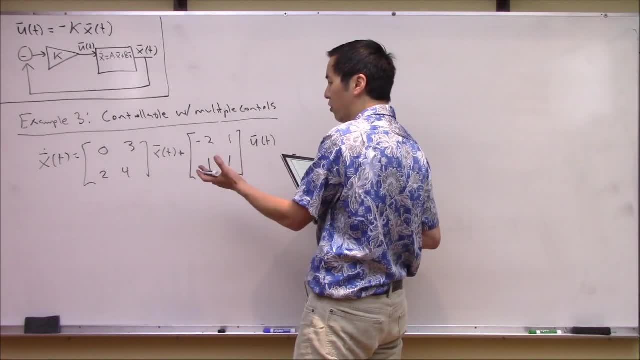 writing out the controllability matrix and checking its rank. Take my word that it is controllable. Well, actually you know what You should know for a fact: that it is controllable, because this is the b matrix we checked already, Right? 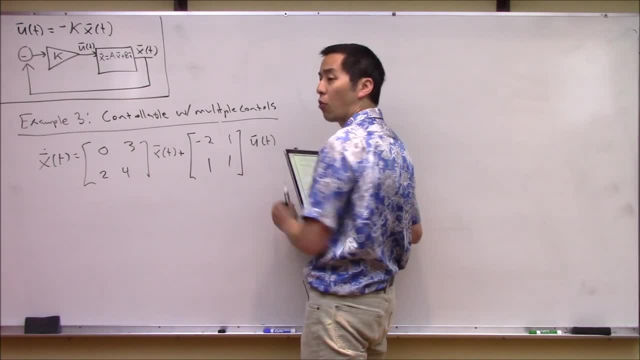 This first column back in example 1. that was controllable. Adding more to this is obviously it's not going to make it less controllable. If anything, it's going to make it more controllable. So this is still controllable. 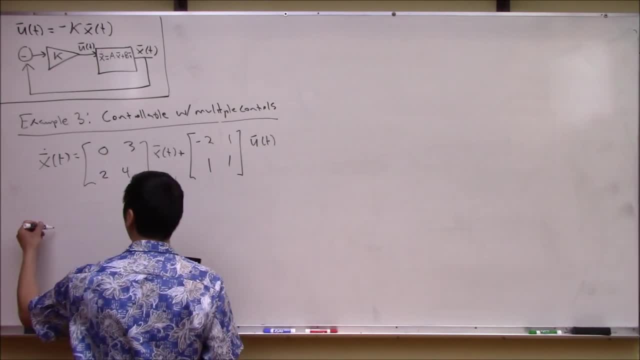 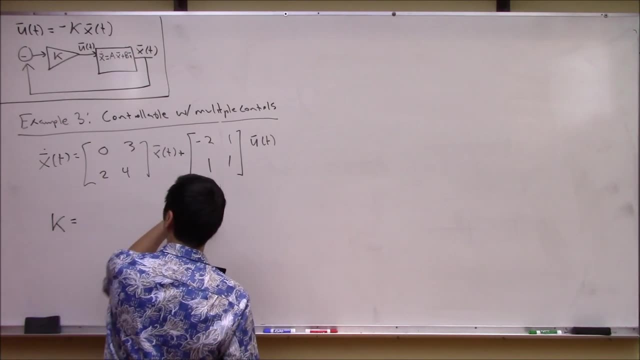 So what we can now do here is: let's go ahead and compute k. So again, make a note here that k in this case- remember we said k was a matrix with as many rows as there are controls. So now this thing has got two rows and now it's actually got two columns as well. 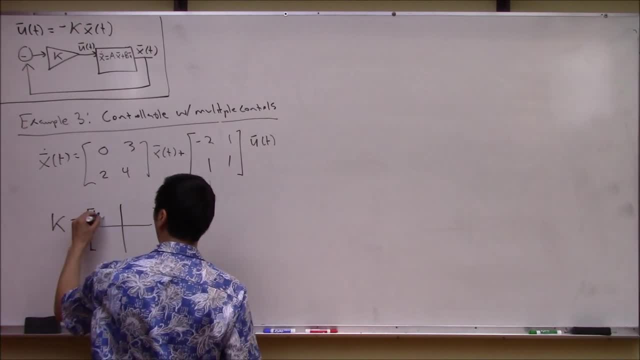 So this thing is actually a 2 by 2.. So now I've got a k 1: 1,, a k 1: 2, a k 2: 1, and a k 2 2.. Right, 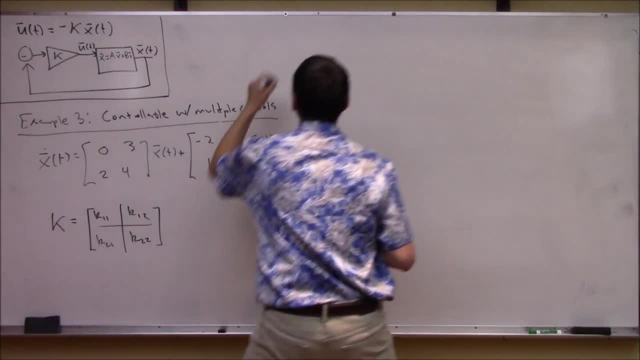 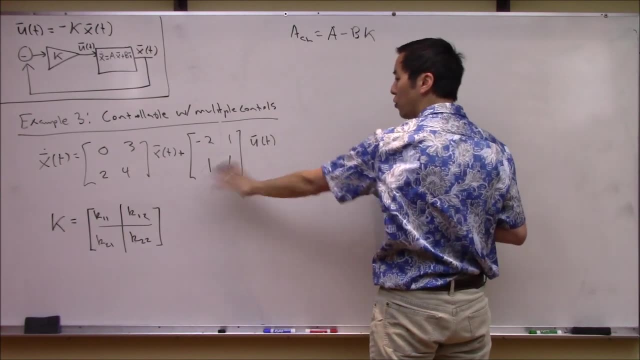 Okay, So we do the exact same thing we did before. So let's go ahead and get a closed loop Right, A closed loop for the overall system. It's still a minus b k, So go ahead and do that matrix math here. 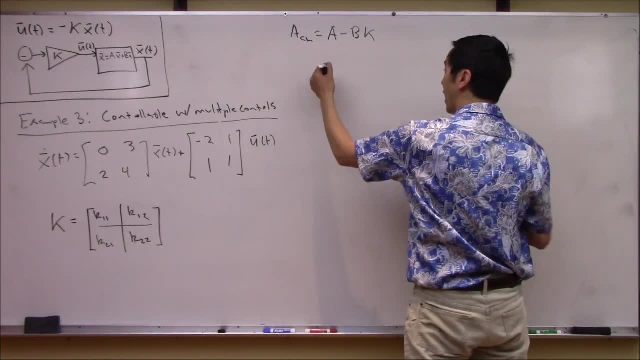 Here's your a, Here's your b, Here's your k. Go ahead and do that. You're going to get something. Let me see It's not ugly, So tell you what. I will go ahead and write it out, just for completeness. 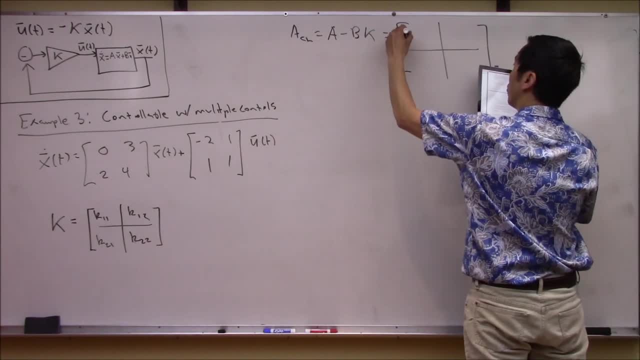 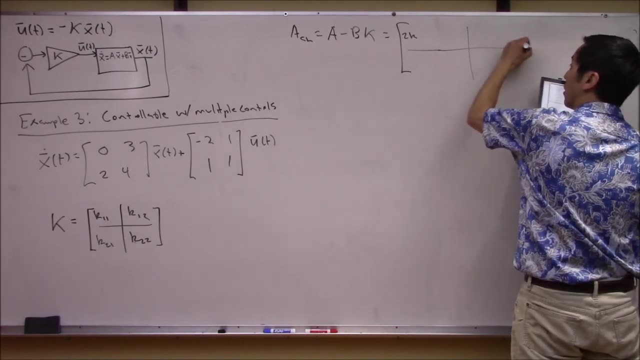 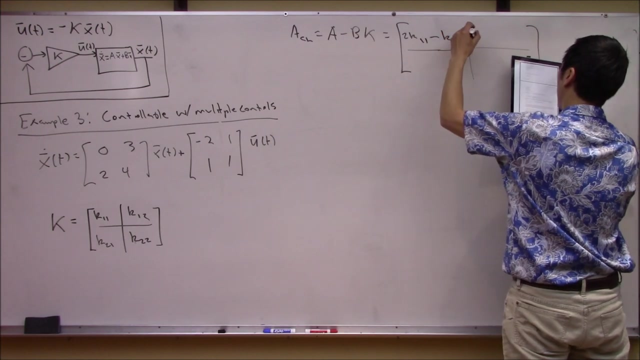 It's not ridiculous. You still get a 2 by 2.. It's 2k. Maybe I need a little more room. Hold on, Makes it a little bit bigger. Okay, So it's 2k1.. 1, 1 minus k2, 1, and then it's 3 plus 2k1, 2 minus k2, 2, and then you get a 2 minus. 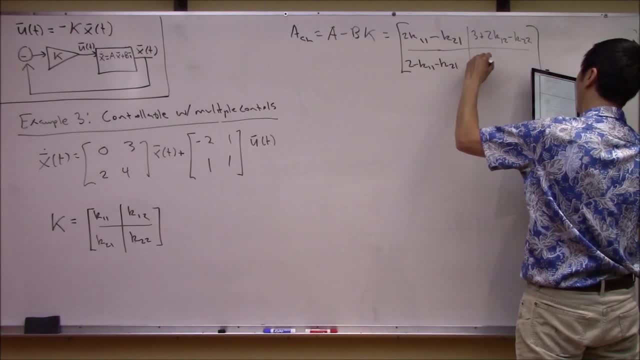 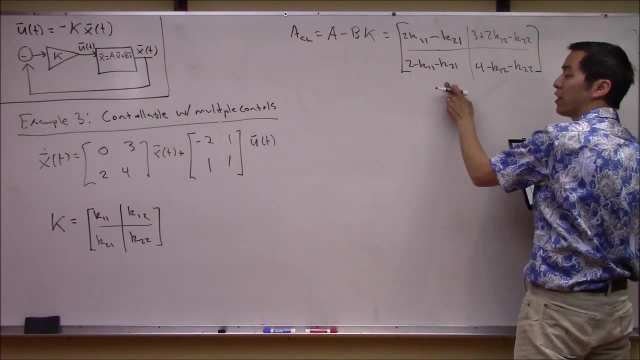 k1, 1 minus k2, 1, and then 4 minus k1,, 2 minus k2, 2.. Okay, There we go. So now let's go ahead and get the characteristic equation of this closed loop system by basically. 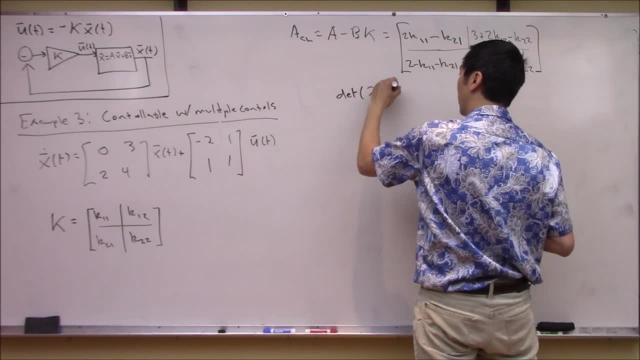 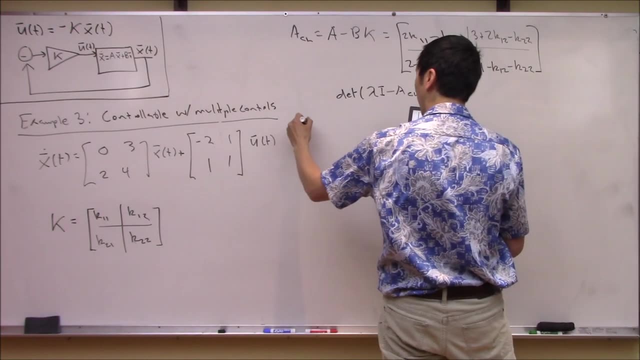 doing our good old friend determinant of lambda. i minus a closed loop is equal to 0. Right, Okay, So this is. This is a little bit more complicated, but still not horribly ugly. I'll write it out for just completeness. 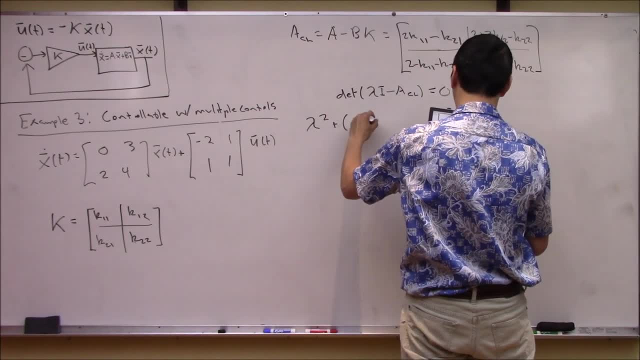 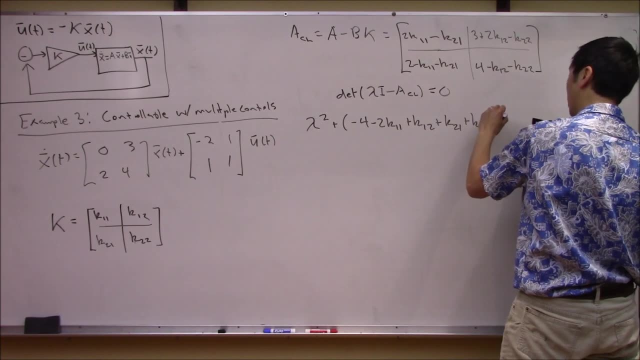 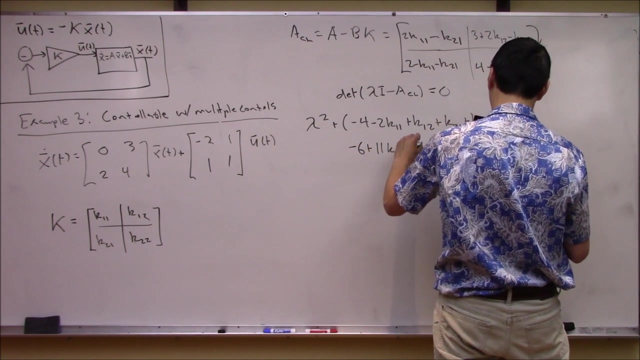 So we get lambda squared: plus minus 4 minus 2k1,, 1 plus k1, 2 plus k2, 1 plus k2, 2 times lambda plus. the constant term here is minus 6 plus 11k1, 1 minus 4k1,, 2 plus 3k1, 2 times. 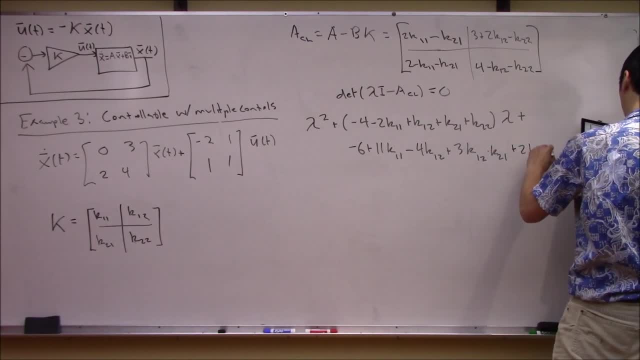 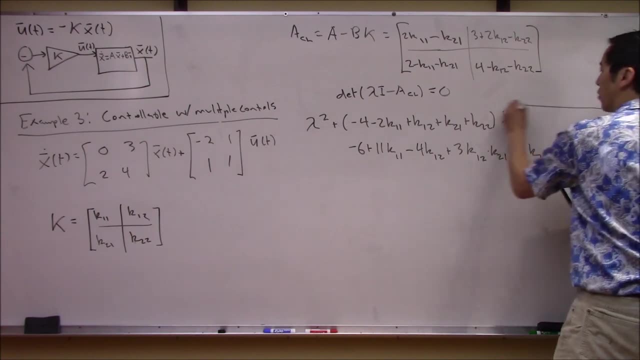 k2,, 1 plus 2k2, 1.. 2, 2 minus 3k1,, 1, k2, 2.. Yuck, A little bit uglier, Okay, So again, box this sucker up. 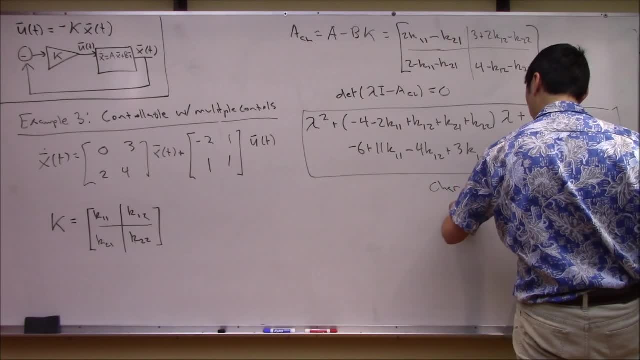 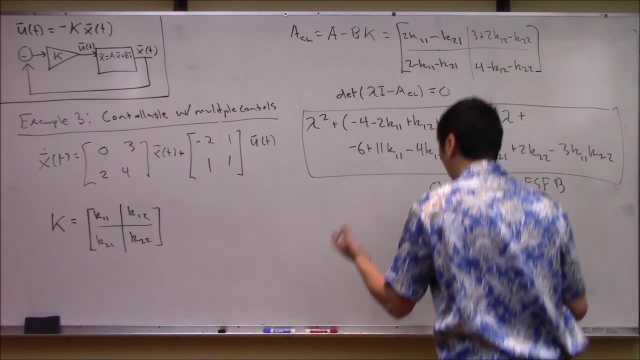 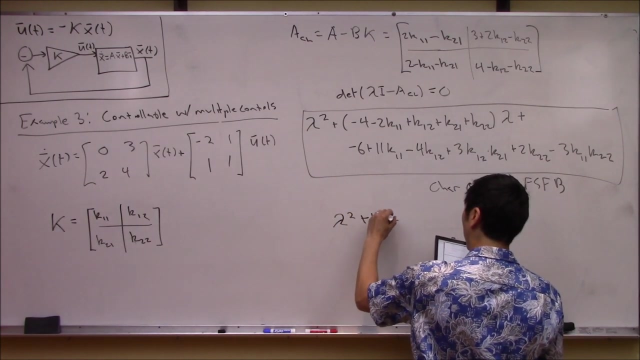 Here's your characteristic equation under full state feedback, Right. And then let's go ahead and compare this with what we want. Let's again use the exact same desired characteristic equation as before. So this was this guy which put our poles at. 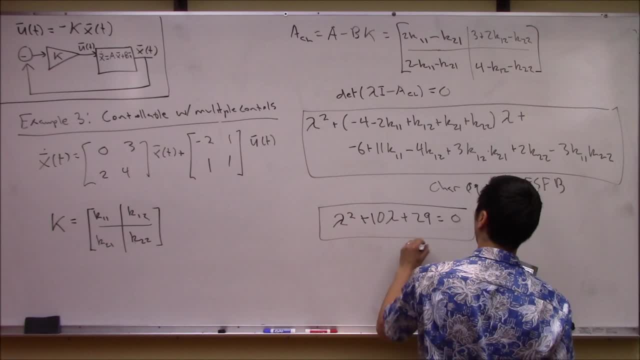 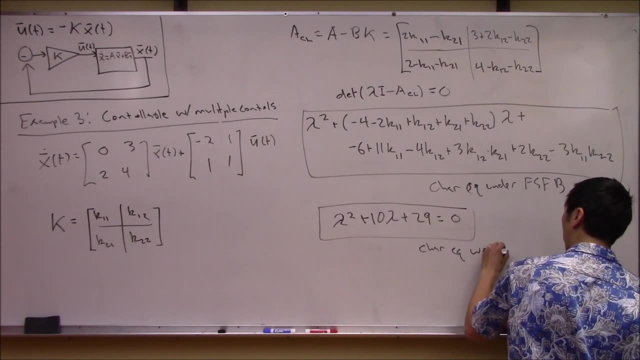 Plus or minus 5, plus or minus 2i. So here we go. So here's the characteristic equation we want. So it's the exact same game, right? Compare the coefficient of lambda with the coefficient of lambda. 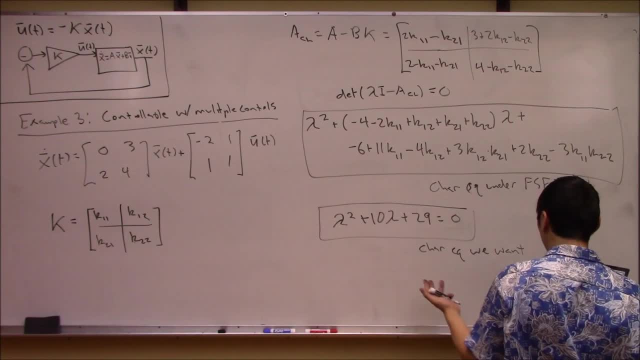 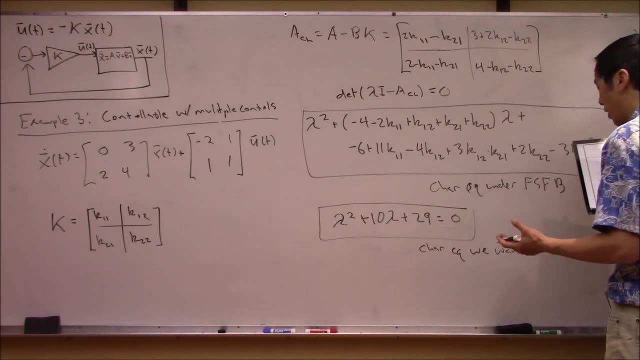 Compare the constant with the constant. But now we see we get a little bit more freedom because we've got now two equations and four unknowns right, So there's an additional degree of freedom here. So, for example, what we could do is we could solve: 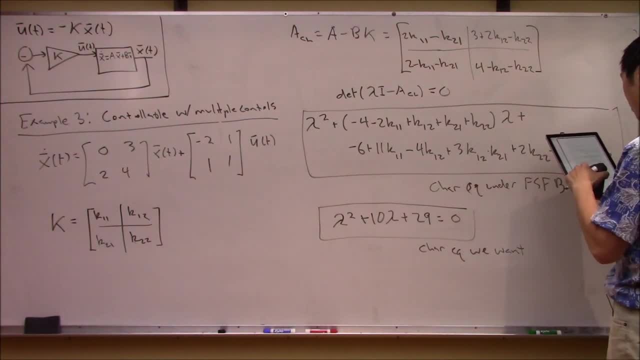 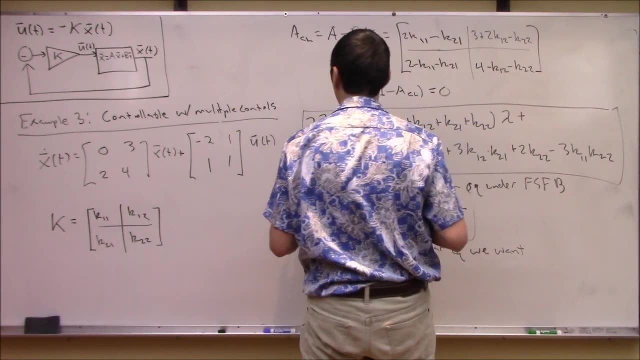 What did I do in my example? Let's solve k21 and 22.. Let's solve the bottom row of this k matrix with respect to the top row. So if you do that, let me go ahead and find some place to erase. 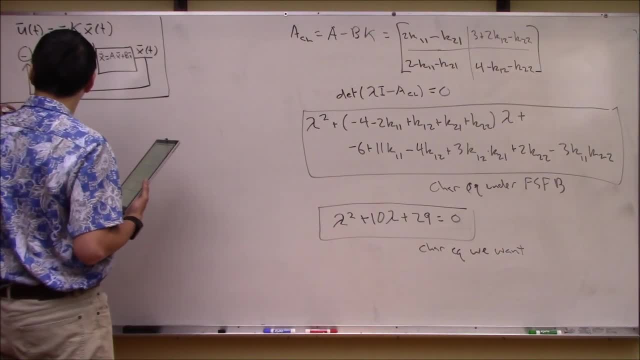 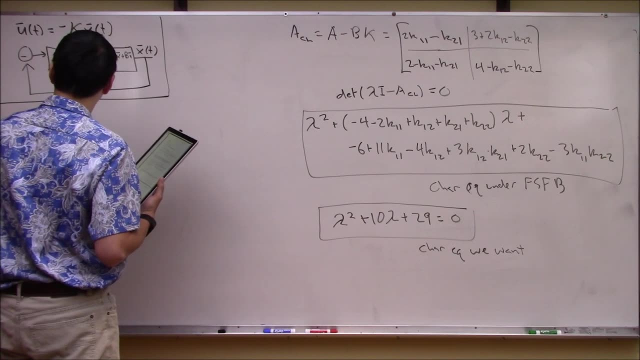 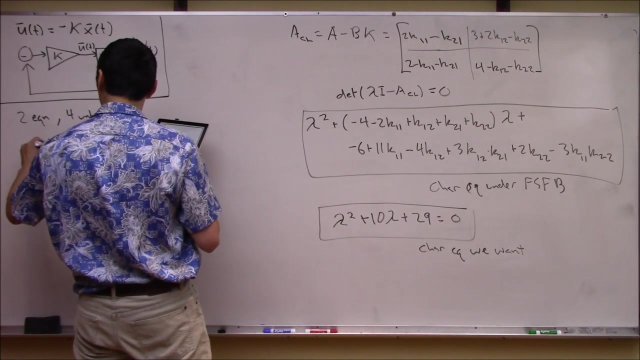 All right, It's just algebra at this point. So what we can say is: again, you've got two equations right, Two equations, four unknowns, So there's infinite solutions In this case. So what you could do is you could get: basically, k21 is going to equal something ugly. 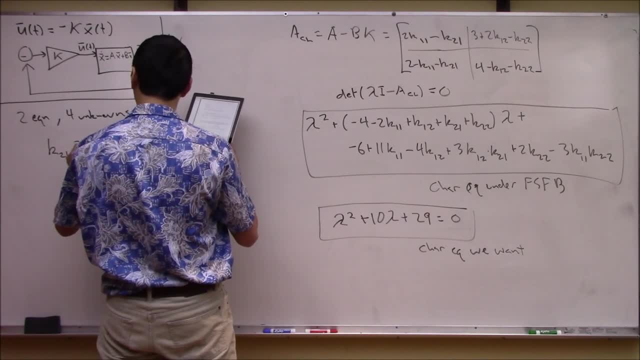 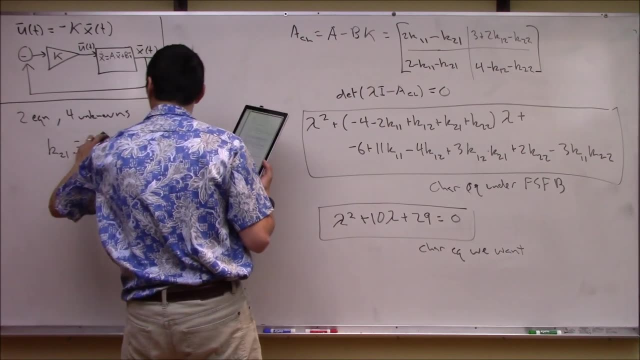 I don't know if I really want to write this all up. Okay, Tell you what. I will write this up once for completeness. Okay, So you get minus 4, minus 2.. Sorry, Whoops, No, I'm looking at the wrong line. 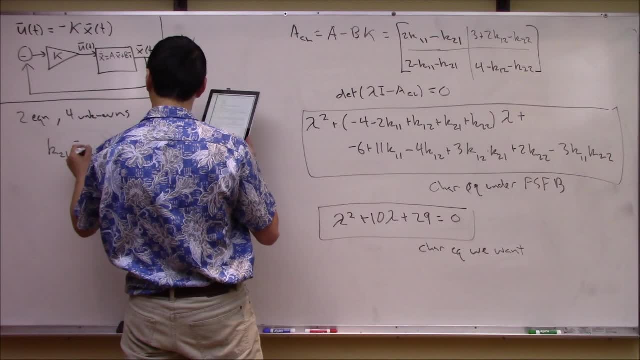 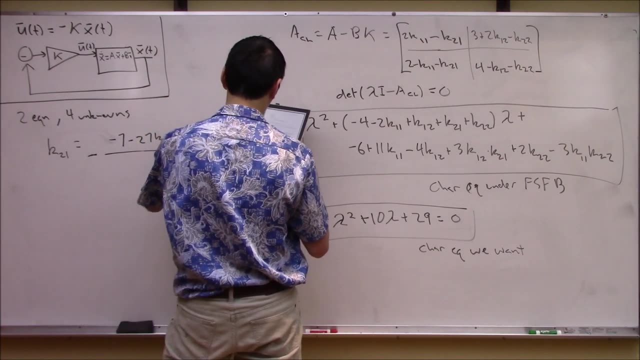 Sorry, All right. K21 is. it's a negative in front of this whole thing. And then you get negative 7 minus 27k11, minus 6k11.. So that's k21 squared minus 6k12 plus 3k11k12, okay. 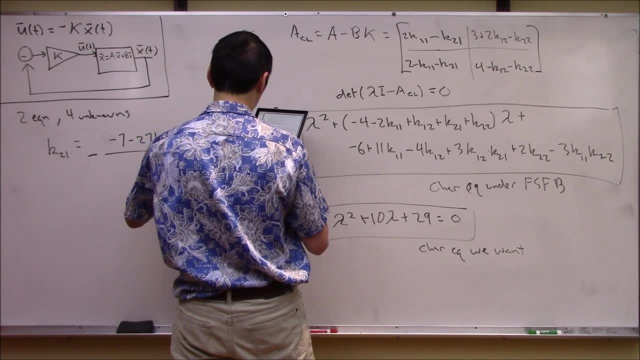 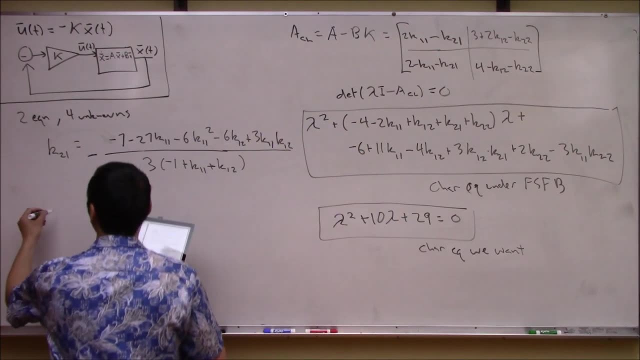 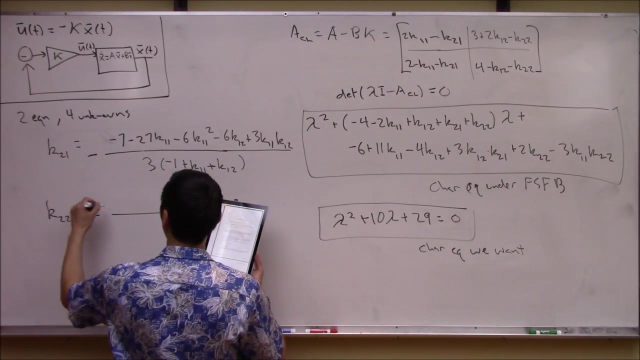 All over 3 times negative: 1 plus k11 plus k12,. okay, So that's k21.. And then k22 is going to be something also kind of ugly. You get a negative and then the fraction looks like 49 minus 9k11 minus 39k11.. 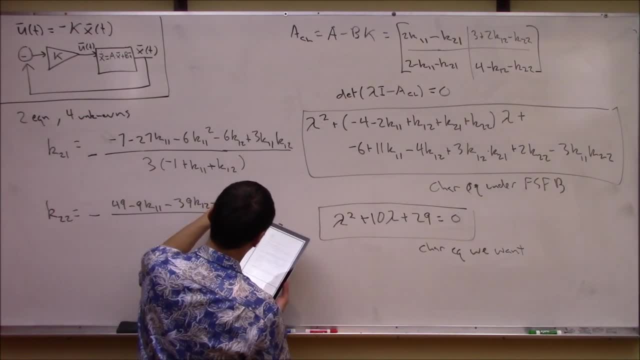 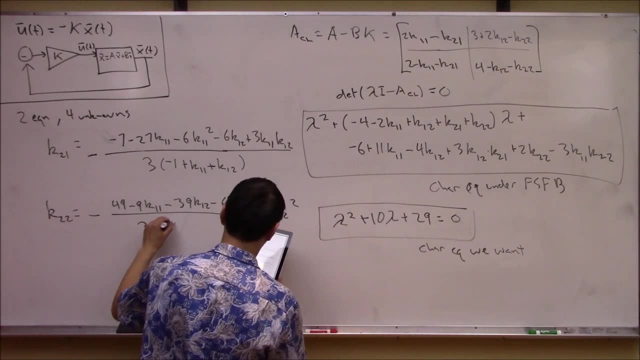 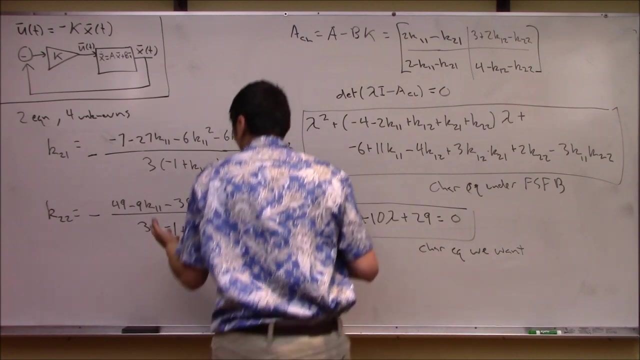 So that's k22 minus 6k11k12 plus 3k12. squared All of this thing over 3 times the quantity negative, 1 plus k11 plus k12.. Yuck, Okay, So a couple of degrees of freedom. 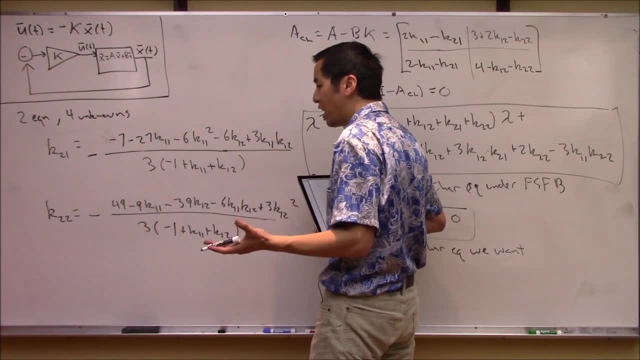 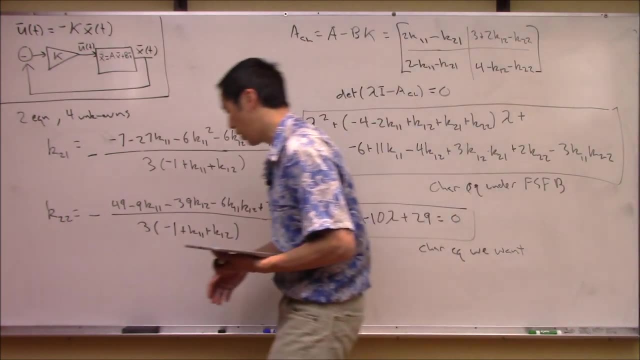 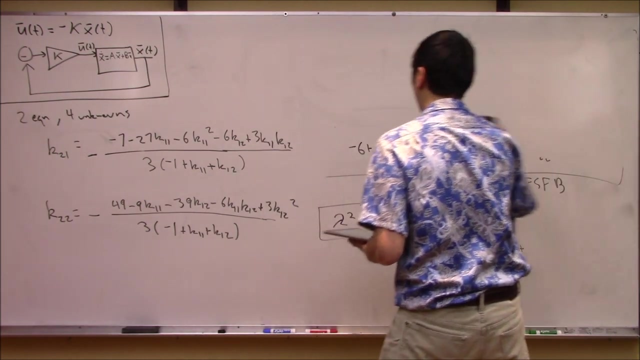 We're now free to choose k11 and k12 to be pretty much anything we want, And then that will dictate what k21 and k22 have to be in order to get the eigenvalues where we want. But This additional degree of freedom is actually nice because it allows us to do other or try to meet other requirements or optimize the system in other fashions. 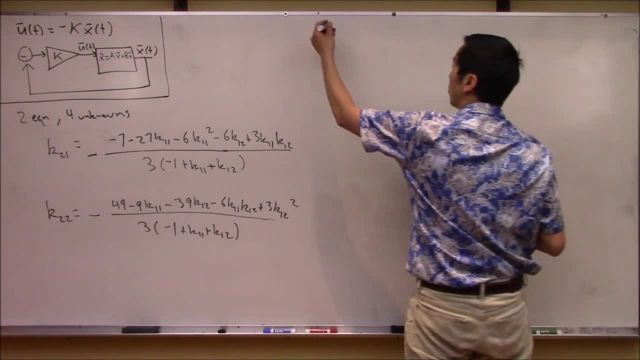 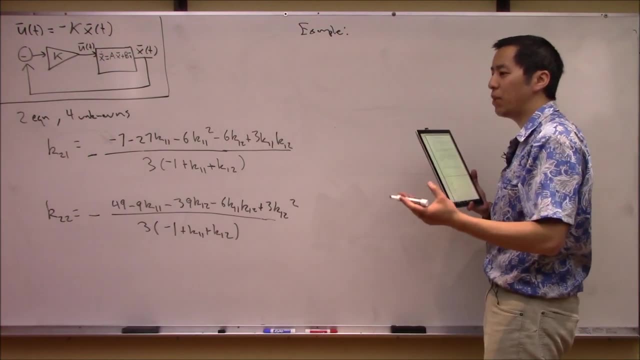 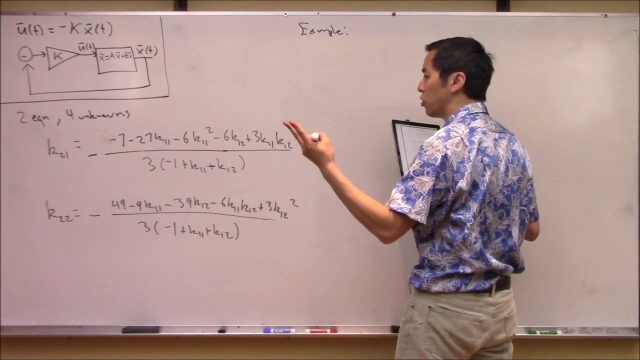 So, for example, you know, one thing you could do is what if we wanted the first control to not be used as much as the second control? If you remember this system here b now there are two inputs. There's a u1 and a u2, right? 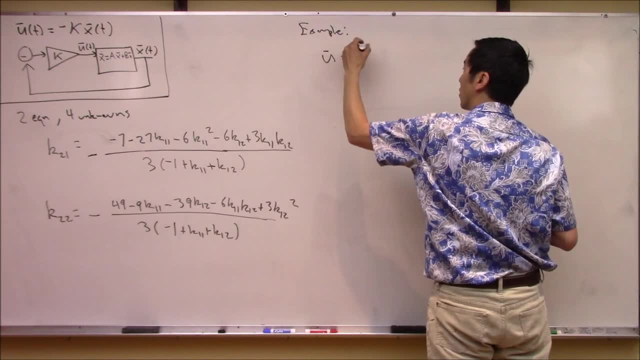 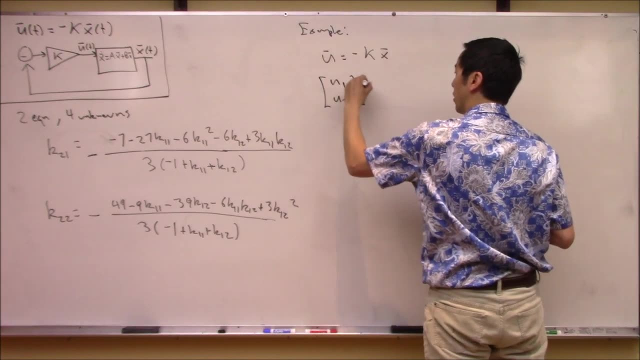 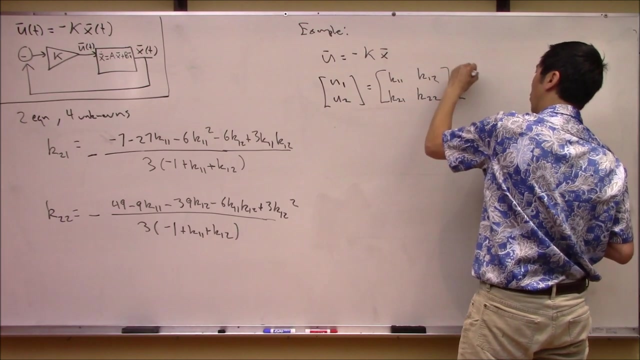 And we said that the control law is: u is equal to minus kx, right? So again, if you write this thing out, this is a u1, a u2 is equal to k11, k12,, k21, k22 times x1, x2, right. 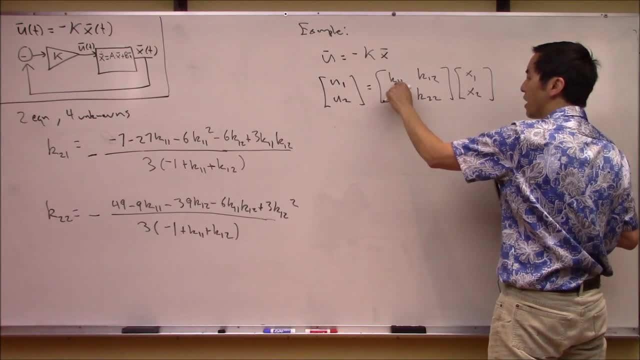 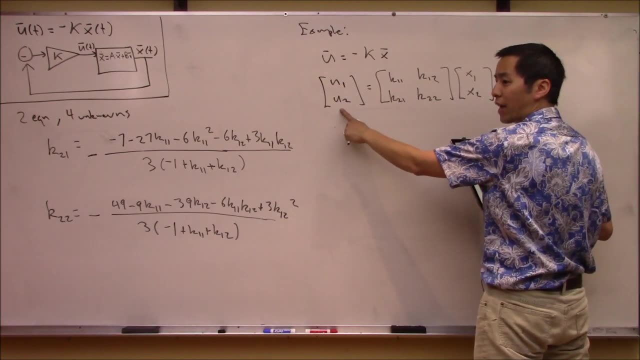 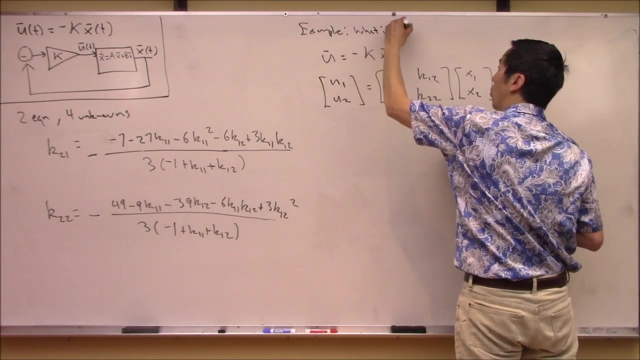 So the first control. you can see that if I make k11 and k12 small, relative to these two, it would mean that the magnitude of u1 is less, Less than the magnitude of u1, relatively speaking here, right? So in this case- example- what if u1 was expensive? 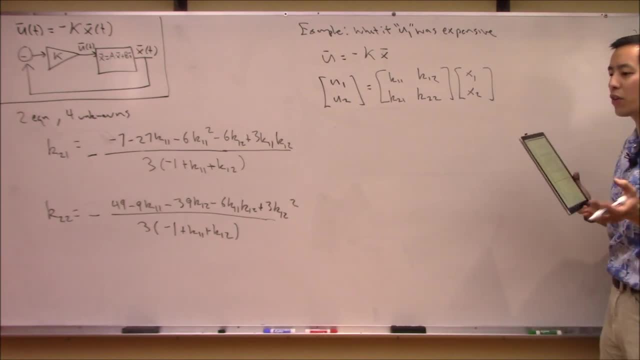 Like u1 was thrust from your satellite or something like that. It was something you know super expensive. It's like jet fuel or something like that. Well, I guess jet fuel is not really that expensive, But you get what I'm trying to say, right. 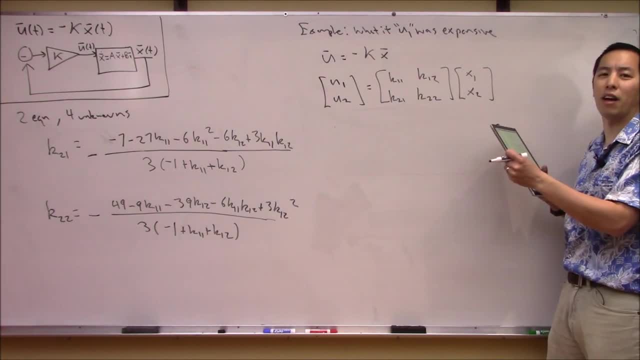 How about u11? is you're shooting babies out the back of your car? Rocket, That's how you're going to generate thrust right, And that's much worse than u2.. U2 is like just using, you know, traditional hydrazine or something like that as a propellant here. 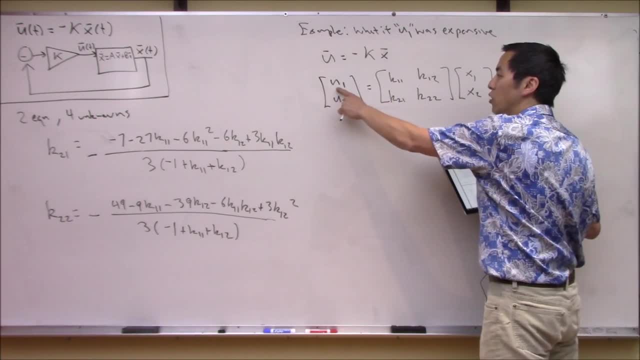 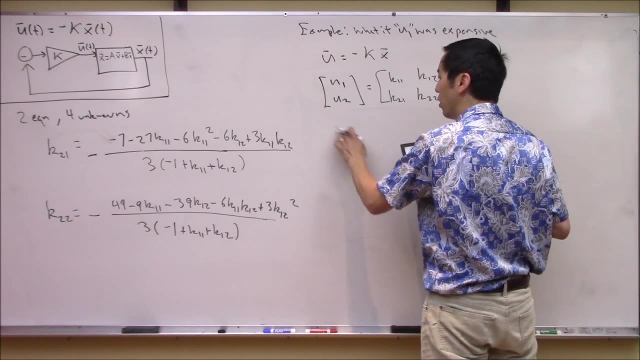 So if I don't, if I want to save the babies, right- If I don't want u1 to be large, what I would then want to do is make sure that k11 and k12 are small. So, for example, you know now what we can say is: let's go ahead and choose. 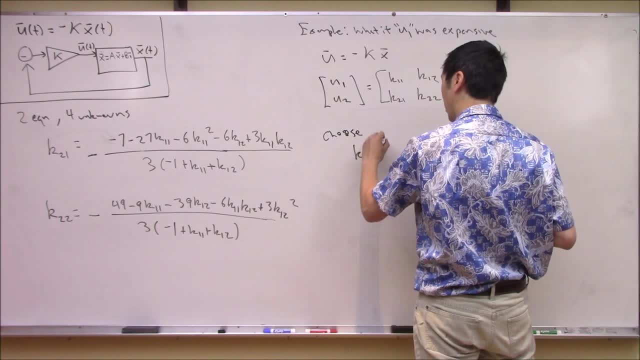 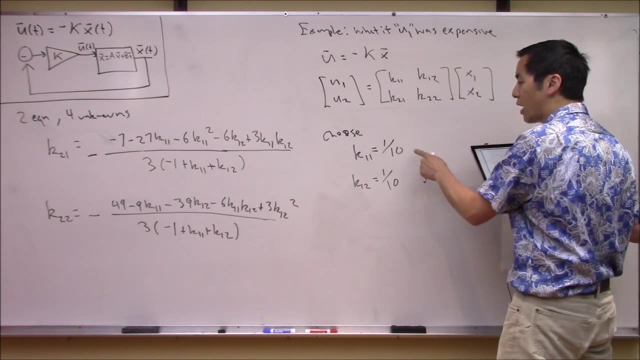 Since we're free to choose, I can say: how about? k11 is like one-tenth And a k Sorry one-one, And k12 is also a tenth, Something small, Okay. So now, what I would do then is plug these numbers back into these expressions to get what is k21 and k22 have to be. 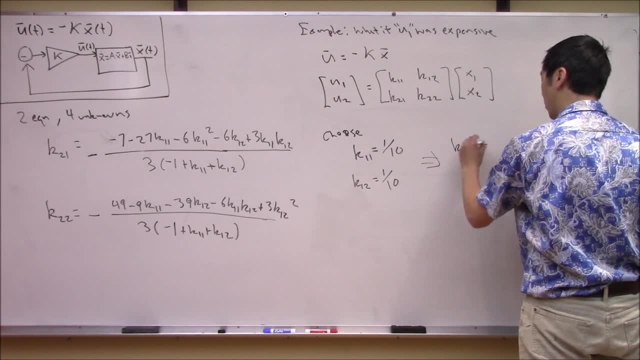 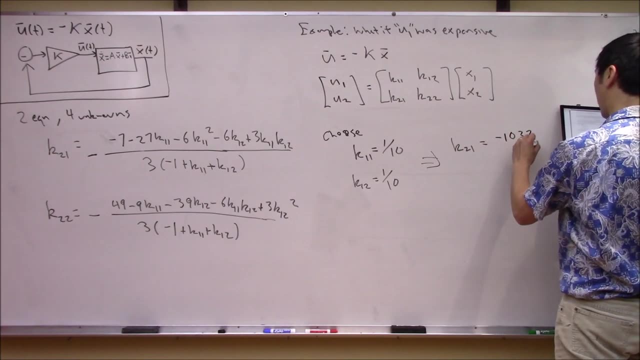 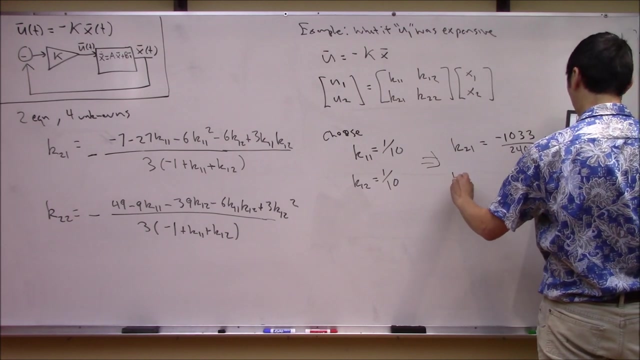 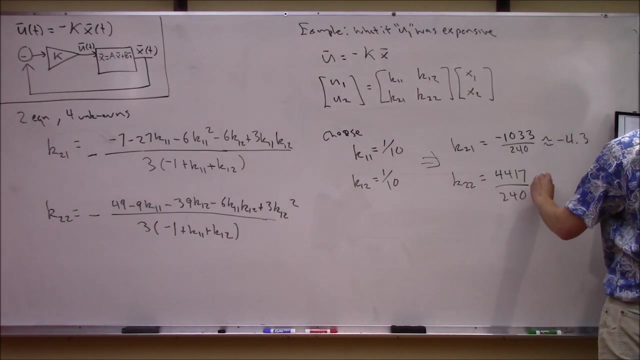 So if you do that, you would end up with k21 as being what was this? Something like minus 1033 over 240,, which is about negative 4.3.. And then k22. Would be 4417 over 240,, which is about 18.440, right. 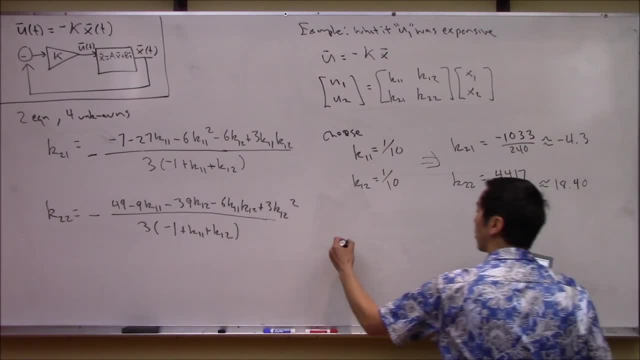 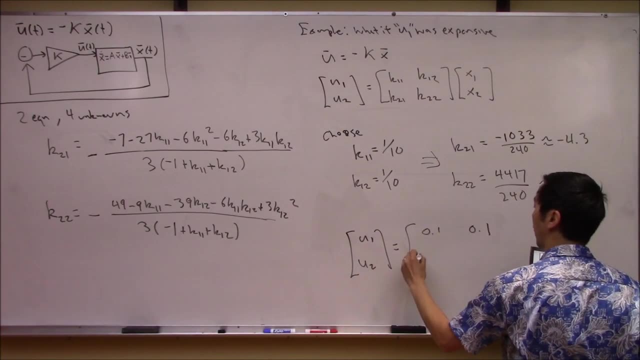 Okay, great, So this k matrix now. So now we see that the control law right, So u1 and u2, it's going to be 0.1, 0.1, and then negative 4.3, and then 18.4 times x1, x2.. 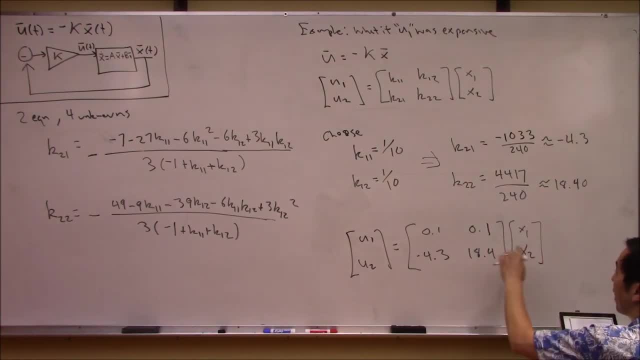 So we can see that for a given x right, If x1 and x2 are, let's just say both of these are one right, So this vector is ones right. So out here, what u1 would evaluate to is just what. 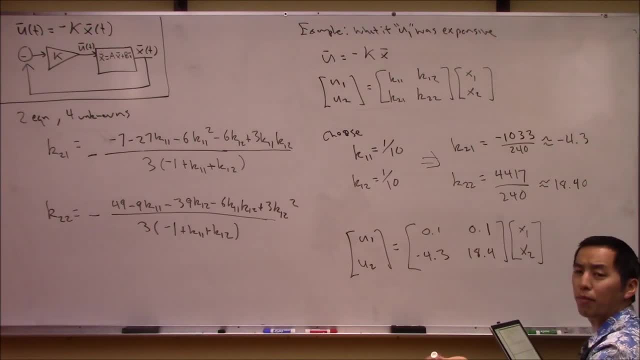 0.2, right. So you only shoot 0.2 babies out the back of your rocket. That's less. that's like what? A fifth of a baby? I guess that's okay. I guess I can live with that right. 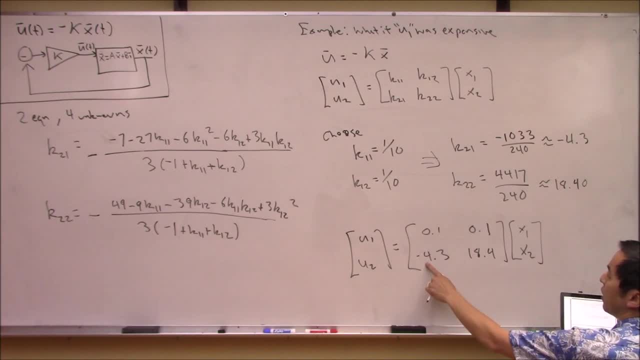 But down here, how much hydrogen are you burning? It's actually what: 4.3., 4.3., 4.3., 4.3., 4.3. So it's like 14 units of hydrogen. 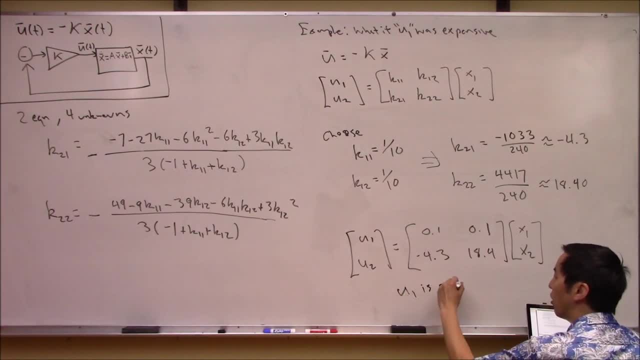 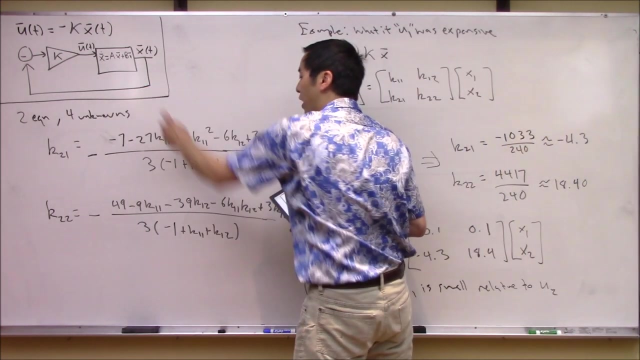 So you can see in this case that u1 is small relative to u2, right, So this is nice. So the pole placement technique- and what's great about this is this K matrix- still will put the eigenvalues of the system, the closed loop system. you know this whole thing. it. 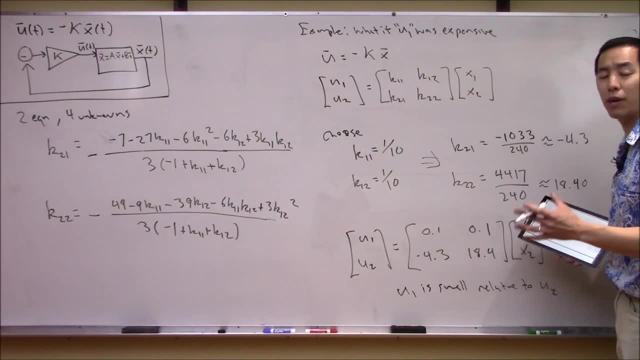 will still put it at the desired locations of minus 5 plus or minus 2i, right. So this is great. It shows us there's a little bit of wiggle room, So, and the pole placement technique can still grace. well, I don't know if I want. 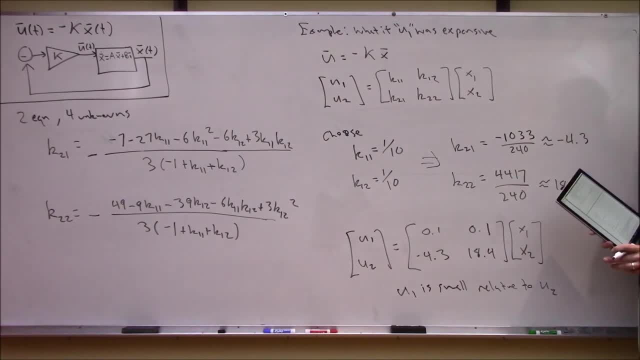 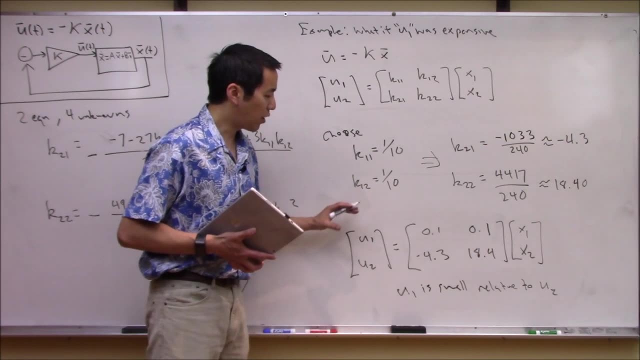 to say gracefully, but you can still take it into account if you manually do this. This sort of sets the stage for our discussion later on, where we're going to start talking about linear quadratic regulators, or LQR, and this is another way that you can use to. 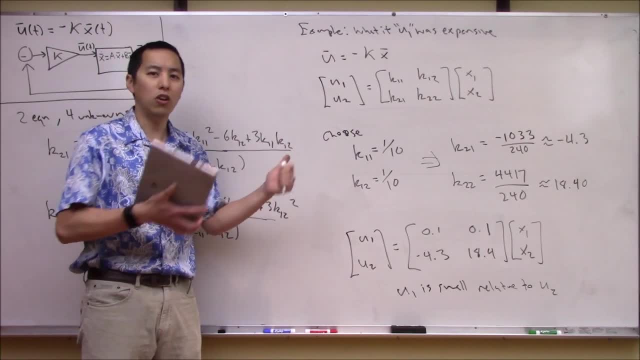 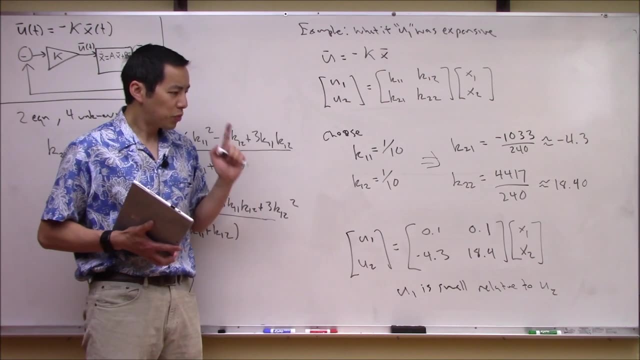 tune. which one of these controls do you care about more, and use pole placement or full state feedback in this entire framework, But I think I'm getting a little bit ahead of myself. Maybe what we should do, though, is let's run over to MATLAB and see that. how is MATLAB? 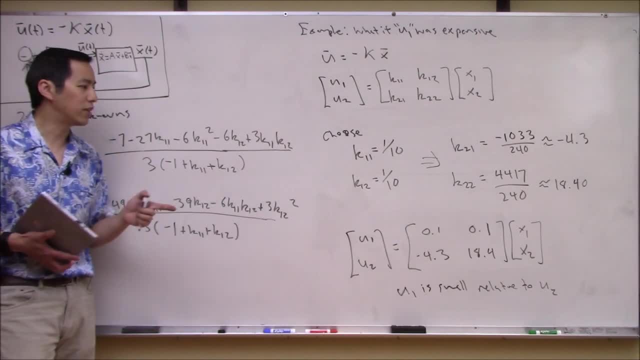 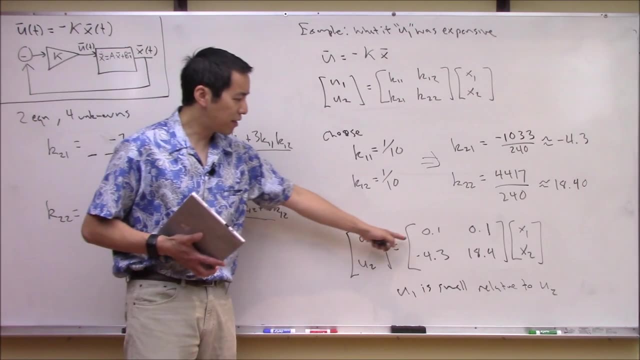 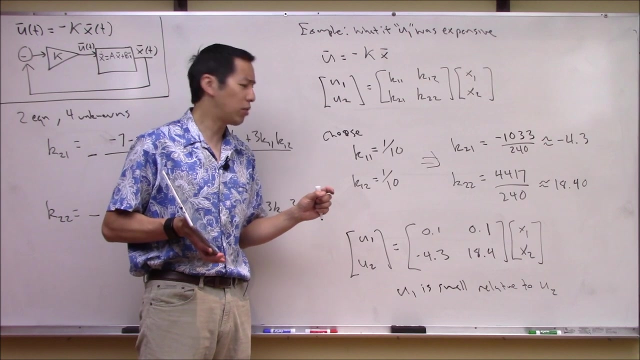 going to handle this situation where we have more than one control input and we're trying to design a K-matrix for this system. So again, keep this in mind: that this is the K-matrix we designed ourselves manually because we wanted to tune. how many babies are we shooting out of the back of this rocket? 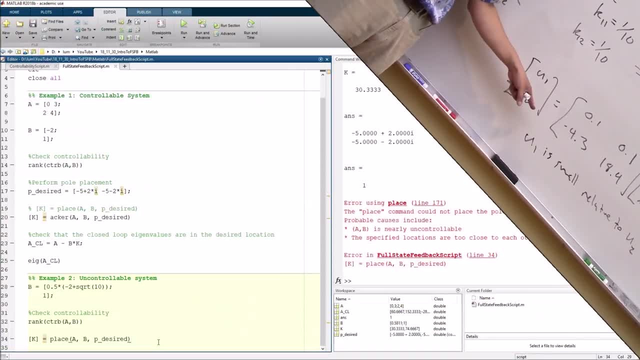 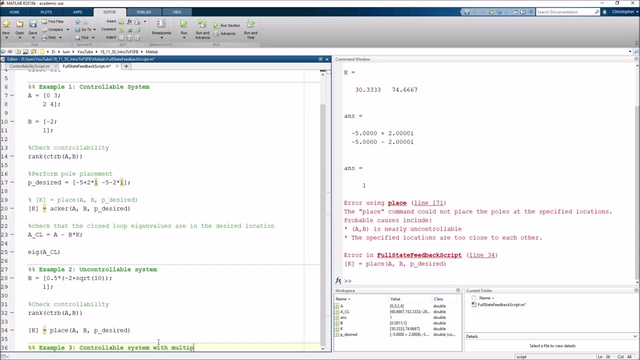 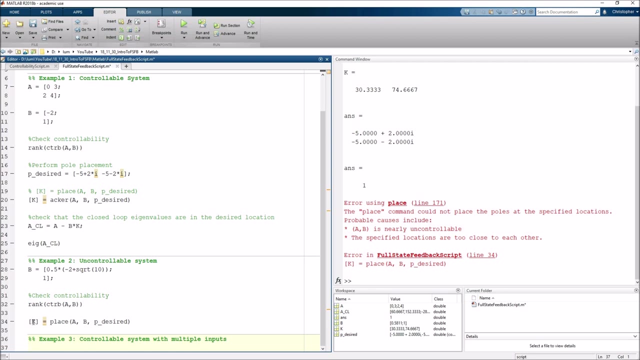 And let's go see what does MATLAB do automatically. All right, so let's go ahead and start. example three: This was our controllable system: Multiple inputs. okay, So actually, before we get started, let's comment out line 34, because we saw that this is going to choke, right. 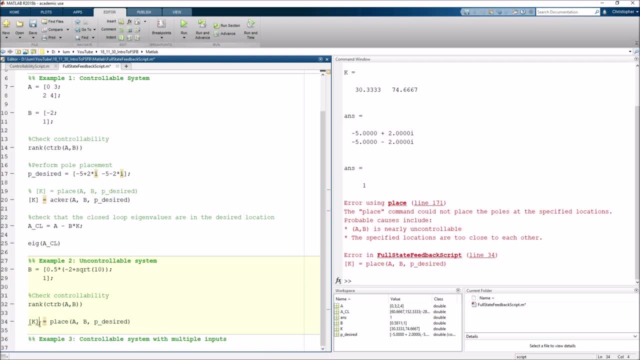 Line 34 was where we had. you're trying to place an uncontrollable system, so this is not going to help us, So let's comment that out, Okay, so now what we said is all we're going to do is augment the B-matrix. 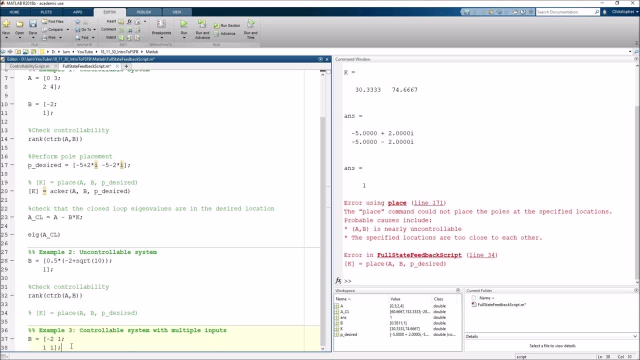 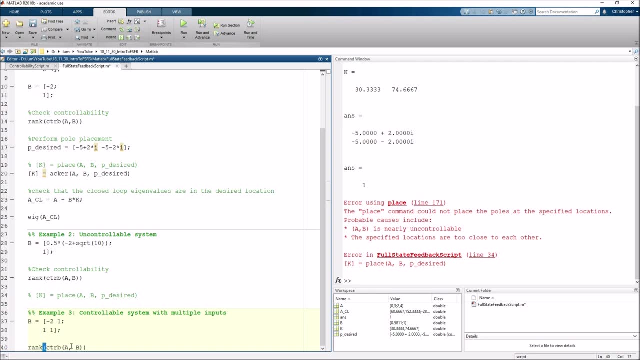 So I think our new B-matrix looks like this: right, This is the B-matrix with two controls. So again, let's go ahead and rank check this thing of the controllability matrix to make sure we- uh, make sure we are fully controllable. and yay, here we go. 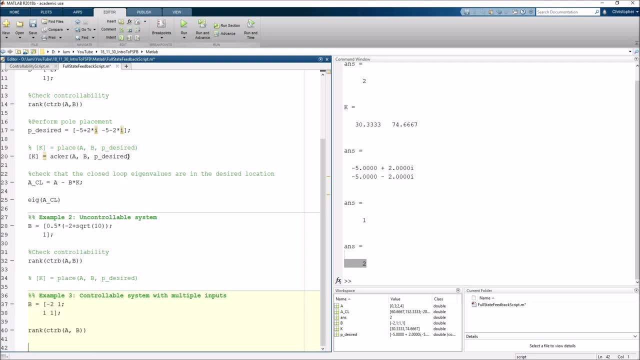 So now I can- well, you know what it's actually- just this command. all right, It's our Place command. So again, let's copy this, paste it down here And we should be good to go. And here, here you go. 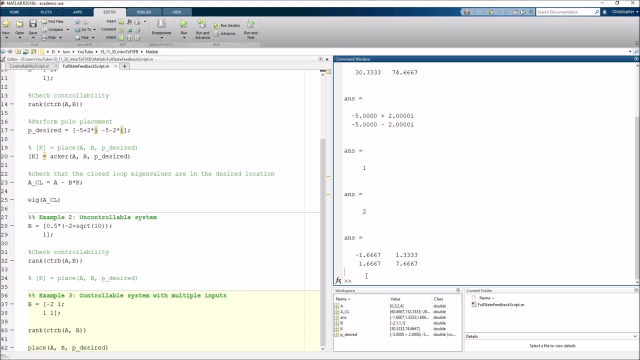 So interestingly, look at this. uh, since Place uh doesn't have any knowledge of how much, do we want to penalize one control versus the other or any of these other ways that Narrow down the degrees of freedom, right? 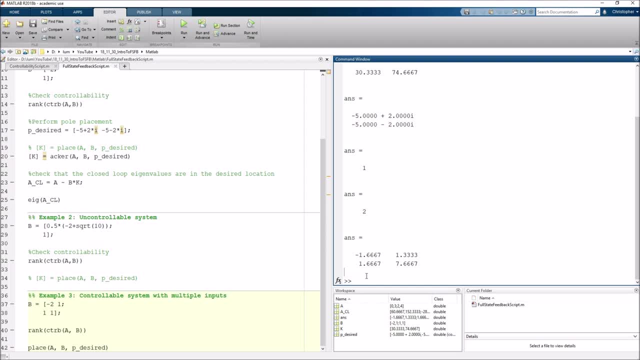 We said there's infinite solutions, so here's one that MATLAB chooses for us, right? It decides that here's a gain that should work. Let's just verify that, maybe. So let's come back over here and let's store this to a variable k. 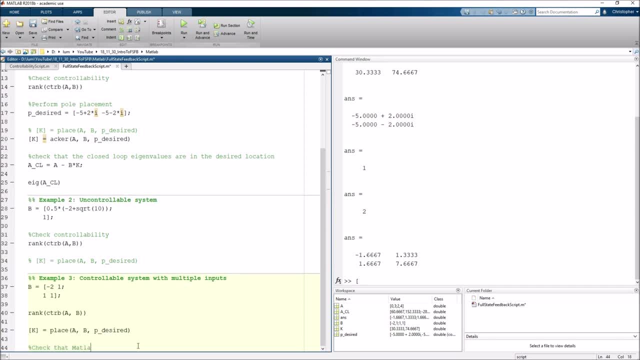 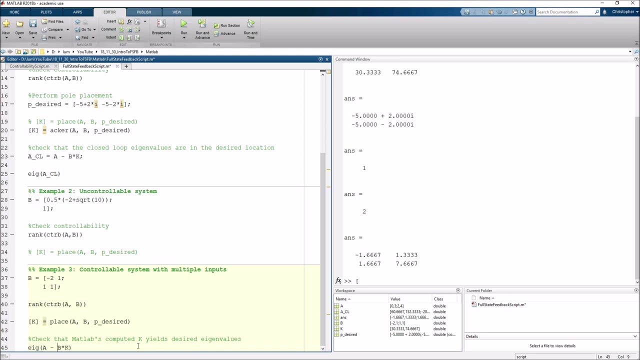 and just go ahead and check that MATLAB's computed k yields acceptable or desired eigenvalues, right? So I want to look at eig of a minus b times k, right? So run this sucker and yay, it totally works. right to put it where we want it to be. 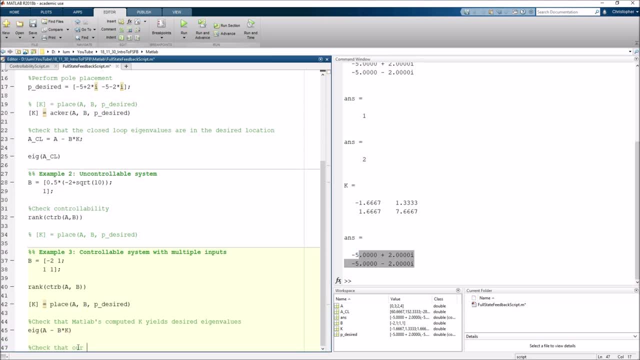 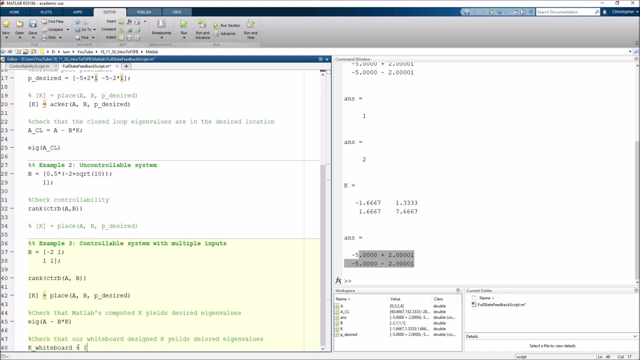 However, let's go and check that our whiteboard designed k's, yields desired eigenvalues, right? So k, let's call it k. How about whiteboard, right? This is what we did up on the whiteboard. What did we say? this was: 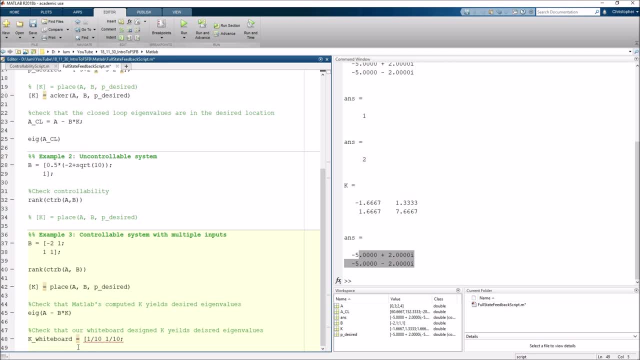 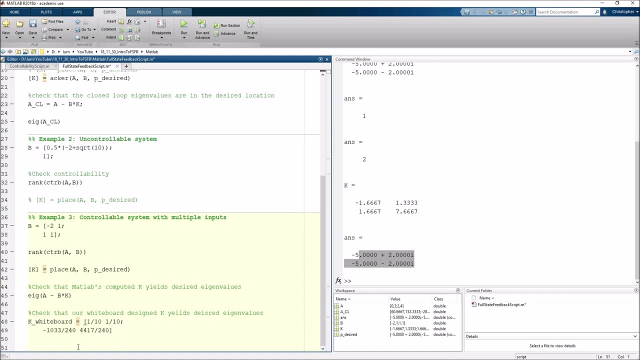 This was 1 tenth, 1 tenth, and then I think it was negative: 1033 over 240 and 4417 over 240, right, So now let's go ahead and check that the eigenvalues of a minus k whiteboard get us where we want as well. 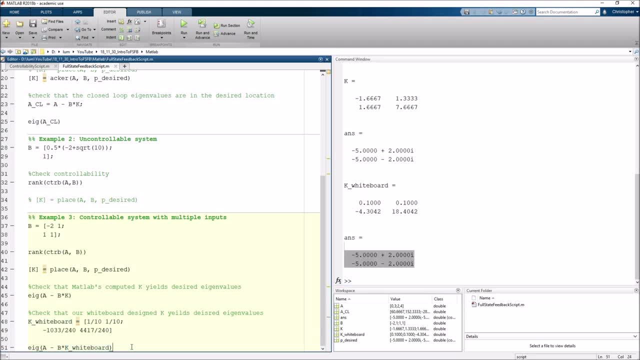 And there you go. Look at this, It also works. So again, there's multiple ways to skin this cat in the situation where you've got multiple inputs because we've got more degrees of freedom. We've got more degrees of freedom than we have constraints. 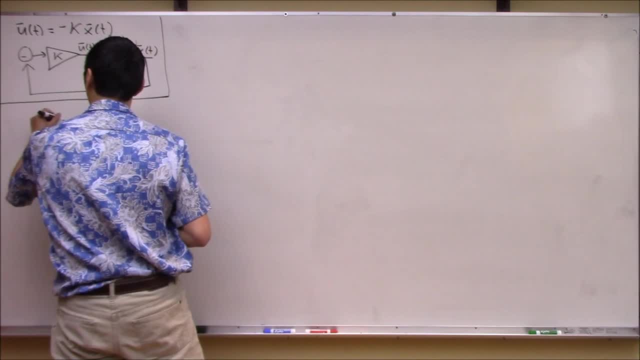 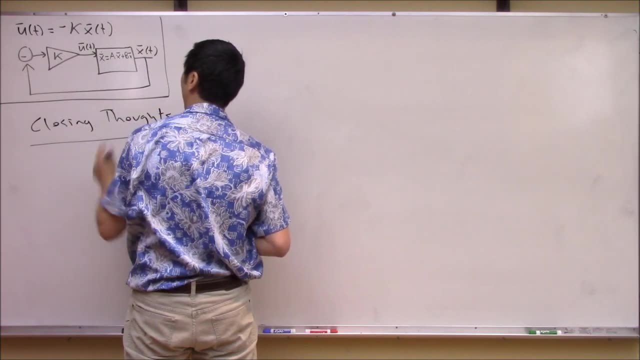 All right. so I want to leave with a couple of closing thoughts. So the first thought is: if you look at the control law here- u is just equal to minus kx- we see that full state feedback is approximately. it's basically proportional control, right. 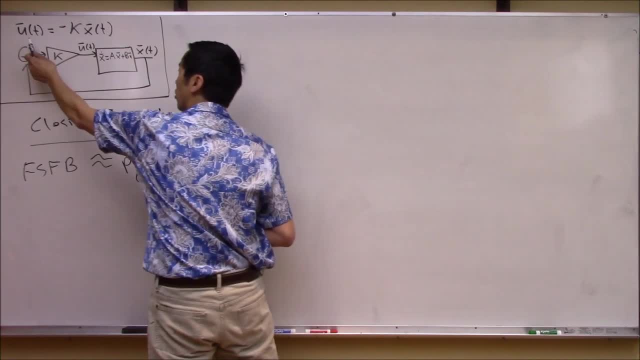 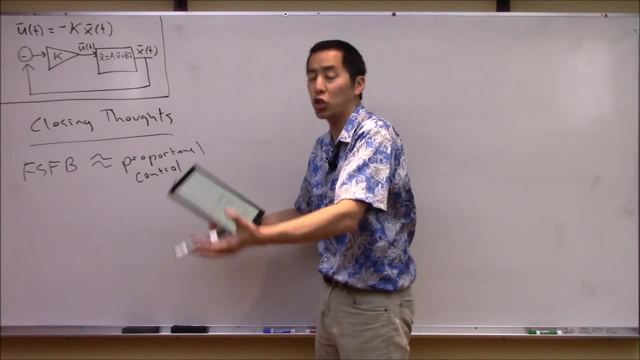 In the sense that to compute the control right now, all you do is you take the current state and you multiply or you proportionate it. Well, that's actually not a verb, is it here? But anyway, the control is directly proportional to the current state, right? 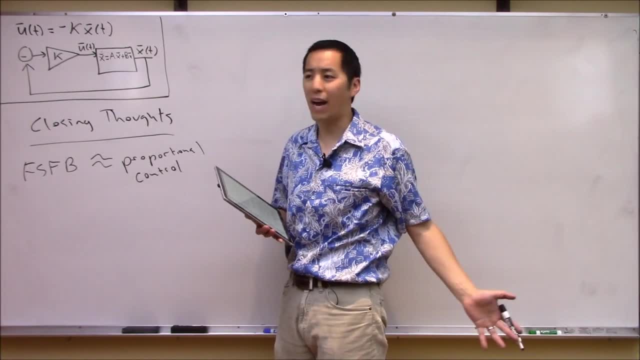 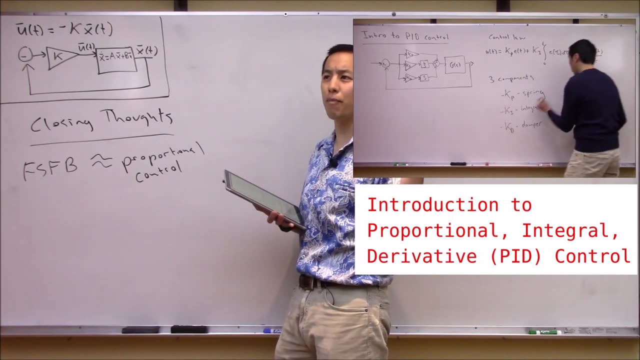 So you don't need anything, any information about the past, right? So, like an integrator, right With PID control, we saw that you needed to add components that would have some idea of the past and you also had things that needed had rough ideas of the future here. 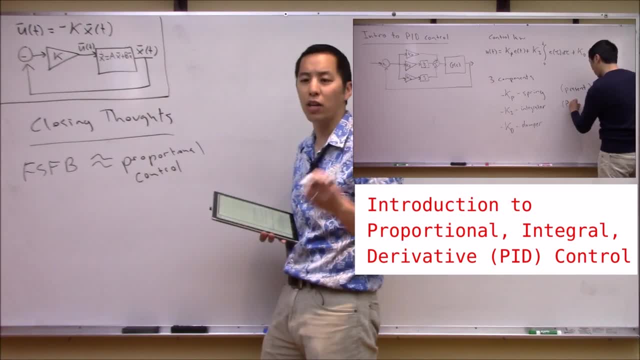 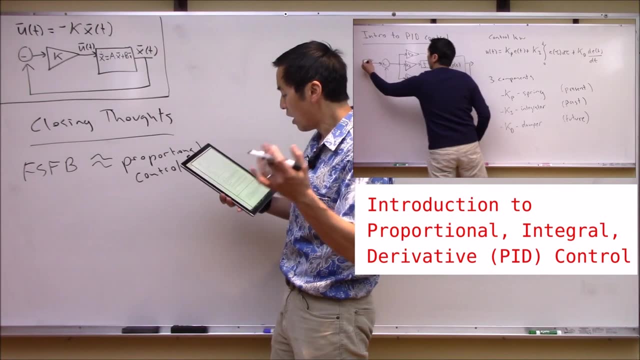 But you don't need any of that stuff here. with full state feedback control, It's really simple. I can compute the control, the control input, now, based on the information I know. now I don't need anything else. The other thing to think about here is, while we're talking about maybe comparing it to PID control, 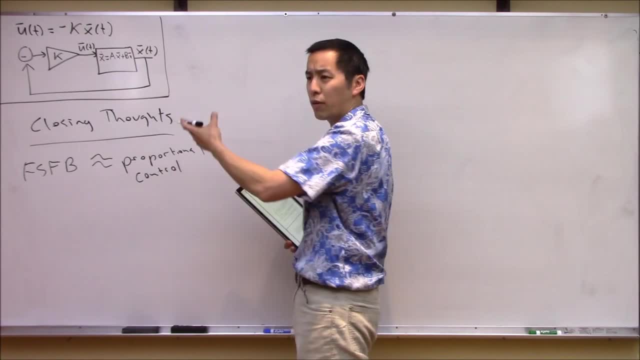 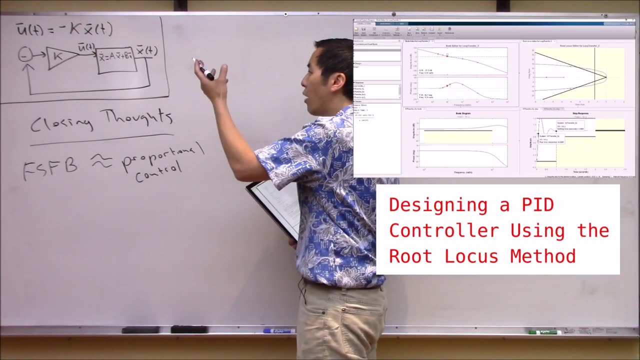 if you remember, here, when we were talking about PID control, we looked at designing them via root locus. In fact, we looked at designing any linear controller using the root locus technique With full state feedback control. there's no concept of root locus right. 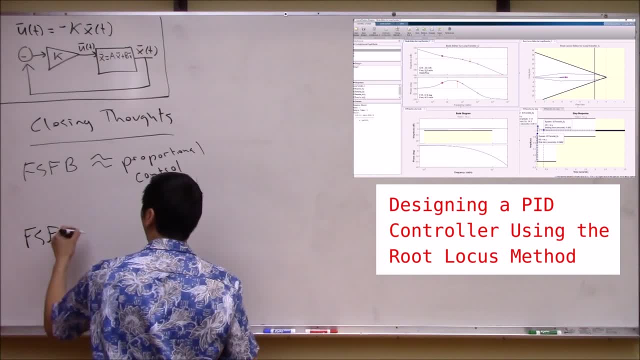 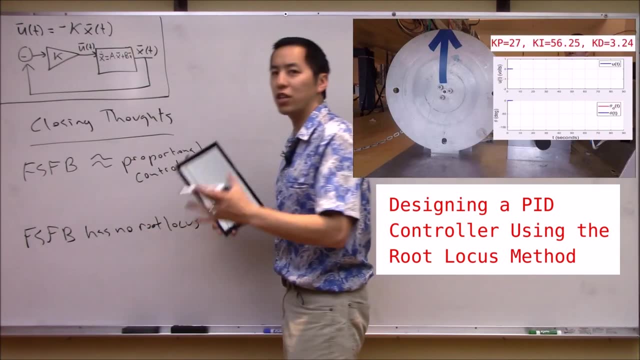 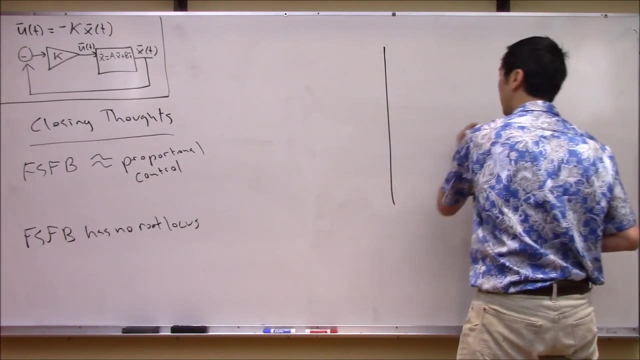 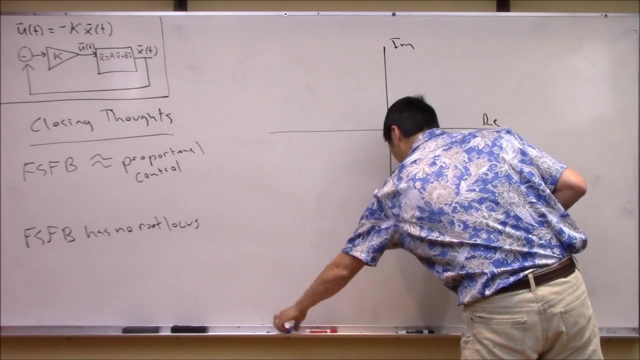 So full state feedback, you know, has no root locus, In the sense that you are no longer constrained to move the closed-loop pole along given locus lines, right? So if you plot out, you know your real imaginary axis and let's say, your open loop system had poles. I'll draw them in blue here, right? 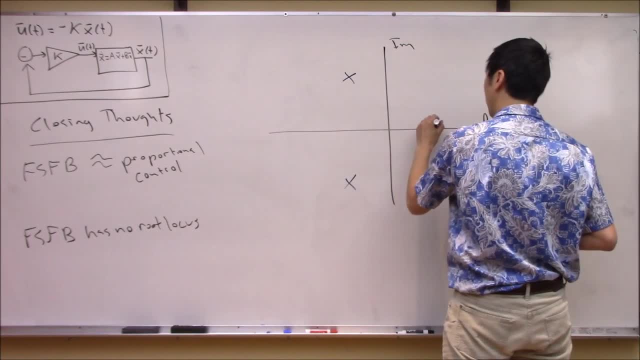 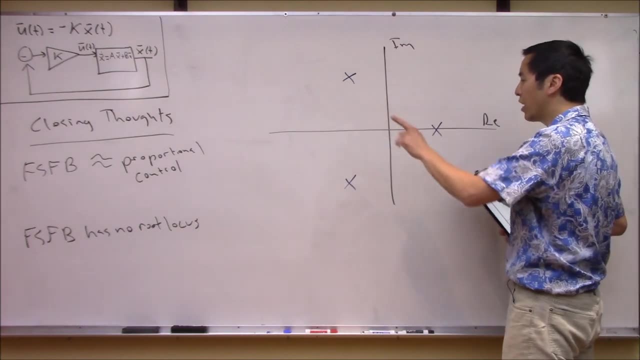 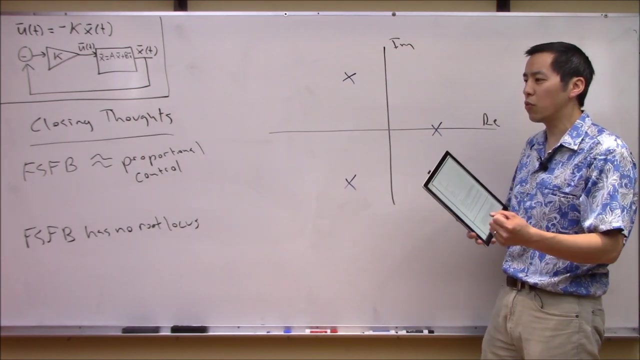 Had poles here, here, here, you know. it had dynamics that looked like this: right And with root locus, right locus. we saw that by adding a controller, these poles would move in specific lines or specific locations, and and half the half of your time was just wrestling with making sure that we placed. 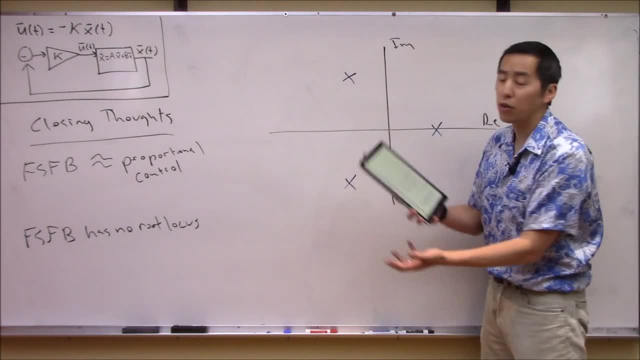 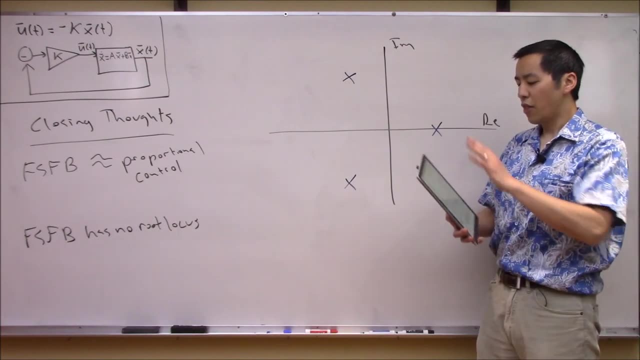 the controller poles and zeros in locations that would drag the locus lines to where we want, and we spent an incredible amount of time just fighting with the system. but with full state feedback control, there's no idea. uh, there's no lines here, right, you can move them anywhere you want, right. 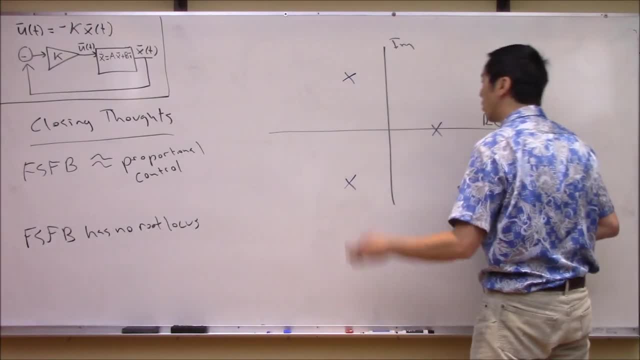 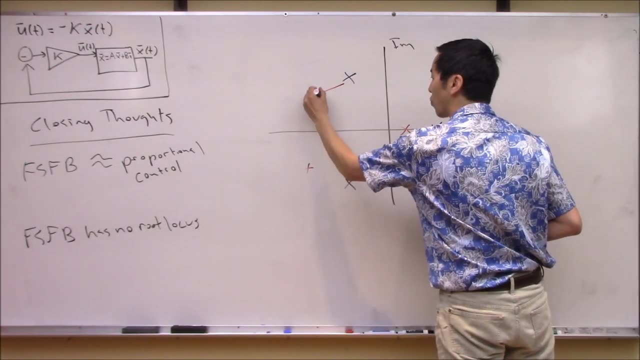 so if you don't like these locations and you want the poles to go somewhere else, like, uh, you know here, here and here, right, you don't have to drag them along lines, you can directly move them with full state feedback, right, full state feedback just will will move them. whabam, right there, okay. 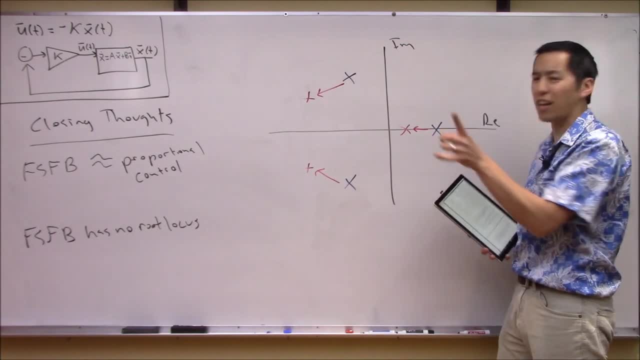 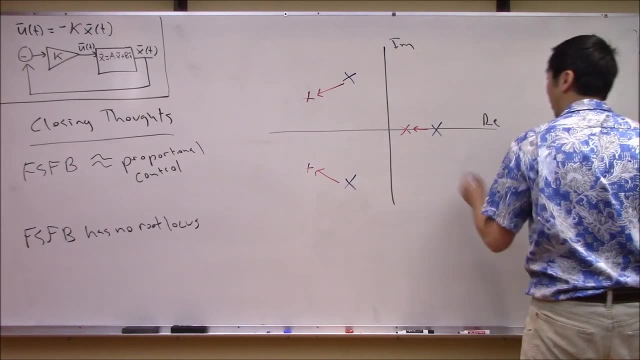 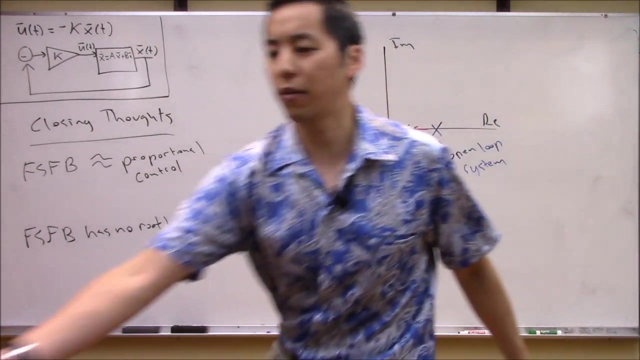 and, and if you think about this like, this has huge ramifications, right? for example, consider what if? what if these blue poles were like your open loop system here? so, like we said, this is open loop system, this is your natural system, right? so again, i i'm, i'm in aerospace, so i like to think of of. 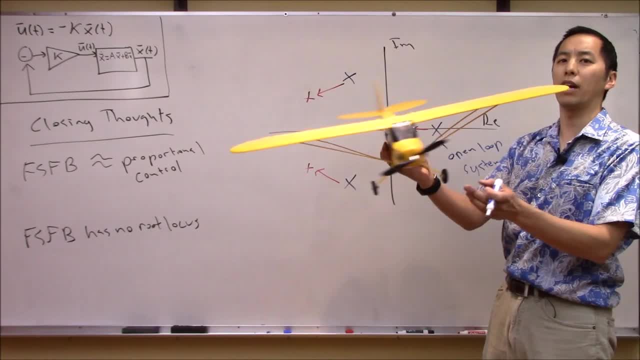 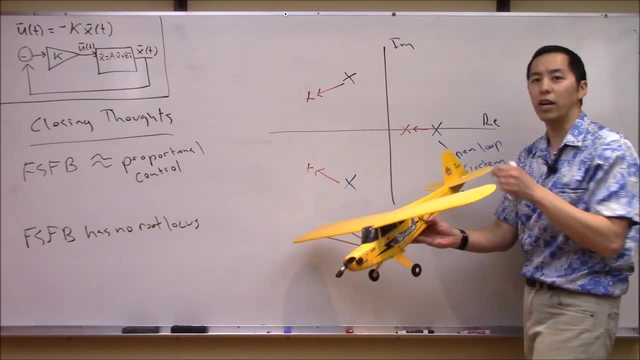 aircraft examples. let's say: you've got this slow piper cub right. this is a low performance aircraft and it it has open loop poles like like this, like these, these blue x's right. well, if i slap a full state feedback controller on this, i can move it to anywhere. like what? if what you know here, let's. 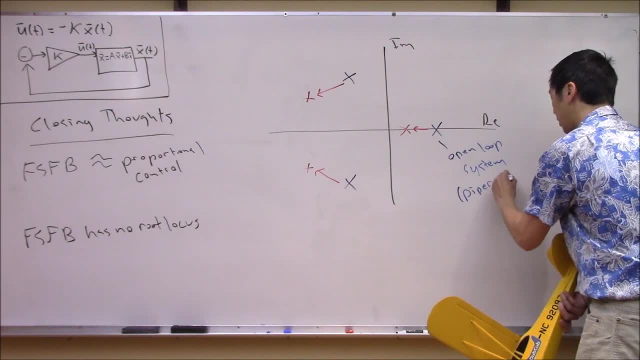 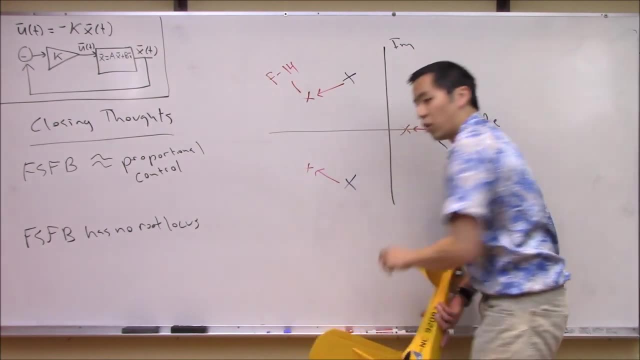 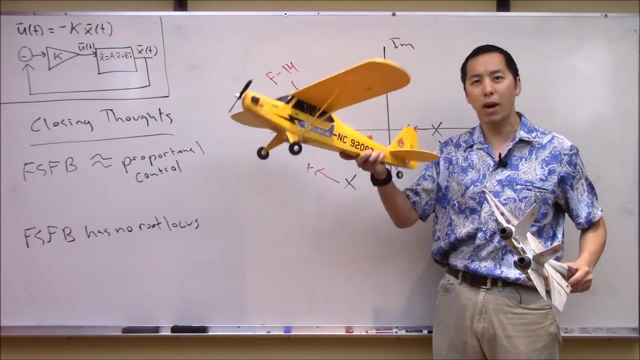 let's call this a piper cub, right? what if these are like f14 dynamics? right, so i don't want this. i want it to look more like an f14 right, so i can get rid of this. full state feedback can make my piper cub behave like an f14 right, so now it. 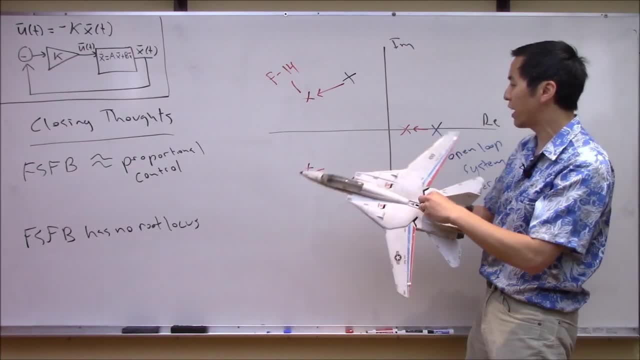 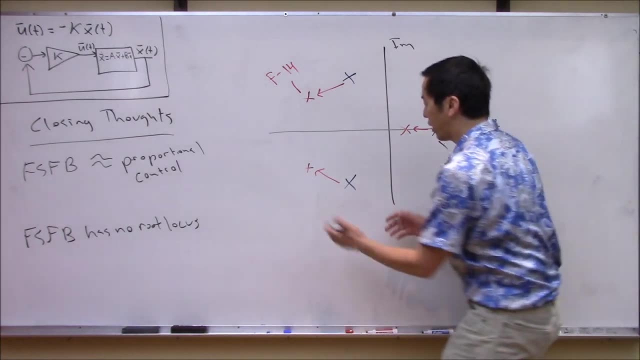 can fly around, it can be doing mach 1, it can be turning and burning, doing all this kind of cool stuff, and it doesn't stop there, right, there's nothing to stop it. let's say, let's say you've got other aircraft like you, you, you want this thing to behave, and yet another. 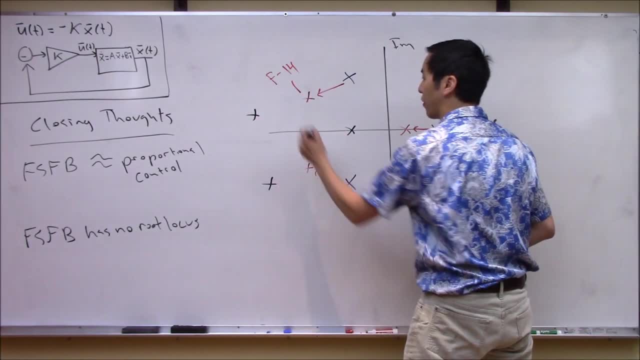 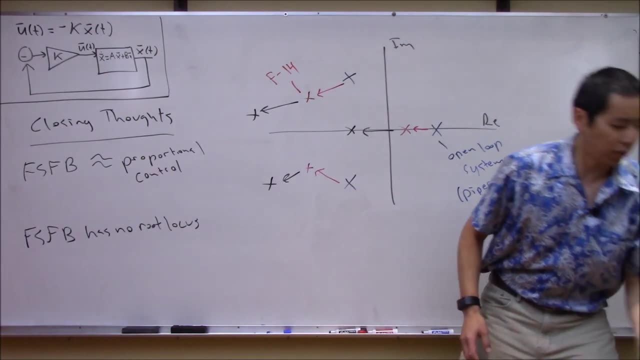 maybe you want it even faster. you want all the poles even further to the left, right. you can move it here to here to here, right. you want it to now behave like some forward swept- you know other ridiculous fighter jets. so i can now turn my piper cubber into my f14, then i can turn it into. 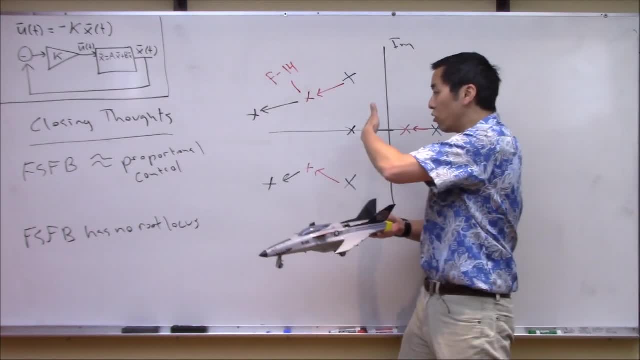 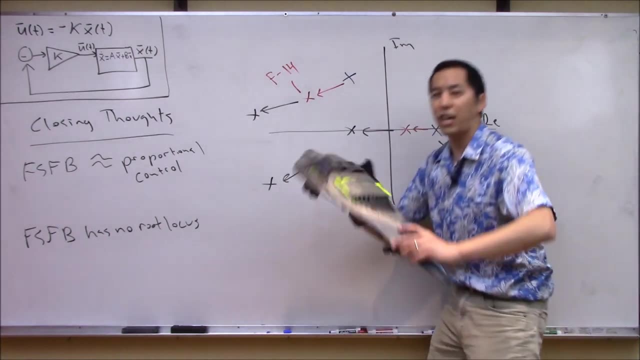 into something faster, or you can even. there's no limit to this, right, you can keep going. you can turn this if you don't like this and you want your experimental, crazy prototype hypersonic vehicle that can fly around and, and and- do it like this. you can do it like this. you can do it like this: 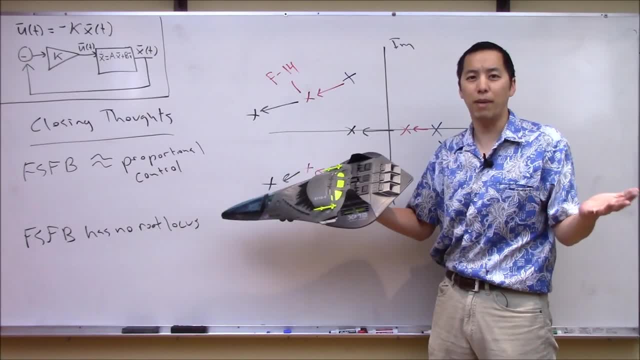 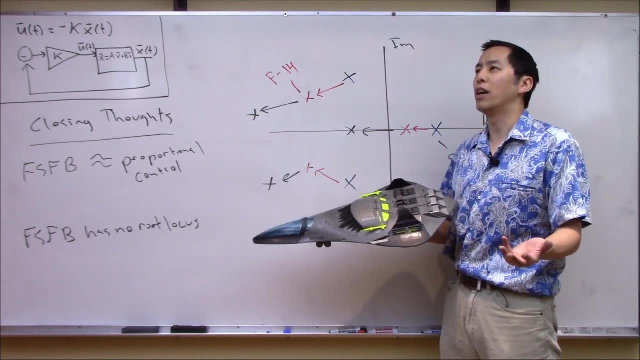 you can do everything. that nothing is stopping you with full state feedback control, right, full state feedback control says you can go anywhere you want, right, you can be gosh. it sounds so, uh, you know my daughter's in kindergarten. it sounds like one of those things they tell you in. 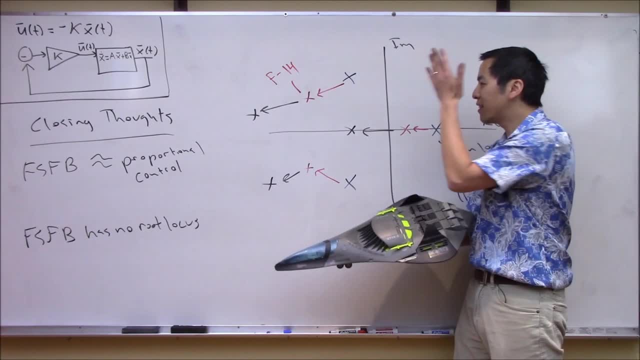 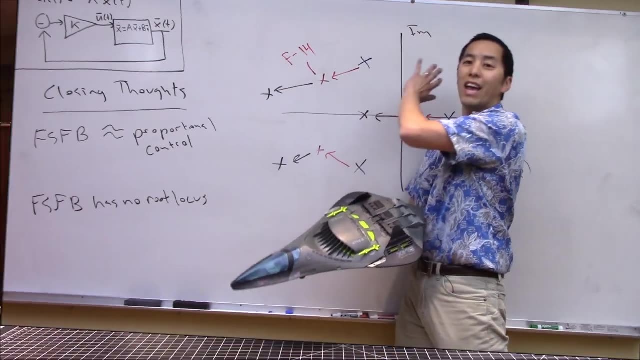 kindergarten. right, you can be anything you want to be right. that's exactly what full state feedback control is telling you. it says: you can be anything you want. i can change the dynamics in my system. i can put the eigenvalues anywhere. so in summary, in this short lecture we saw how full state feedback 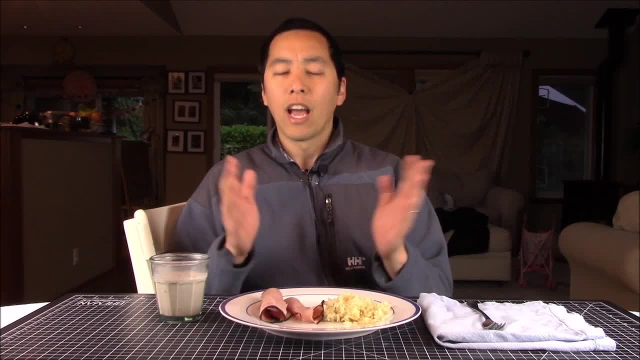 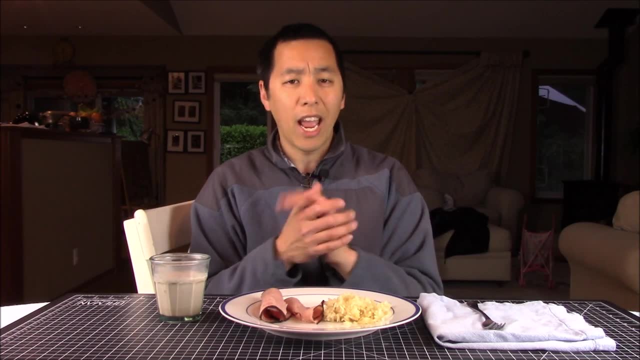 is an incredibly simple yet incredibly powerful control architecture. as long as your system is linear and controllable, full state feedback is going to allow you to move the closed loop eigenvalues- your system- to pretty much anywhere you want, so what this means is you can make any system behave. 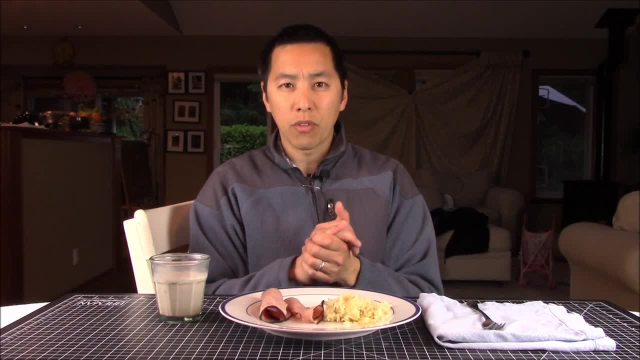 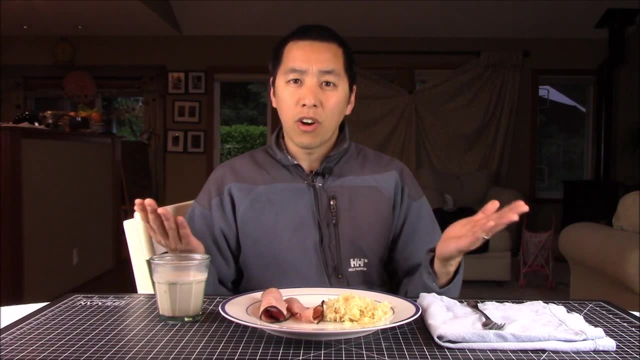 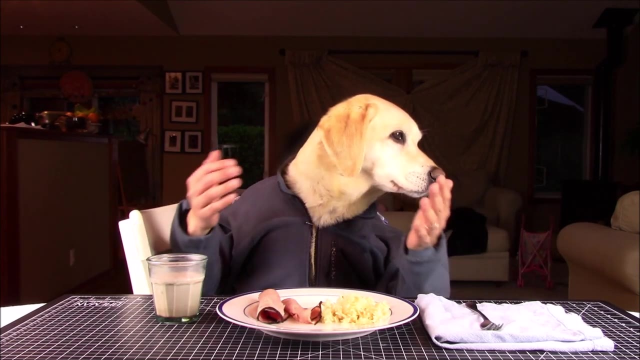 like any other system, as long as they have the same number of eigenvalues, so you can literally transform your system to be whatever you want. so if i wanted to act like a human with a dog's head on top, full state feedback would make this possible. now, obviously, this is a little ridiculous. so you have to ask yourself: where does full state 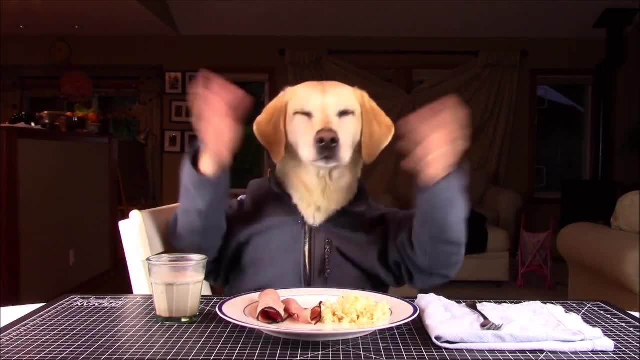 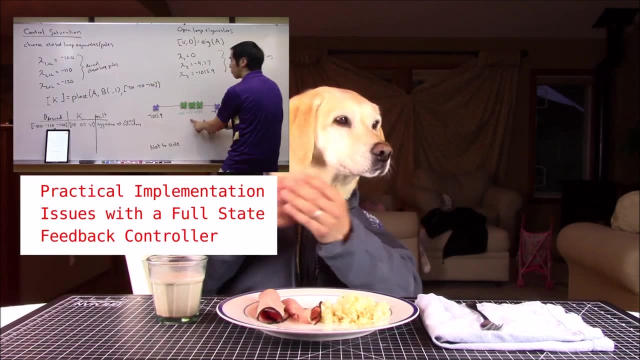 feedback break down. i mean, if full state feedback is so great, why doesn't everyone use it? well, i'm glad you asked that question because in our very next video we're going to take a look at some practical implementation issues that you're going to encounter with full state feedback. so with that, 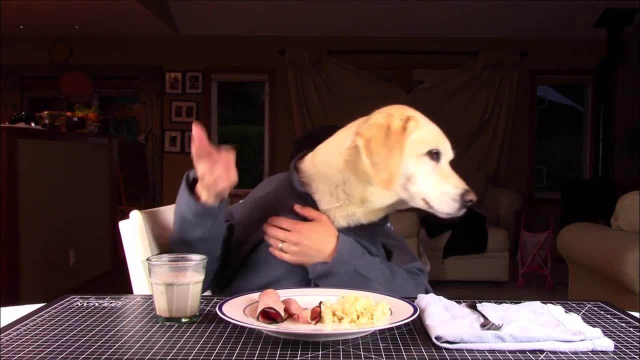 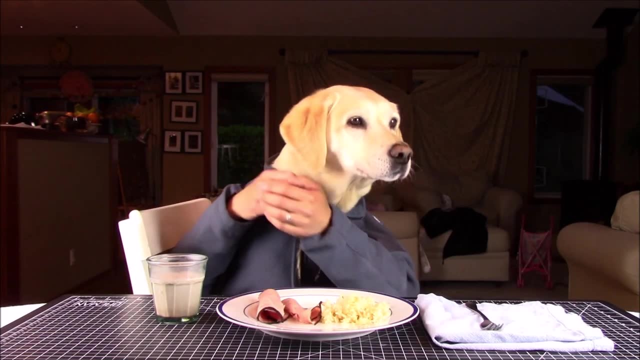 being said, i hope you enjoyed the discussion today and, if you're already a subscriber, thanks for sticking with with us. if you're new to the channel, please consider subscribing, as we'll have lots of great controls engineerings in the future and i hope you'll join us at a future video. now i don't 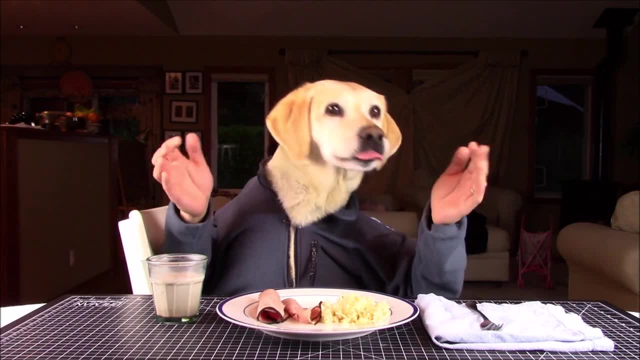 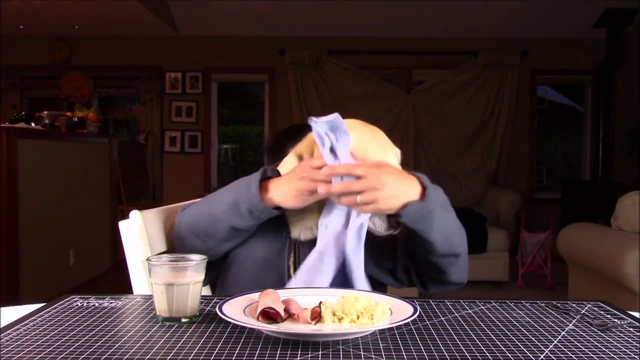 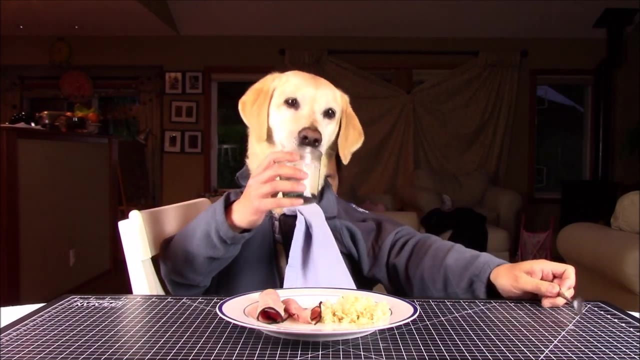 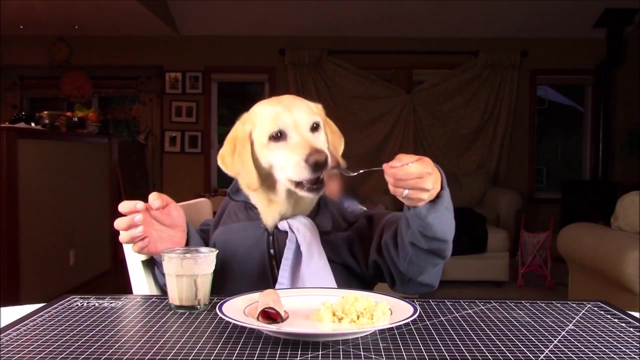 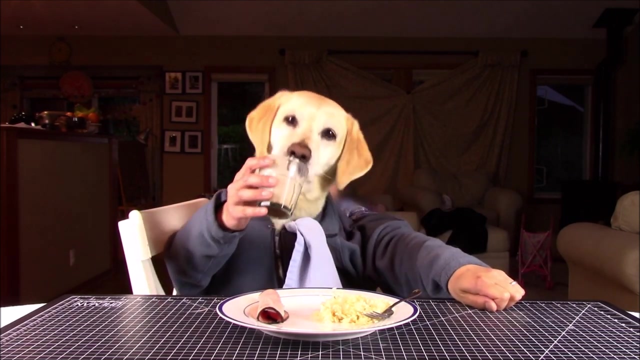 know about you, but i'm pretty hungry after all this talking, so i'm going to grab a bite to eat until our next time. i hope to see you later, talk to you later. bye, so you.